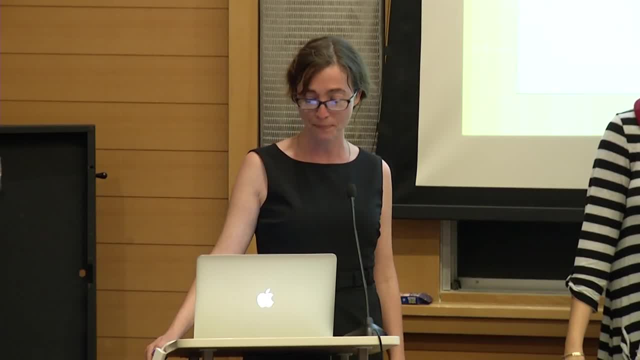 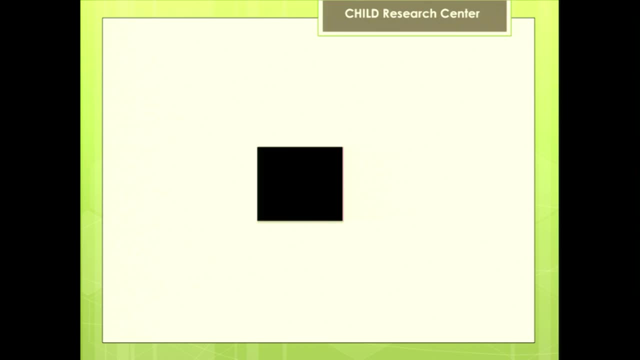 Alison Briscoe-Smith, who's one of our co-directors that I'll introduce in just a moment. So let's start out by thinking about a black box. Some of you have been sitting in the room staring at this black box, wondering what that is about, And essentially we can think about what the public 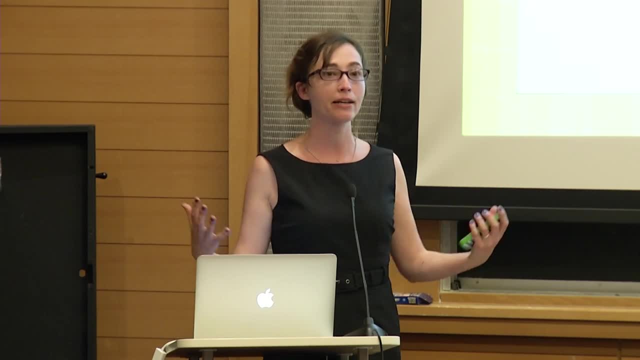 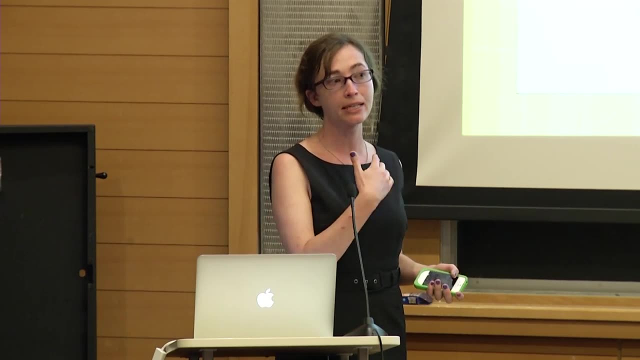 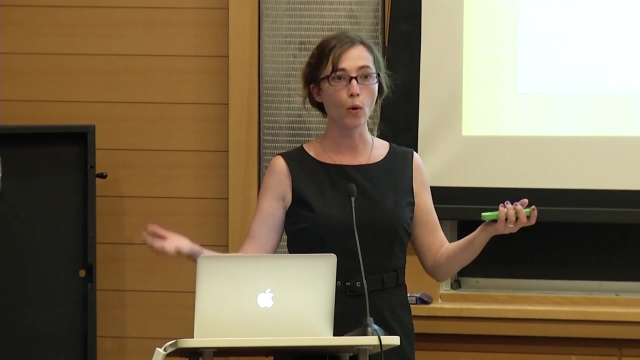 or what we, even as scientists, know about what's going on in a child's development that leads to better or worse outcomes- outcomes of any kind: health outcomes, successful school matriculation, career, et cetera. And what do we know about what causes these outcomes? Well, we think about genes. 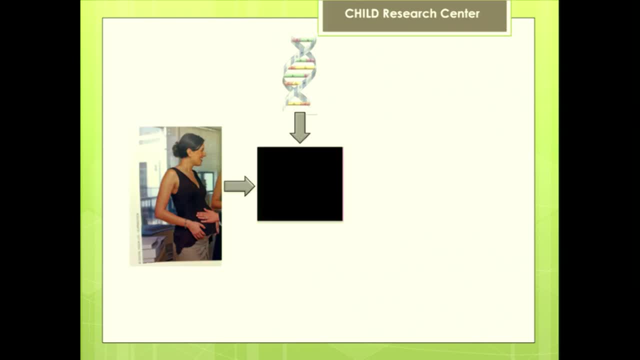 Genes go into this black box. We think about prenatal exposure to different toxins, as Dr Eskenazi is going to talk about today, or to substances of abuse. We think about toxic stress, the home environment, the school environment, the parental unit, And then we think that there's some. 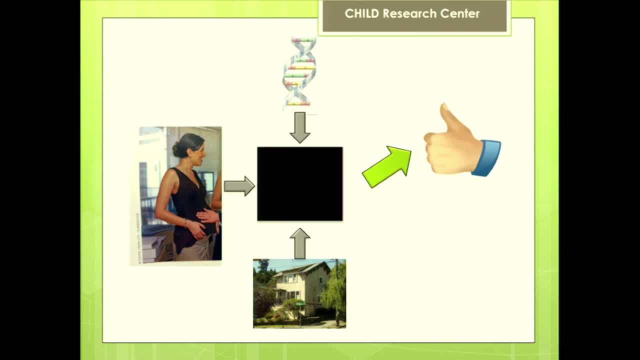 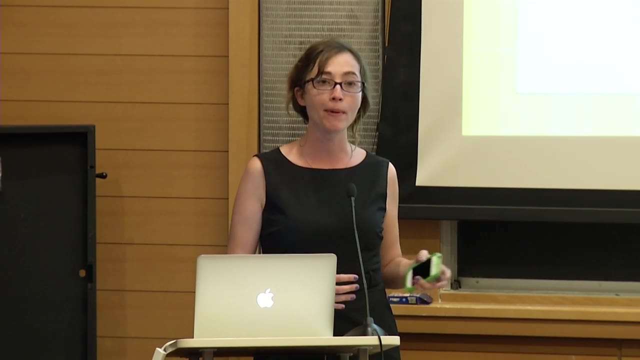 kind of black box algorithm that then determines whether the child's going to have a good outcome- health-wise, education-wise, career-wise- or a bad one, And the goal of this research center is to try to figure out how to move beyond this. Let's learn a little bit more about the mechanisms that are at play. 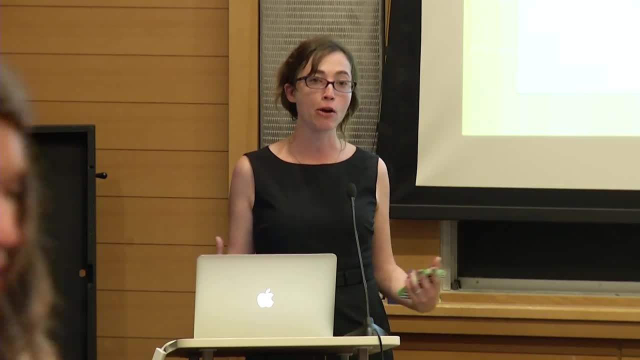 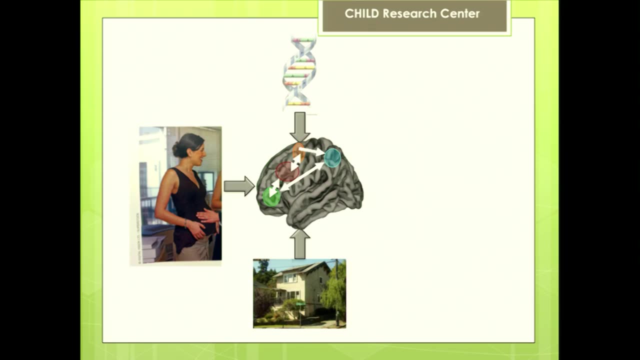 here that all interact- the genetic and biological and environmental and societal mechanisms that are all at play, And so for this we really need to take a closer look at where all of these factors are interacting, and that's in the brain right, And so we've got specific brain networks that are 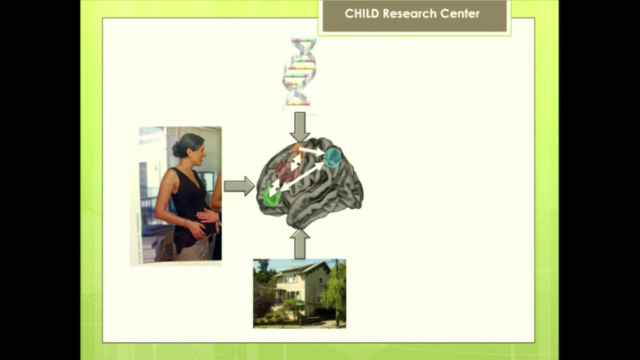 developed and we've got specific brain networks that are developed and we've got specific brain networks that are developing during childhood and adolescence. Some develop before others. They're modulated by gene expression, by environmental factors, And we want to figure out what's going on. 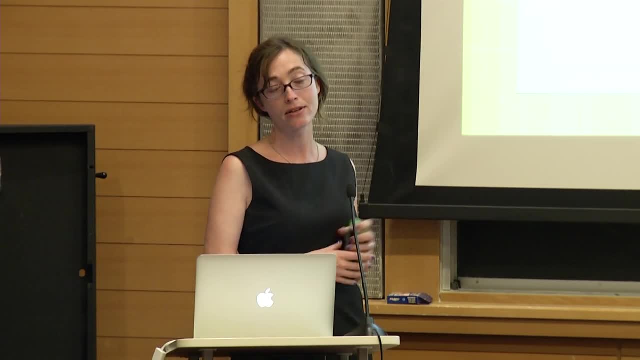 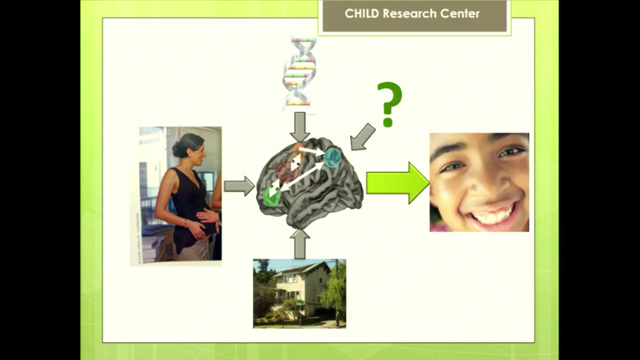 that's disrupting or that's enhancing the growth of these networks? When might one network be able to take over from another if another one's been damaged in some way, And what are the kinds of interventions that we can build, knowing what we know about the developing brain, so that we can try to? 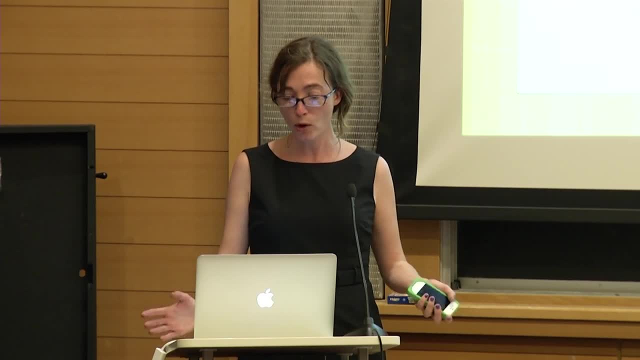 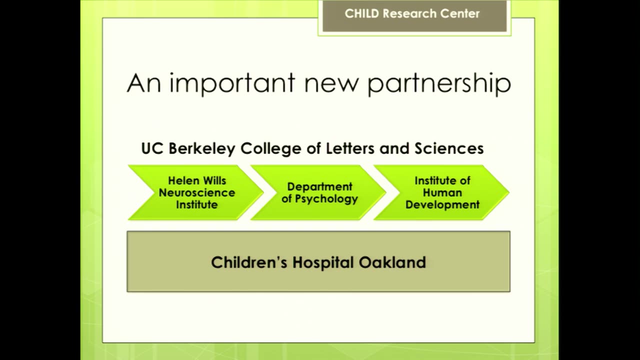 ensure that we're able to take over from another if another one's been damaged in some way. So this is an important new partnership. This is straight collaboration between UC Berkeley and Children's Hospital Oakland, And so it's supported. We've gotten seed funding from all of these. 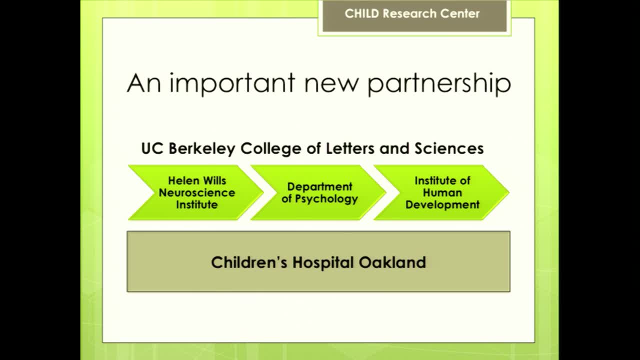 institutions, so thank you to all of them. We're going to need other support to keep it going, though, But from the College of Letters and Sciences- and here I've ordered the three institutions within UC Berkeley, from neurons to neighborhoods, essentially just picking up on an. 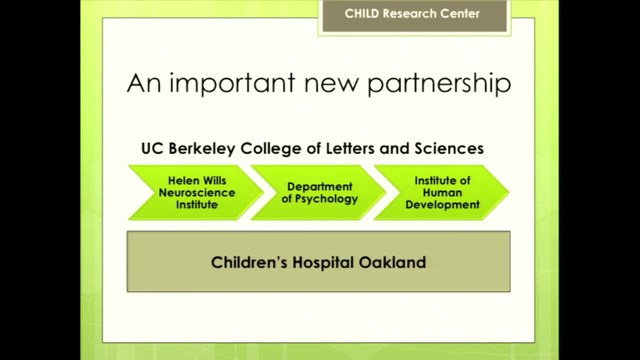 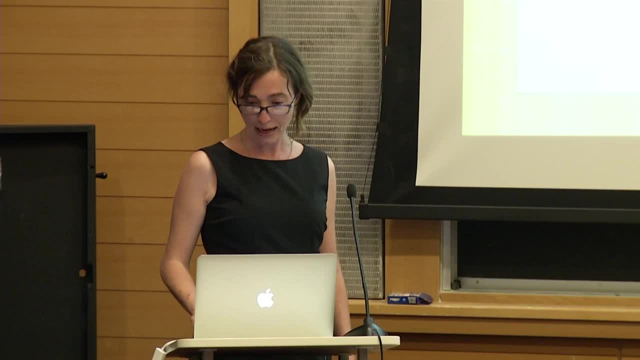 old term from a national network. So from neuroscience, individual cells and cellular interactions all the way up to how humans interact with their families and society. Okay, So our mission is threefold right now. We're brand new, This is our first public event, And so 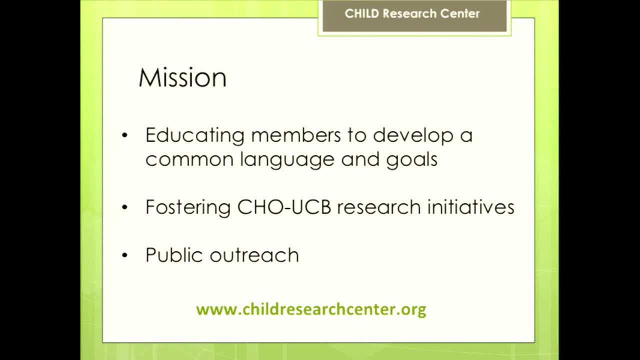 the first one is really to figure out who are the members, who are all the people at UC Berkeley and at Children's Hospital Oakland that care about this joint mission of trying to do the right science, to figure out how to get the right help to the right people. And so we're going to need 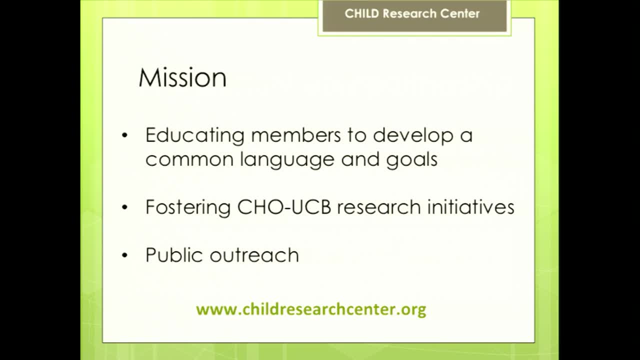 a lot of people, And so to be able to do that, we've got clinicians and scientists and staff that all need to be able to talk a common language right, So we need to be able to go to each other's talks. So we have a website now to be able to make announcements about these sorts of things And the 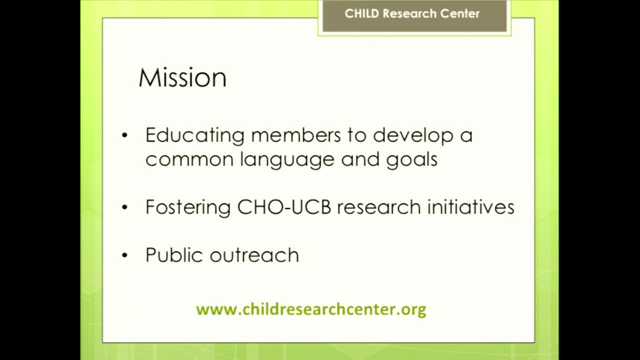 website is also. the newsletters are also available to folks from outside this community who want to join in. Secondly, we want to find ways to support from the ground up research collaborations that are going to involve children at the Research Institute- sorry, at the Children's Hospital Oakland. 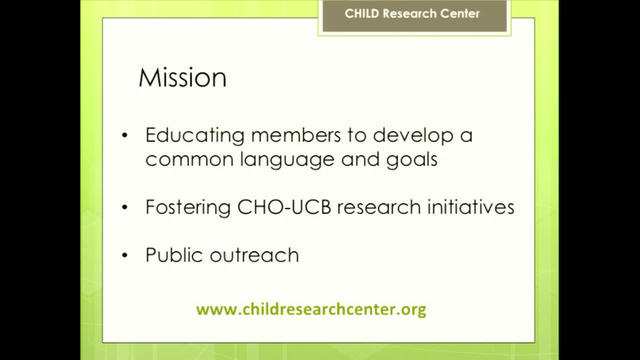 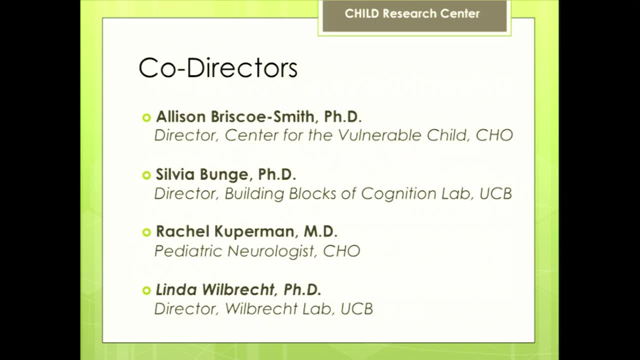 and working with scientists at UC Berkeley. And third is this public outreach. So the co-directors- the first one is Dr Allison Briscoe-Smith, who got her PhD at UC Berkeley And she now directs the Center for the Vulnerable Child And the others. we have a pediatric neurologist as well as a 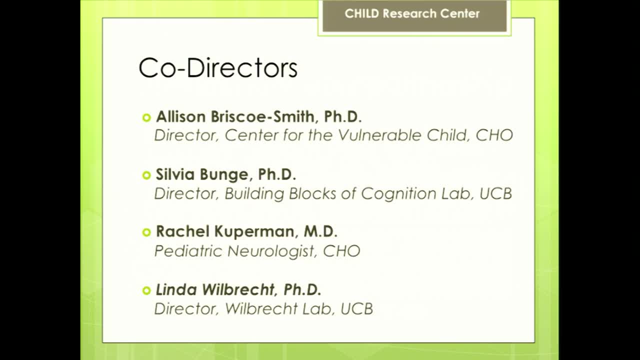 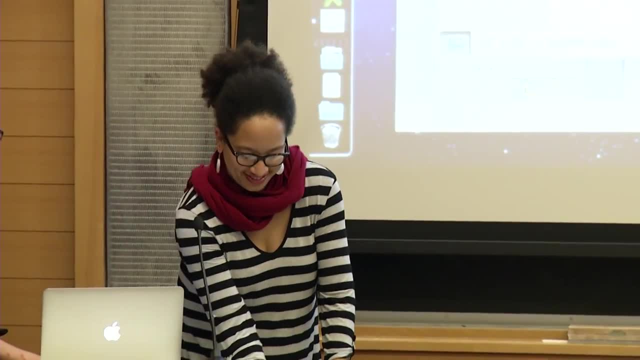 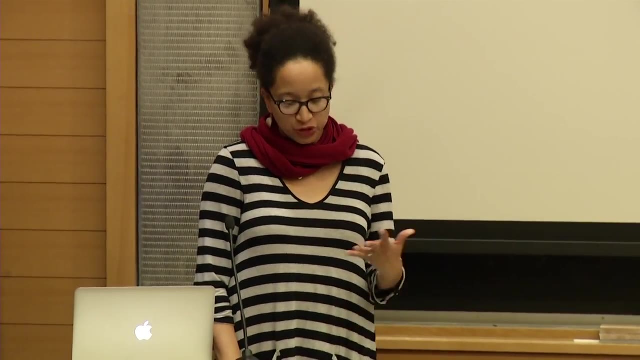 neuroscientist, who's a systems neuroscientist, who will be joining us soon at UC Berkeley. So, without further ado, Thank you, And thank you all for coming. We're again very excited to be launching our lectures in this way, So it's my 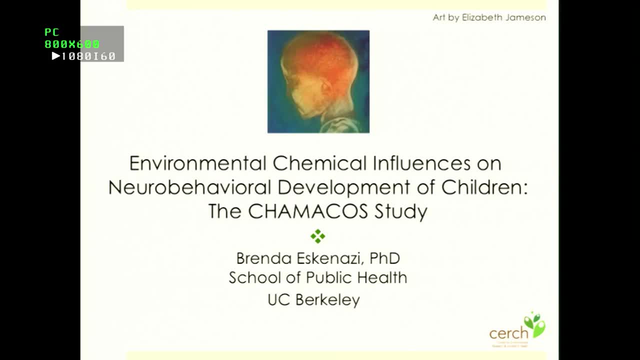 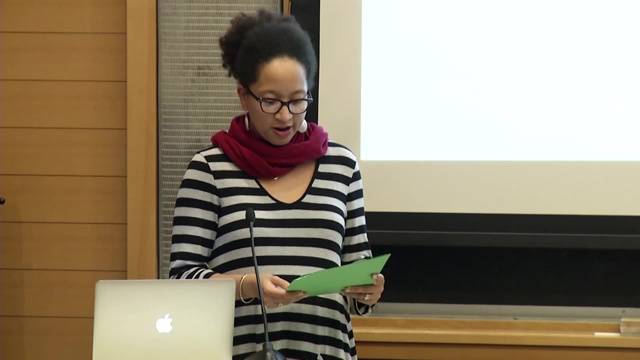 pleasure to go ahead and introduce Dr Eskenazi. She is the Jennifer and Brian Maxwell Professor of Maternal and Child Health and Epidemiology at the UC here And the principal investigator of the direct and the director of the NIEHS EPA Center for Environmental Research and Children's Health. She's a neuropsychologist and an 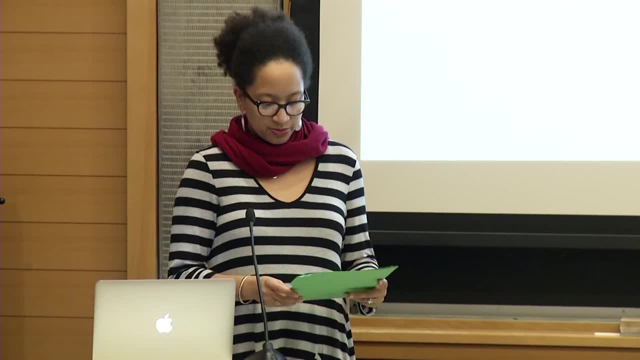 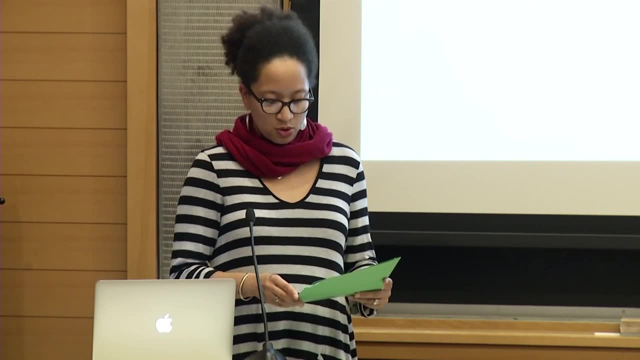 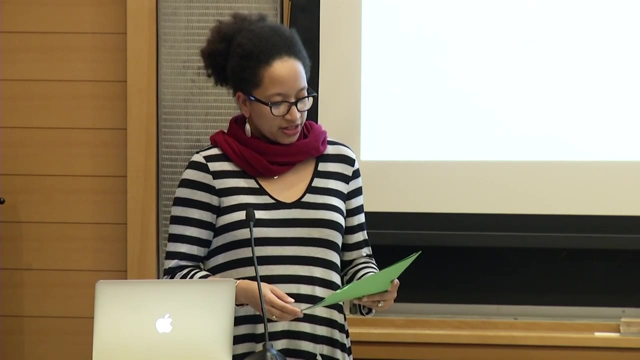 epidemiologist who has longstanding research interest in terms of the side effects and the impacts of toxins, including lead solvents, environmental tobacco smoke, pesticides, on human reproduction, both male and female, and also child development, And she's the director of CHAMACOS. Did I say that right? Close CHAMACOS And the 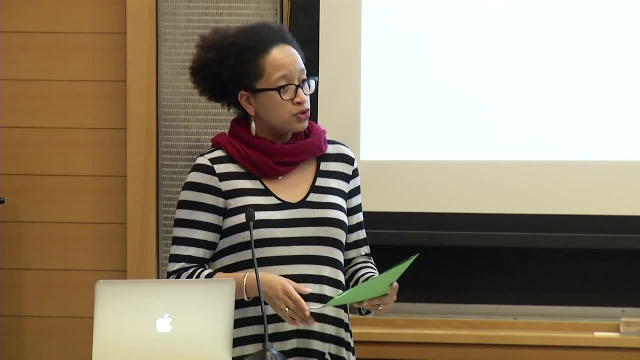 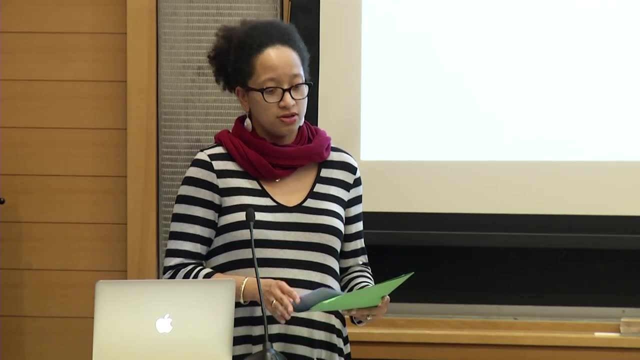 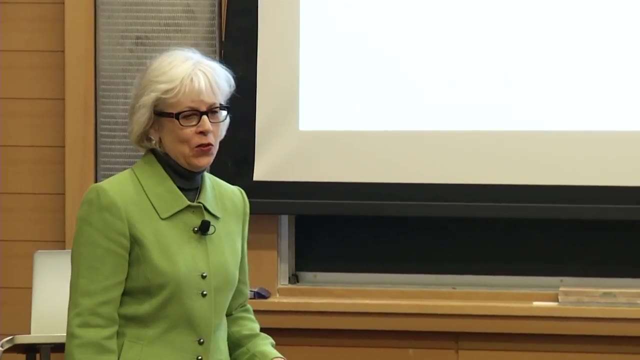 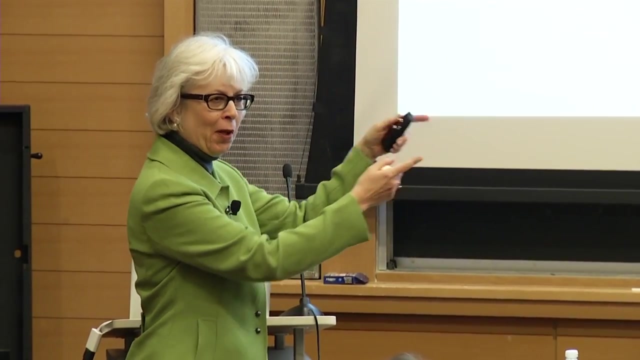 project that she's going to be talking about tonight. This is a longitudinal birth study examining chemicals and other factors In the environment And, again, the impact on children's health. So welcome, Thank you. So the first thing I'd like to say is: Sylvia, in your slide I'd like there to be another arrow that says School of Public. 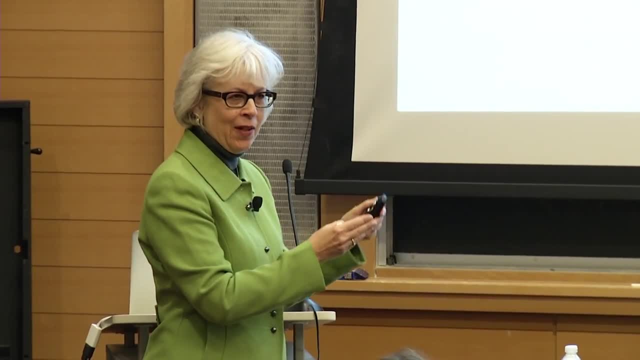 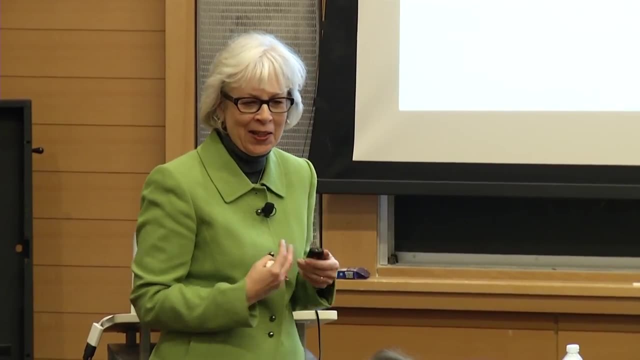 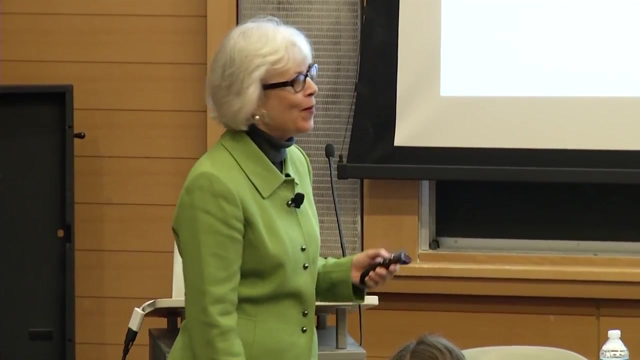 Health, because we should be going all the way up to not just neighborhoods but large communities and whole societies, And I think that's exactly exactly what, Exactly what public health does, Except nobody invests in public health. Anyway, today I'm going to talk about environmental 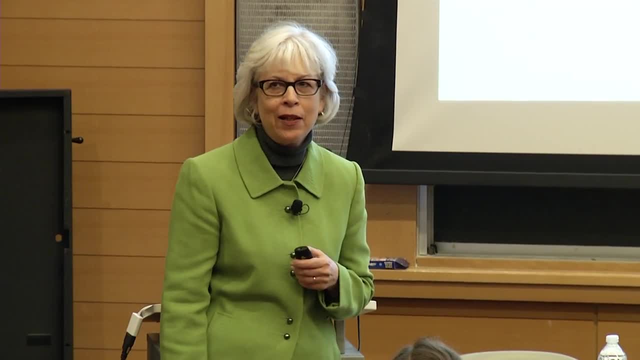 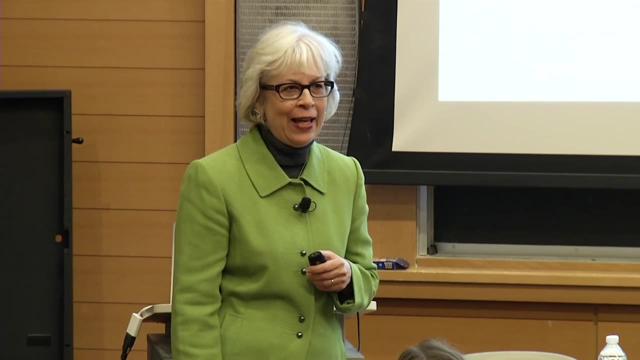 influences on neurobehavioral development. And let me just say as a disclaimer that I was trained as a neuropsychologist. I do have my PhD in neuropsychology And I gave up being a neuropsychologist after six months of practicing neuropsychology. So I do. 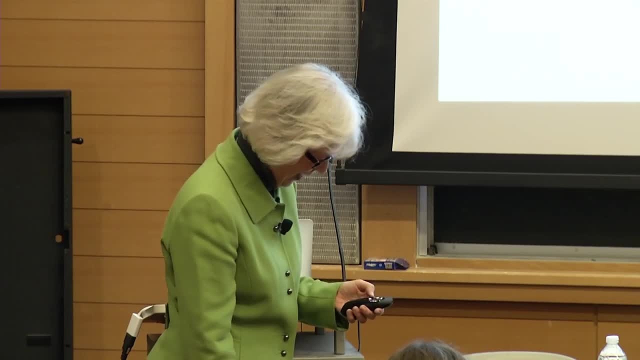 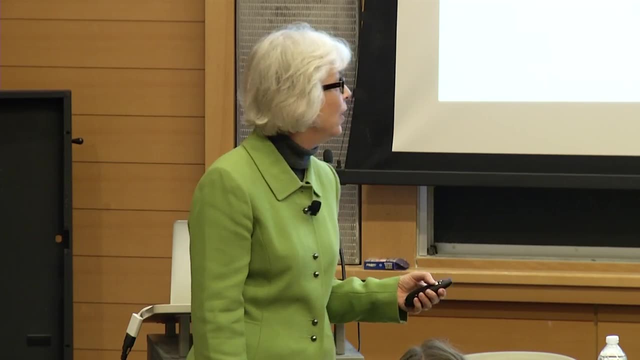 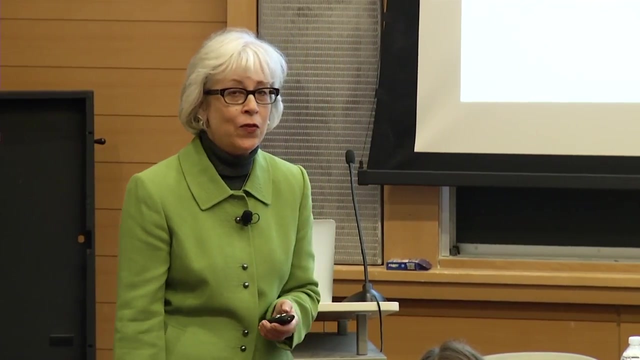 not claim to know anything, But I work very closely with Carolyn Johnson, or Kai Johnson, who is the neuropsychologist on our team. So Take you back about 30 years ago, when I started in this field- actually more than 35 years ago. 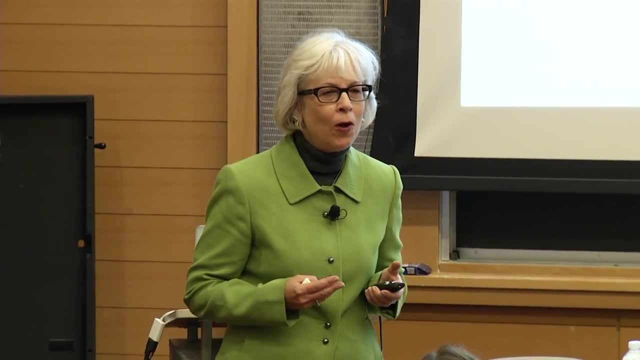 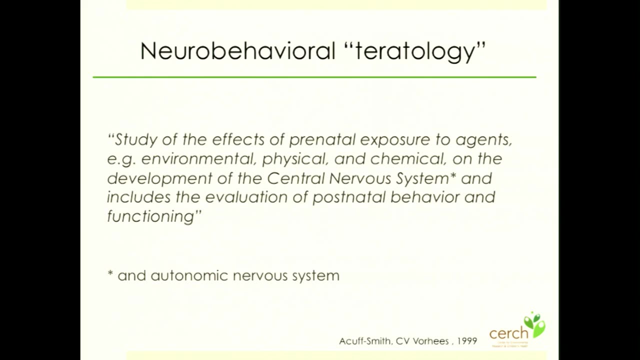 There was a field that was blossoming and we called it neurobehavioral teratology. Teratology because people were interested in chemicals and how they affected structures, anatomical changes in children causing birth defects. Neurobehavioral because people began to think, hey, maybe there are chemicals that can also affect neurobehavioral development. 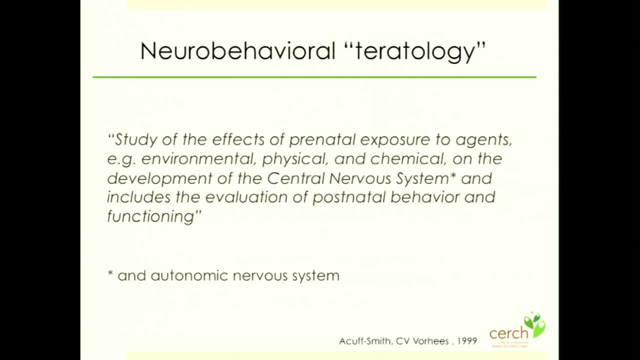 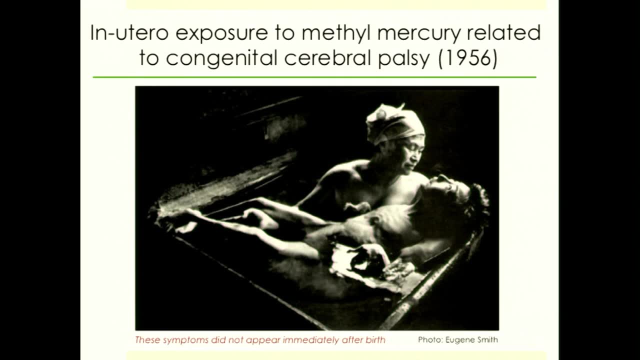 And so the field of neurobehavioral teratology began. It also began because a number of unfortunate events occurred. In 1956, mercury was spilled into Minamata Bay, Japan. Unfortunately, Japan has had its fair share of unfortunate events. 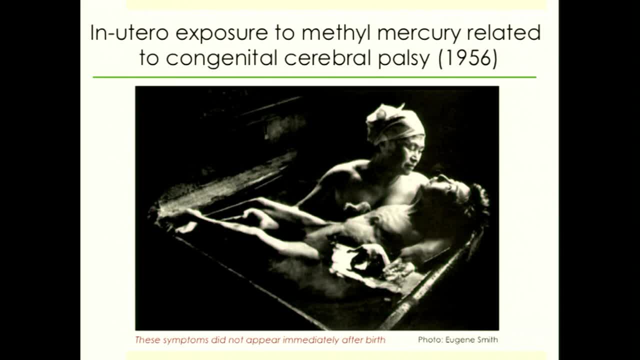 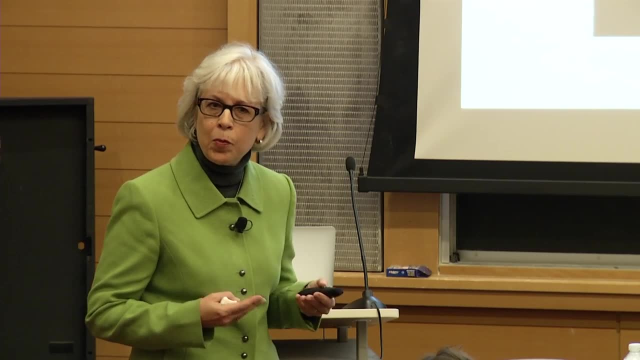 And this was one of the first In 1956, actually not the first, The first was Hiroshima. But in 1956, this mercury was spilled into the bay and it was methylated by the microorganisms in the bay. Children were born with cerebral palsy. 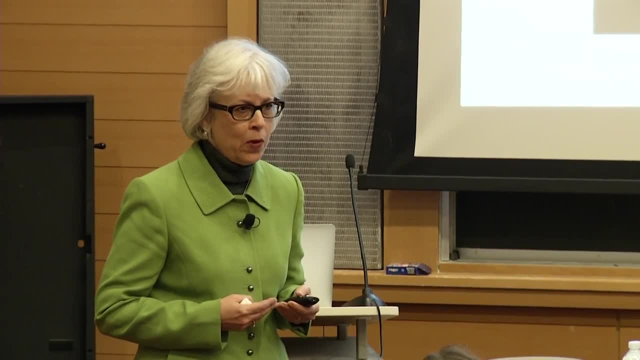 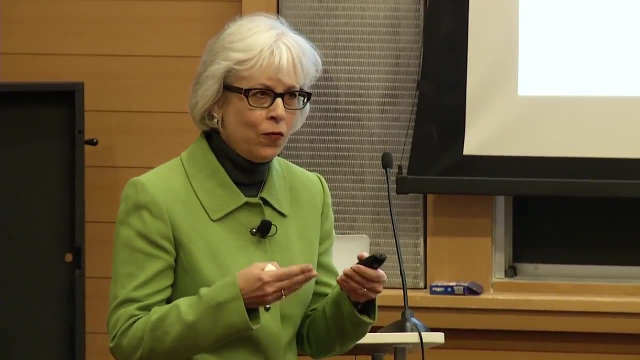 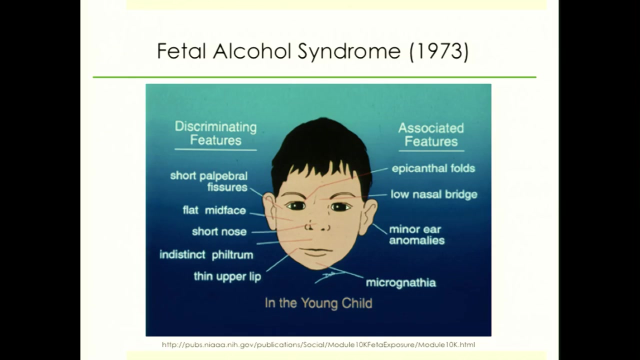 And they couldn't figure out what was causing that cerebral palsy. And so began the concern that chemicals in the environment could actually affect brain development. Taking you a few years further, in 1973, we identified for sure at this point, fetal alcohol syndrome. 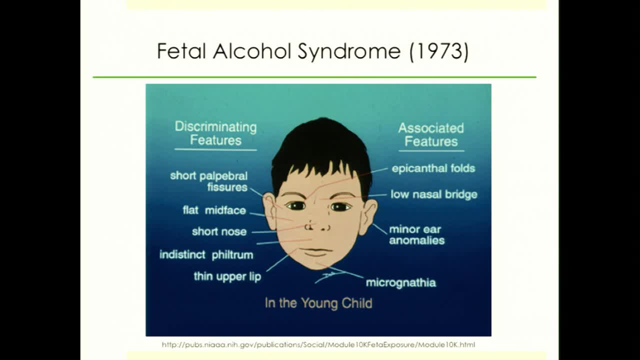 That high doses of alcohol consumption of the mother during pregnancy could cause behavioral and actual facial changes of the child that would result in cognitive deficits. But what they also found out is that when women consumed lower levels of alcohol, not as much as they did when they were born, they were more likely to suffer from cerebral palsy. 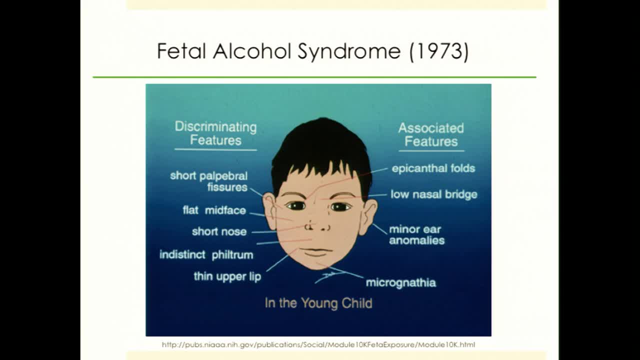 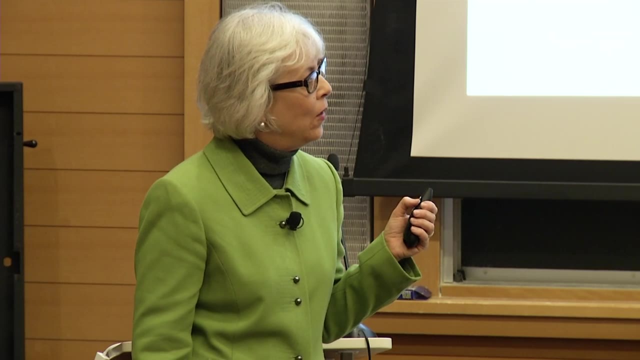 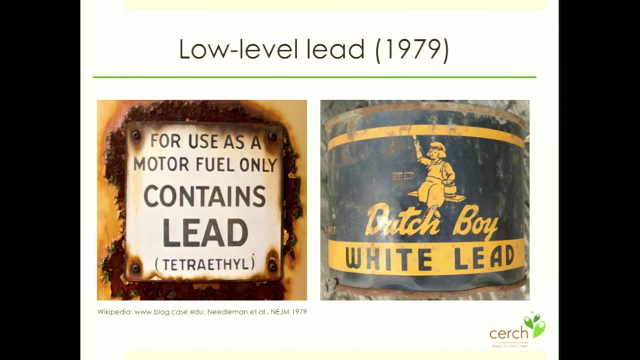 Not to the point where it caused fetal alcohol syndrome, That kids also may suffer from cognitive deficits. In fact, there was no clear threshold of when alcohol consumption was safe during pregnancy. Take you to 1979. During the first post-war years, people became very aware that high doses of lead 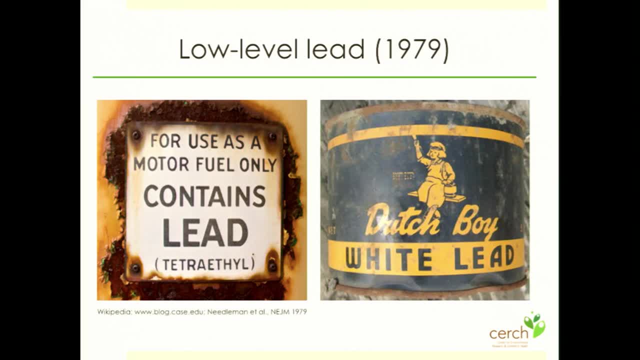 resulted in a high level of blood sugar, Resulting in a high level of blood sugar, Resulting in a high level of blood sugar, Resulting in cognitive deficits and also coma at very high doses. But in 1979, there was a very important paper that was published. 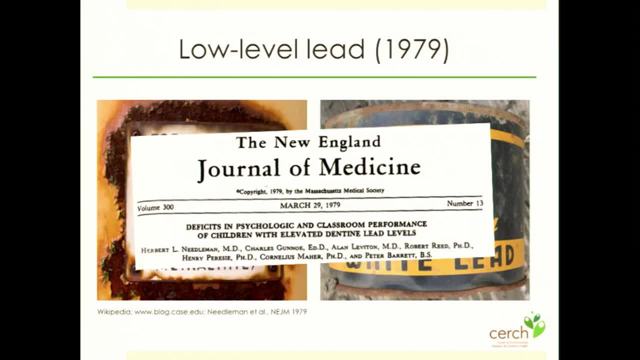 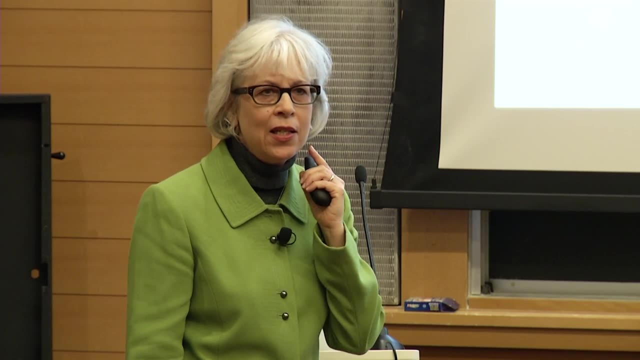 It was published by Herb Needleman in the New England Journal of Medicine, which is very unusual that the New England Journal of Medicine would publish an article on neurobehavioral outcomes in children. This study analyzed lead in teeth of children and I'm going to come back to teeth a little bit later on. 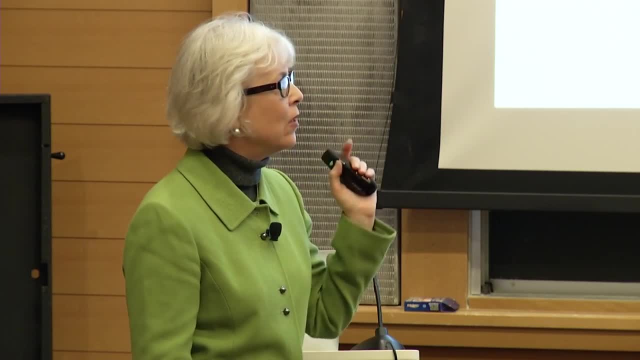 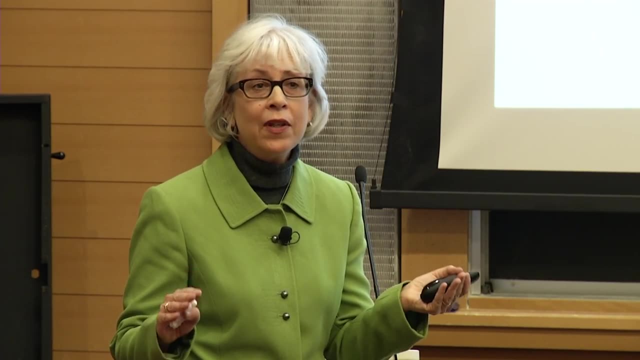 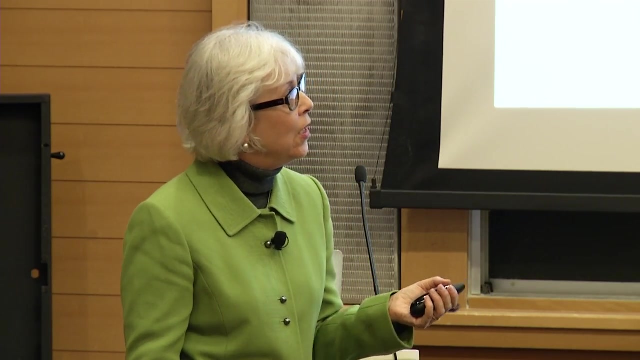 and found that there were psychological and classroom performance deficits associated with I wouldn't say low levels compared to today, but lower levels than they had suspected in the past as causing neurobehavioral deficits. So why were we concerned about these chemicals? Why were we concerned about these chemicals? 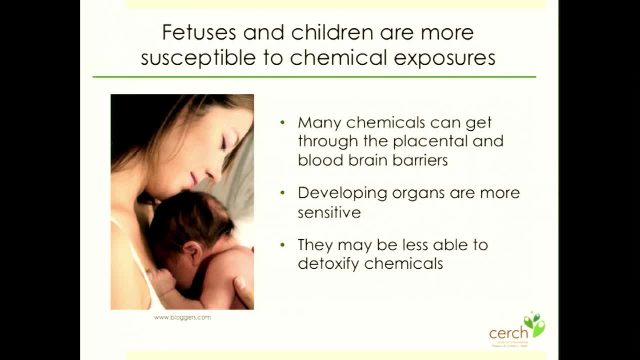 Because fetuses in children are more susceptible to chemical exposure. Initially people thought that nothing could get through the placenta and nothing could get through the blood-brain barrier, And then we found out that that's not true at all. These three cases that I just told you about are case in point. 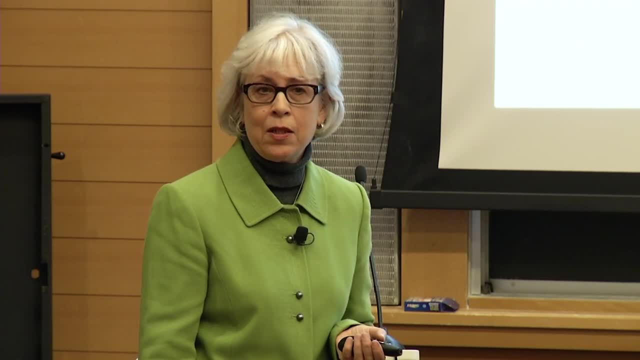 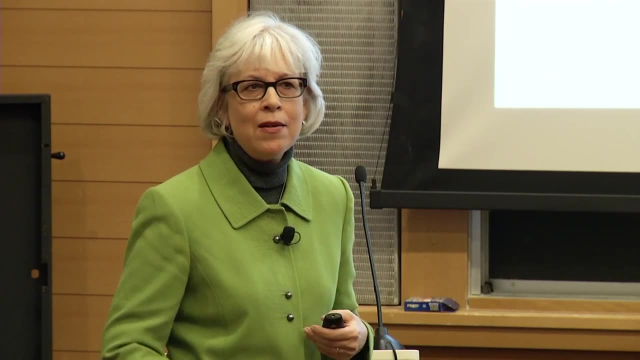 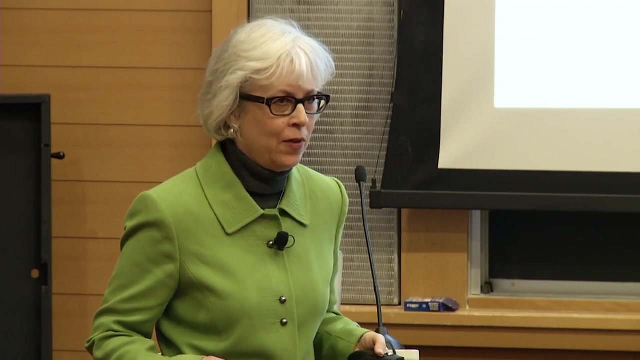 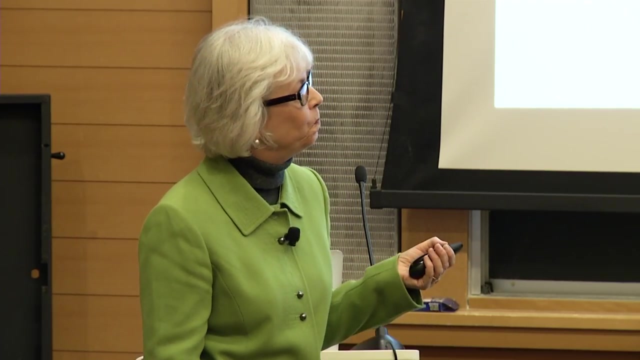 But we also found that developing organ systems were very sensitive, And not only that, but that fetuses in children may not have- they may not have- the adult mechanisms to make these chemicals less toxic in their body that adults have, So that it's only when we reach certain ages that we're able to detoxify chemicals. 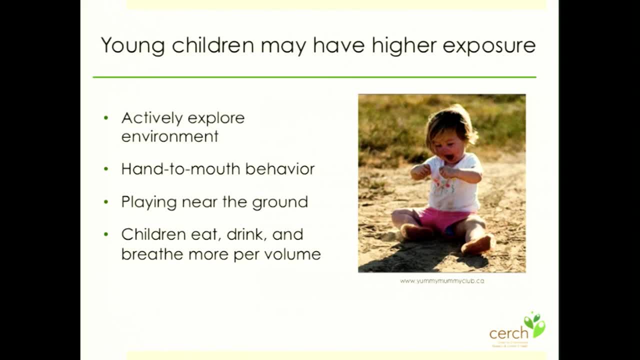 Not only are children more susceptible, but they also are not little adults in terms of how they interact with their environment. They actively explore their environment. They play with their hands in their mouth, so what's on the floor gets into their hands, what's on surfaces gets onto their hands, gets into the mouth and they ingest it. 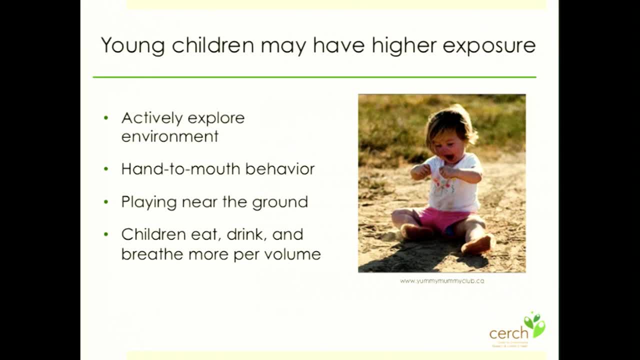 They also happen to play closer to the ground where many of these chemicals settle, And children eat, drink and breathe, per unit volume of their size, much more than adults do. Hence, not only are they more susceptible, but they actually get more exposure. 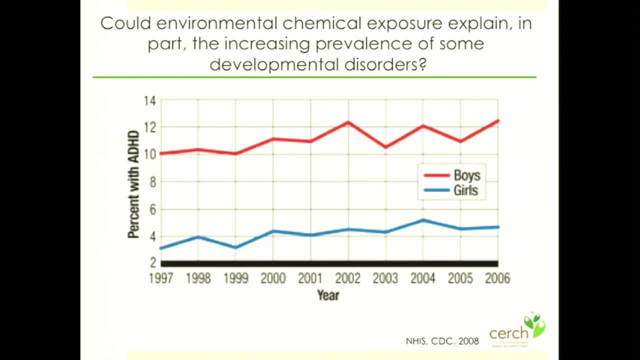 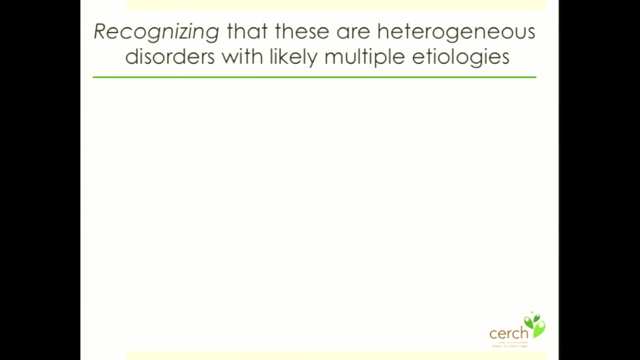 So how does developmental exposure explain, at least in part, the increasing prevalence of some developmental disorders that we've been hearing about lately, Whether it's an increase of learning disabilities, or childhood autism or ADHD? Clearly, we recognize that all of these disorders are heterogeneous, with likely multiple etiologies. 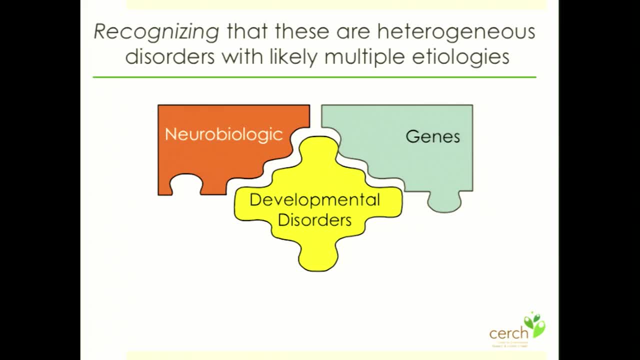 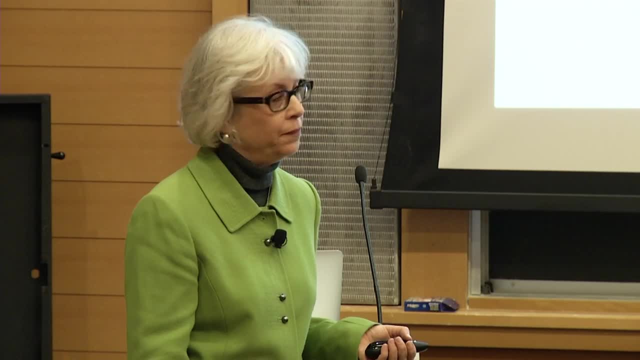 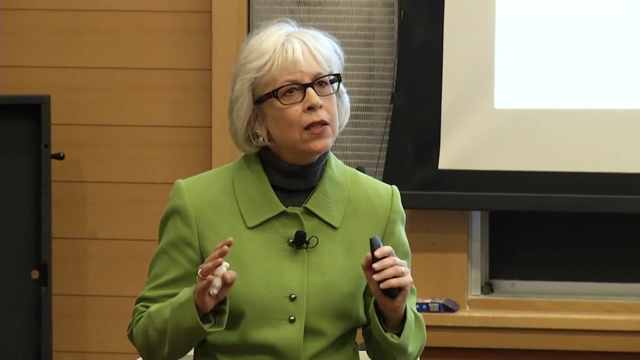 Whether they're neurobiologic or genetic or due to some kind of central nervous system insult or environmental. So I gave you a little bit of the history of neurobehavioral teratology, but for many years there wasn't much research on how children are specifically more vulnerable. 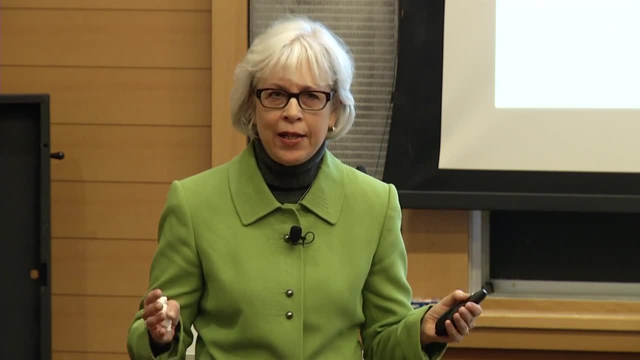 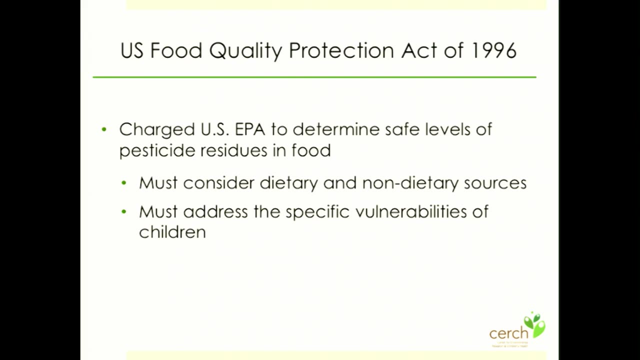 and susceptible to environmental chemicals. In 1996, there was a tide change. What happened in 1996 is the US Congress passed the Food and Drug Act, the Food Quality Protection Act. It charged the US Environmental Protection Agency to determine safe levels of pesticide residues in food. 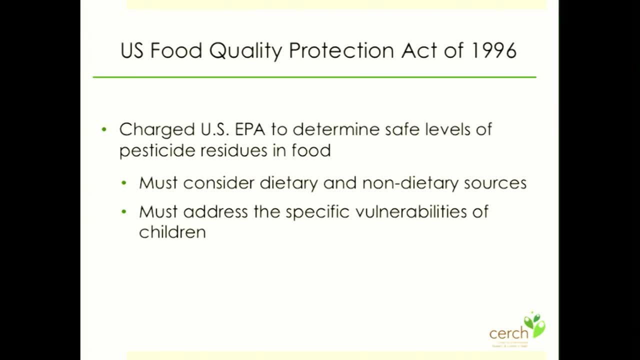 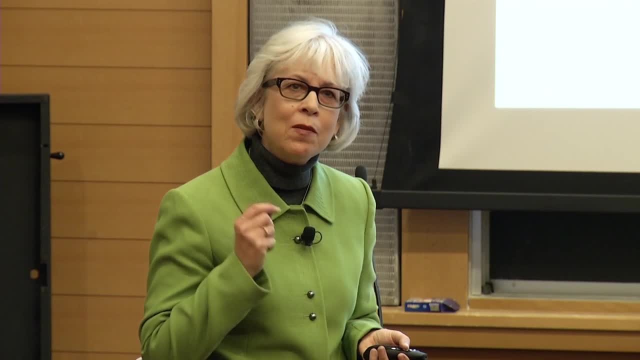 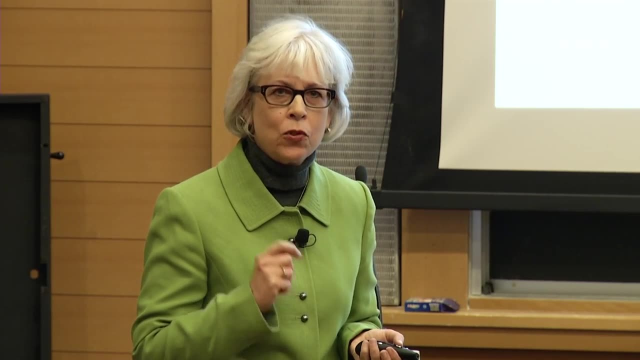 And it said not only to consider the dietary but also non-dietary exposures, like, for example, from living in the environment. But most importantly, it said in this Congressional Act that we must address the specific vulnerabilities of children to pesticides. That brings me to 1998.. 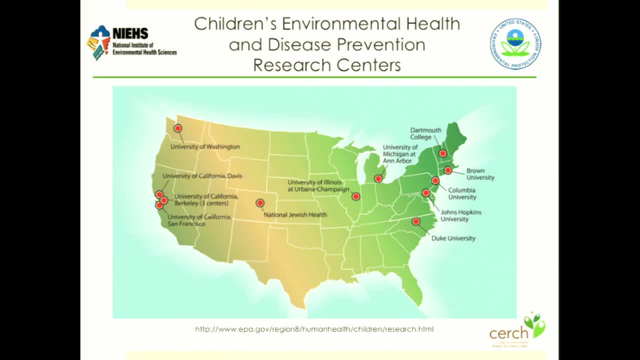 As a result of the Food Quality and Protection Act, the US EPA and the National Institutes of Environmental Health Sciences, which is part of NIH, jointly came together and they said: we need to fund research to inform the Food Quality Protection Act. We don't have enough information to regulate on these chemicals. 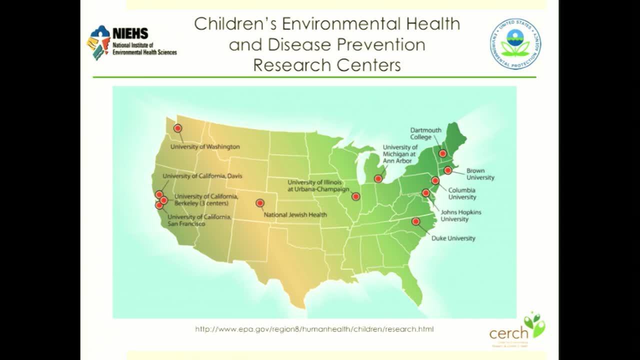 And so they set up different centers, including, over the next 15 years, three at UC Berkeley. We were the first, but there are now three at UC Berkeley And, if you notice, none of the other locations have multiple ones. We're very special. 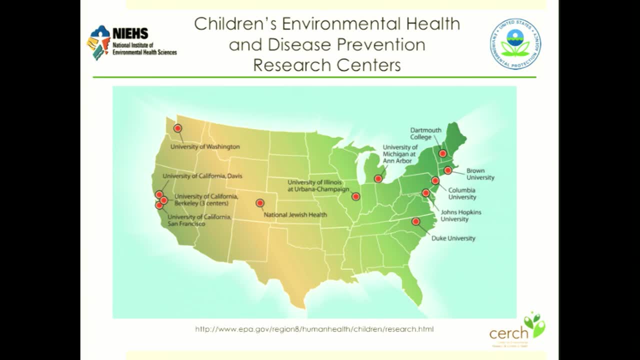 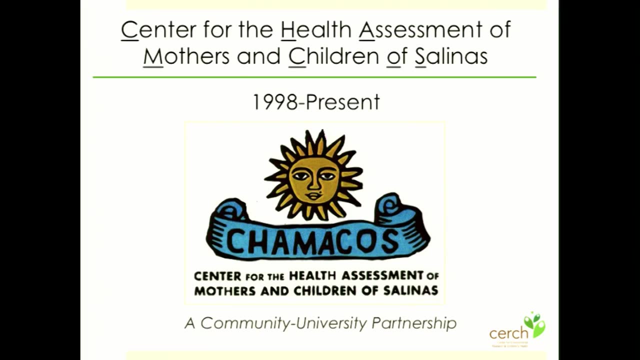 And very good. So we were one of the first and we're only one of four that is still existing since 1998.. And that brings me to our study, The Center for the Health Assessment of Mothers and Children of Salinas. 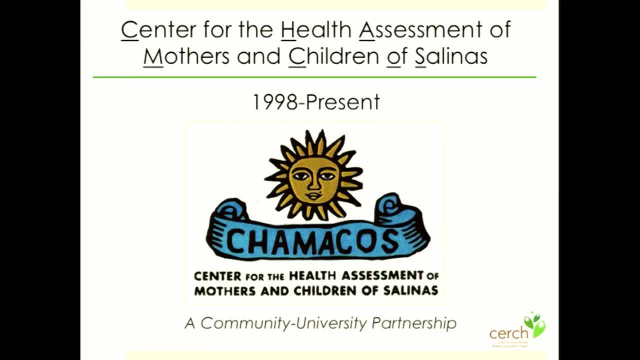 or the CHMACOS study. CHMACOS means kids in Mexican Spanish, And that tells you a little bit about the population that we're studying. So we are a community-university partnership and I'll get into that a little bit more later. 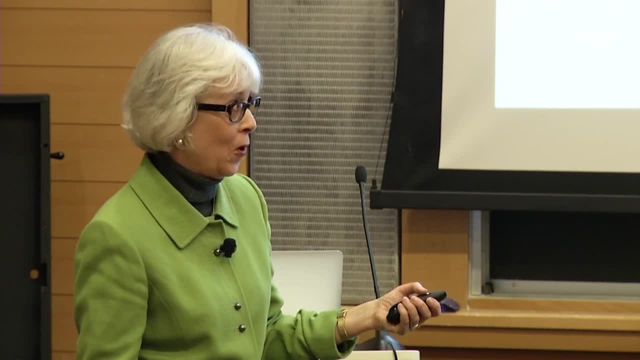 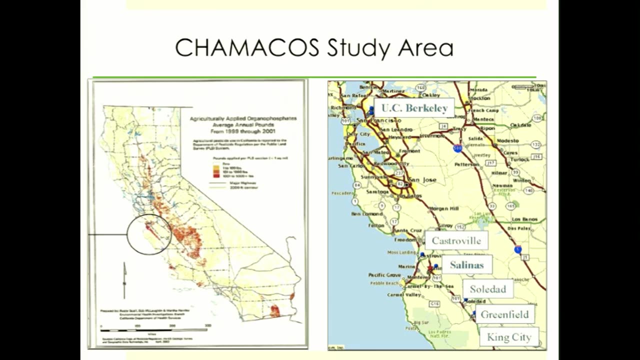 And we started in 1998, and we're still going strong. So where are we studying the population? We are in the Salinas Center, Salinas Valley. That's about a two-hour drive, as you all know, being from the area. 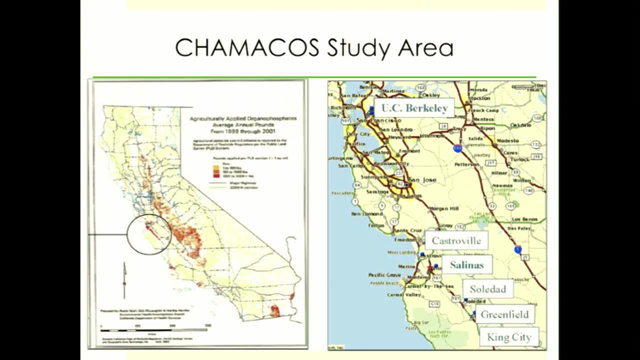 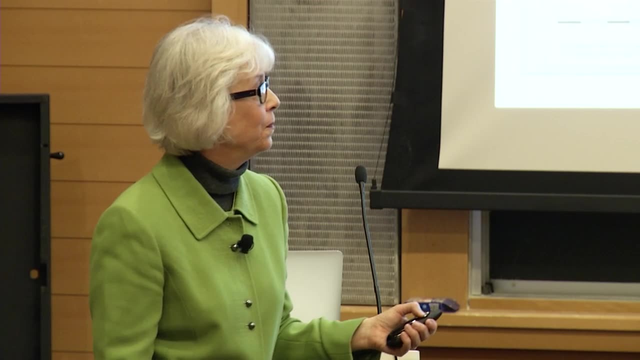 And the valley from top to bottom is about an hour drive And this area is the salad bowl of the nation. California is the leading agricultural state in the United States and Salinas Valley is the salad bowl of the nation. The CHMACOS study. 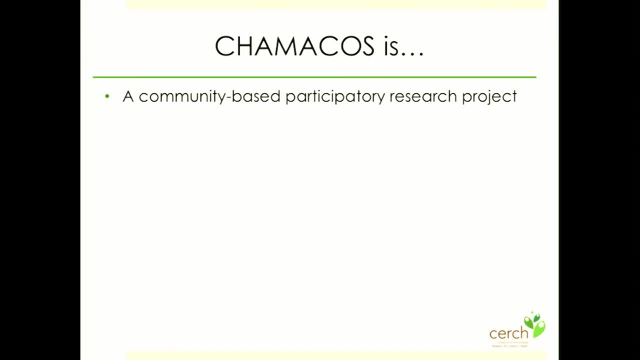 is a community-based participatory research project, Which means that we work closely with our community in devising the research, in disseminating the results of the research. We study the impact of environmental chemicals on women and children's health, And we have four main activities. 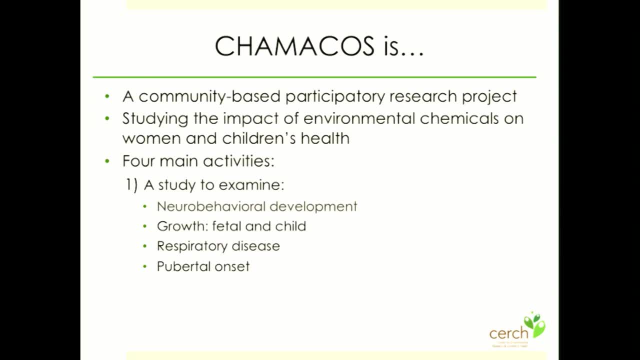 A study to examine neurobehavioral development, growth, both fetal and child, respiratory disease and the age of onset of puberty. We have lots of exposure studies and Asa Bradman over here is in charge of those studies And we have many studies. 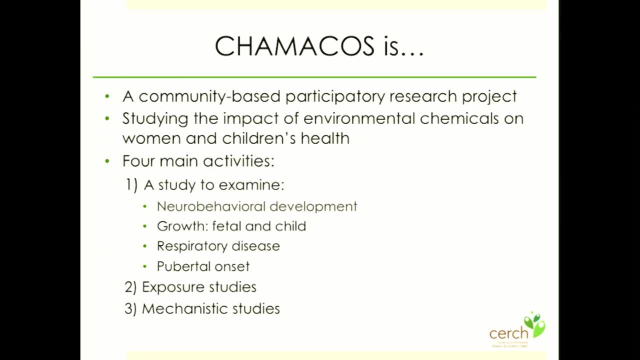 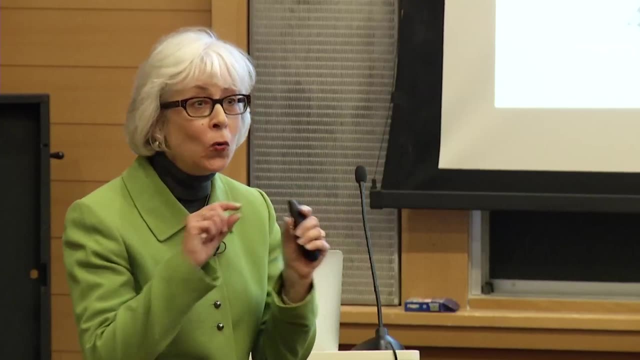 of mechanisms such as epigenetics and genetics, And Nina Holland here is in charge of those studies, And we also have a very strong community outreach and translation core. Today, I'm only talking about one little piece of this and that's on neurobehavioral development. 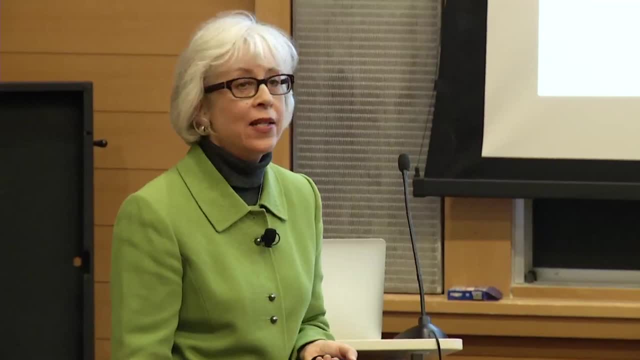 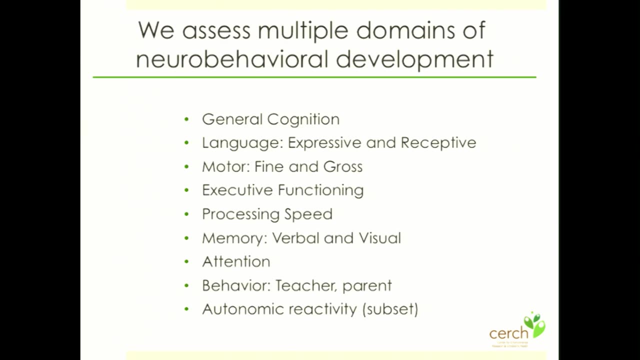 We assess, every time we assess these children, multiple domains of neurobehavioral development, And those are some of them, And we select the ones that we're going to look at with a specific toxicant based on animal studies or pre-existing human studies. 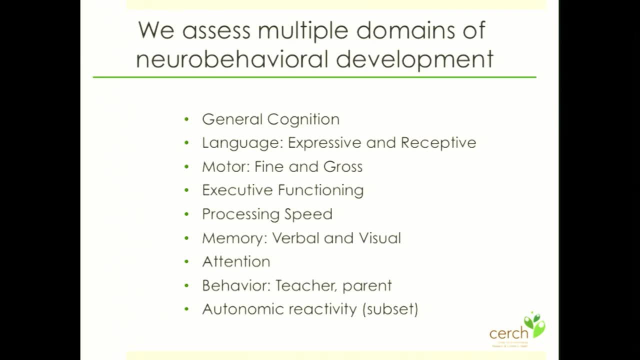 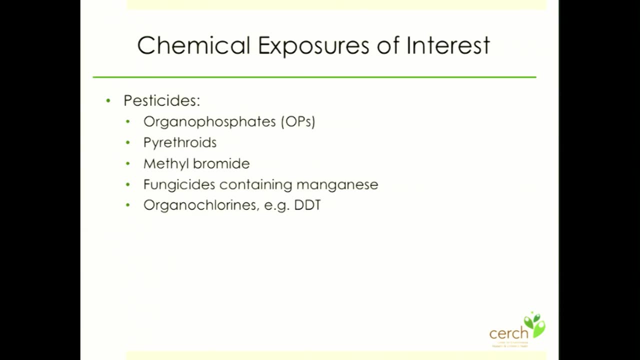 So we don't look at everything for every chemical, because then we're likely to find something. The chemicals of interest that we have studied are pesticides, and I'm going to be talking a lot about organophosphates, or OP pesticides, pyrethroids. 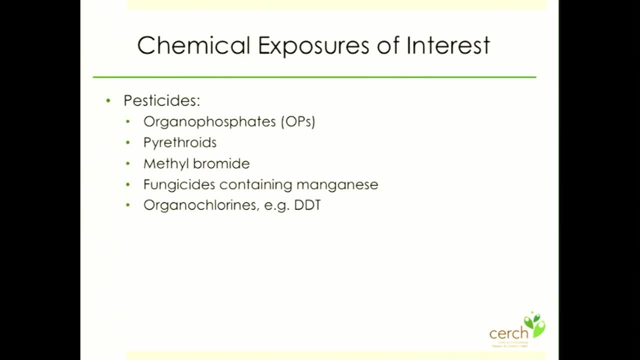 methyl bromide, fungicides and some of the organochlorines, many of which are no longer used. Also, flame retardants, the polybrominated diphenyl ethers, chemicals in plastics, The chemicals of interest that I'm going to talk about. 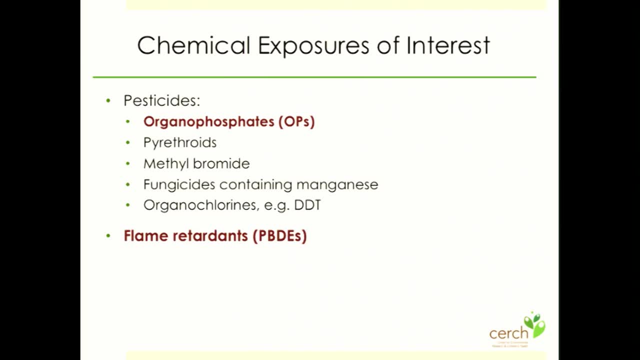 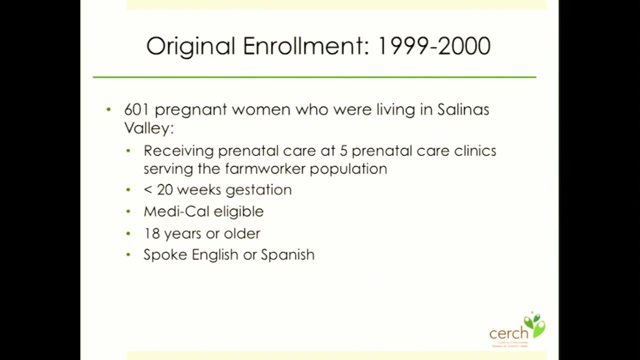 today are the organophosphates and the flame retardants. I'm not going to be talking about all the other things, So let me tell you a little bit about Chamacos and the history of Chamacos In 1999 to 2000,. 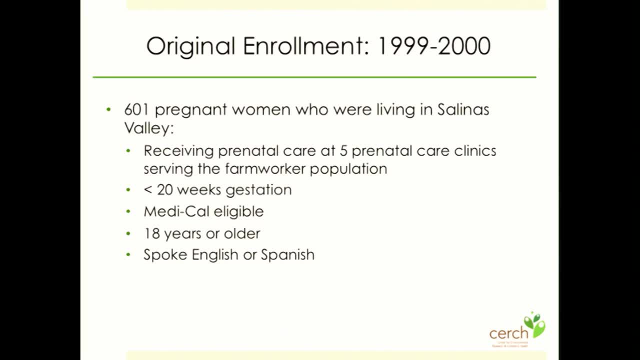 we recruited 600 pregnant women who were living in the Salinas Valley. They had to receive prenatal care at five clinics primarily serving farm worker population. The women themselves weren't necessarily farm workers, but the clinics were community clinics. They had to speak English or Spanish. 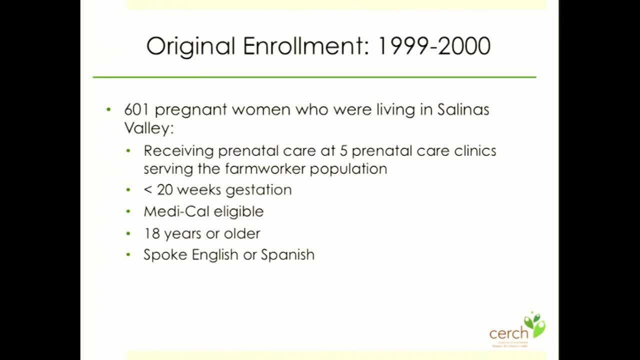 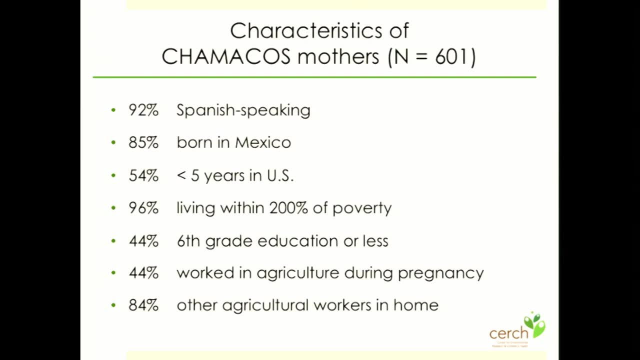 and they were medical eligible, which means that most of the women had to be at a certain income level to receive federal subsidy and state subsidy. What did the Chamacos women look like? 92% are Spanish speaking. 85% of the women. 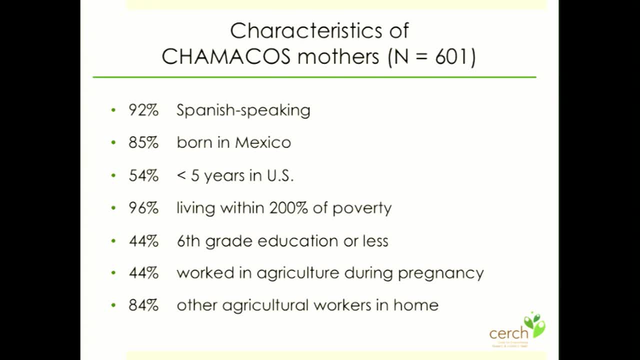 themselves were born in Mexico. half of them had lived in the United States for less than five years. almost all were living within 200% of poverty because that was the requirement being in Medi-Cal Education low. about half of the women worked in agriculture themselves during pregnancy. 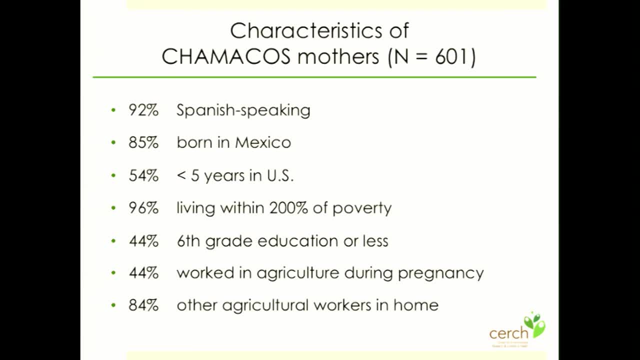 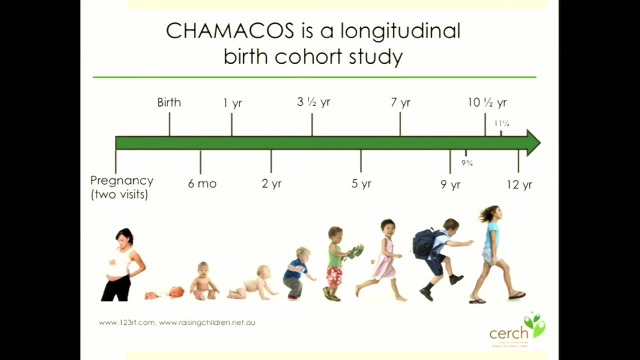 but even if they did not work in agriculture, someone in their household worked in agriculture. So we like to say that this population is a low income, primarily farm worker family population, Latina. The Chamaco study is a longitudinal birth cohort study and what we mean by that. 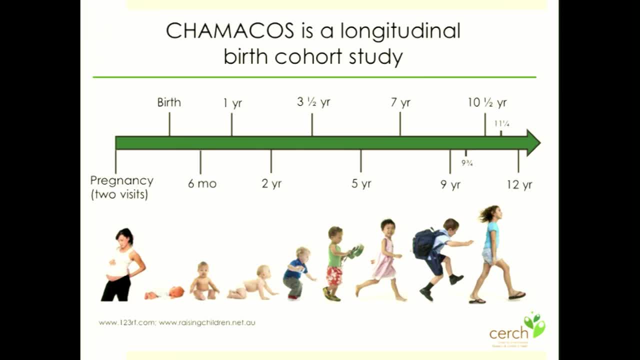 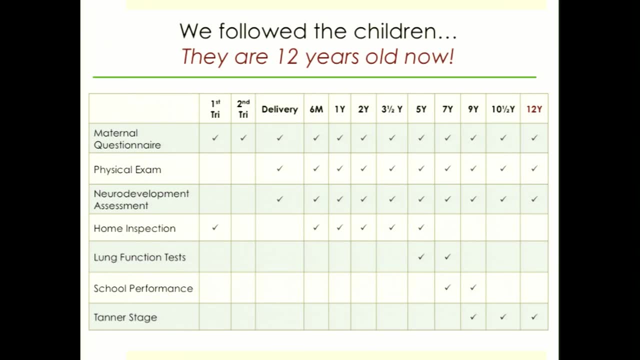 is. we started in pregnancy and we have followed the children over time. Specifically, we have interviewed the mothers twice in pregnancy, once at delivery, when their children were six months old, one year old, two years old, three and a half years old, five years old. 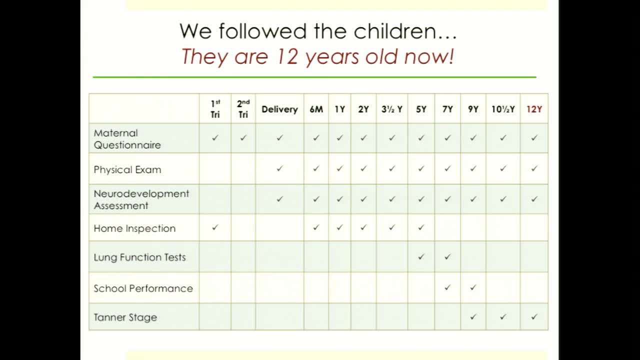 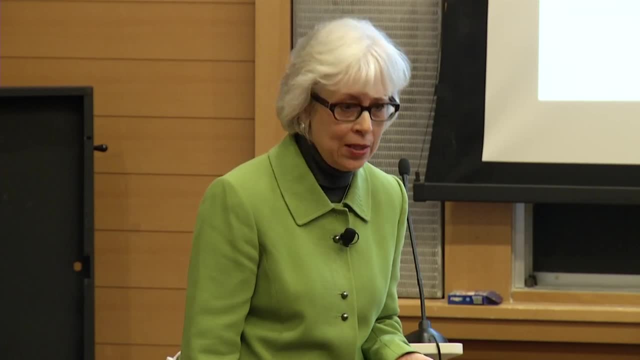 seven years old, nine years old, ten and a half years old and the children are 12 years old now. We have done physical exams on these children. We have done detailed neurobehavioral development assessment on the children We have looked at. 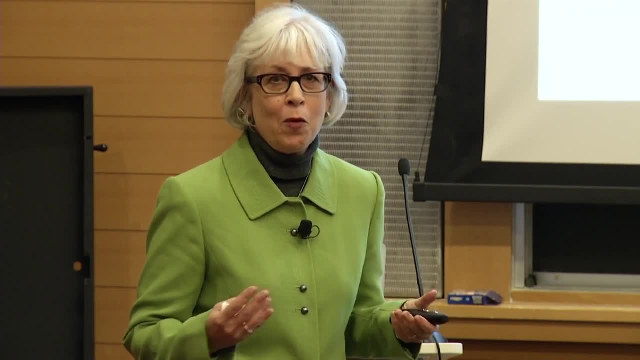 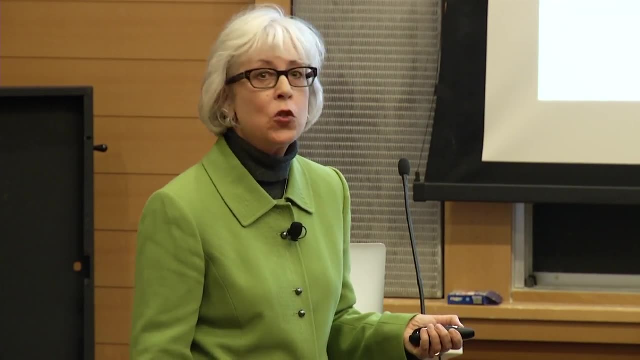 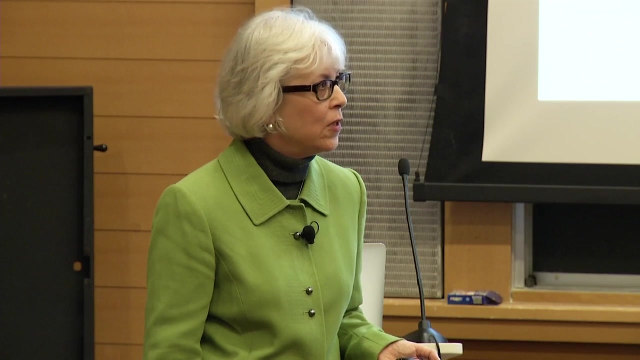 thousands of homes. In fact, in some ways we know more about farm worker housing in the Salinas Valley than almost anybody. We have done spirometry tests or lung function tests on the children. We have asked the teachers how the kids perform in school. 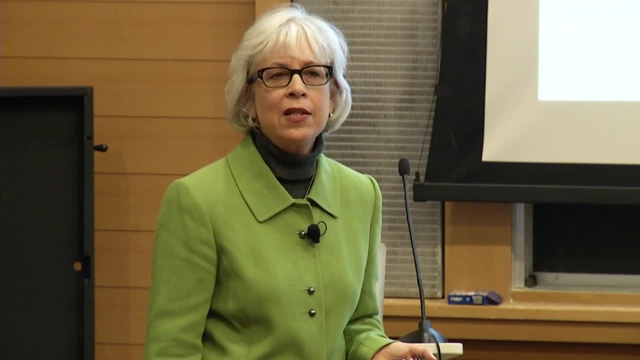 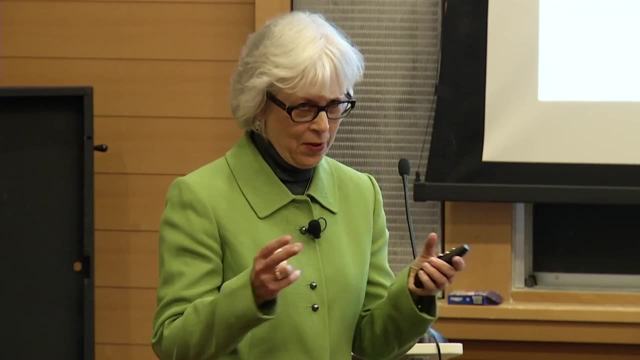 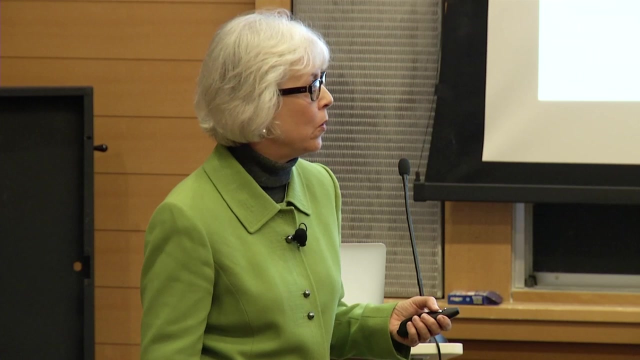 So we've gone to the teachers And most recently we've been examining the children: their breasts, their testicles, their pubic hair, depending on whether it's male or female, to look at the age of onset of puberty. So we actually do physical exams to look. 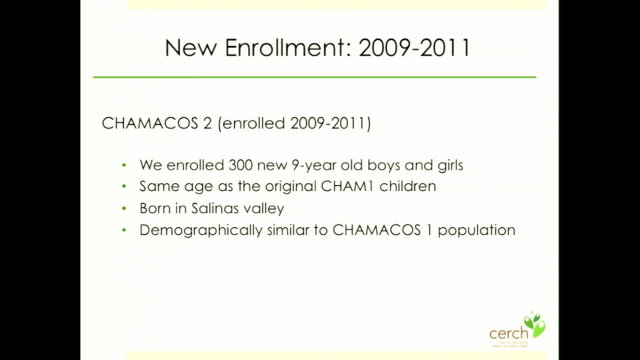 at this the gold standard In 2009,. we received more money and we actually recruited even more kids into the cohort, But now we started at age 9.. And these kids were demographically similar to the Chimacos 1 kids. 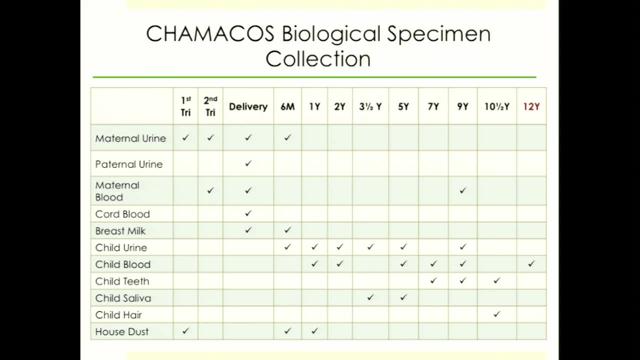 We have collected lots and lots and lots of biological and environmental samples And they're all stored in Nina's biorepository, Which I'm not saying where it is, School of Public Health's biorepository, Okay. And we've collected maternal urine multiple times. 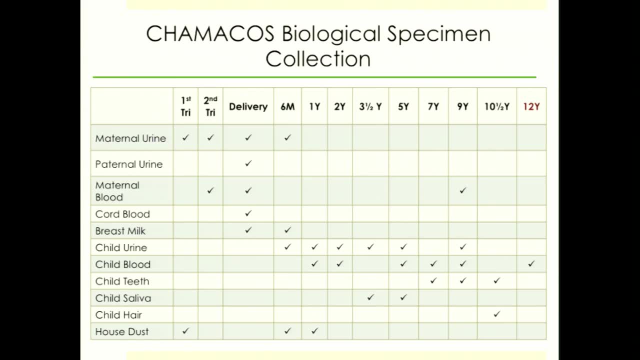 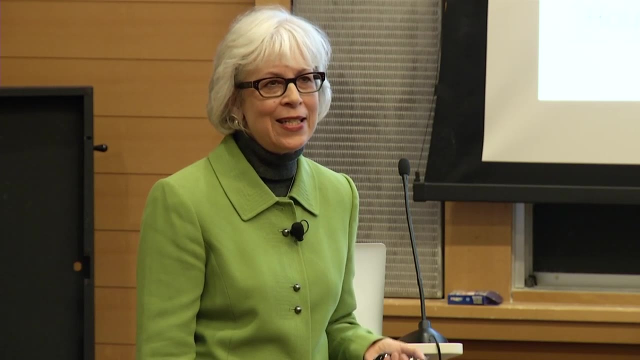 Paternal urine, maternal blood, cord blood, breast milk, child urine multiple times. child blood multiple times. deciduous teeth from the children, saliva, hair and house dust. So we'd like to say that we knew what we were doing when we 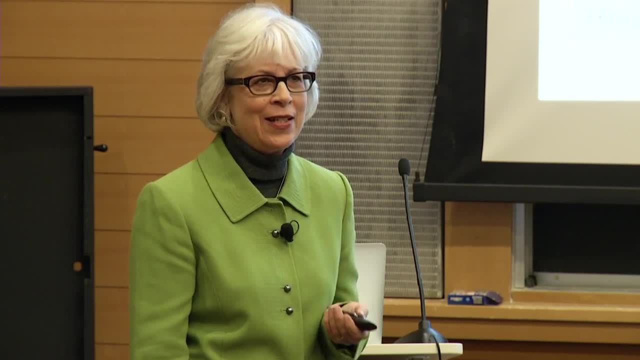 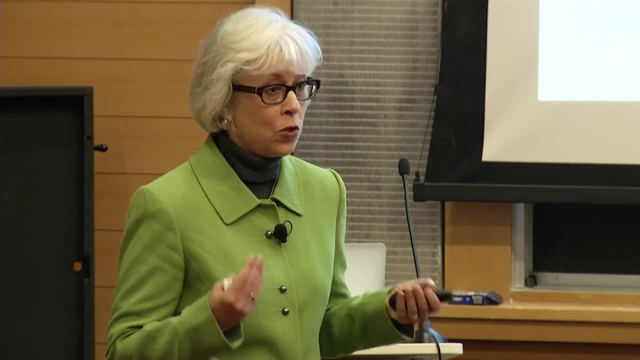 decided to collect all these biological samples, but I also like to say it's because I didn't know what I was doing, and neither did Asa, And so we collected more biological samples. sometimes we weren't sure the best way to analyze these different chemicals. 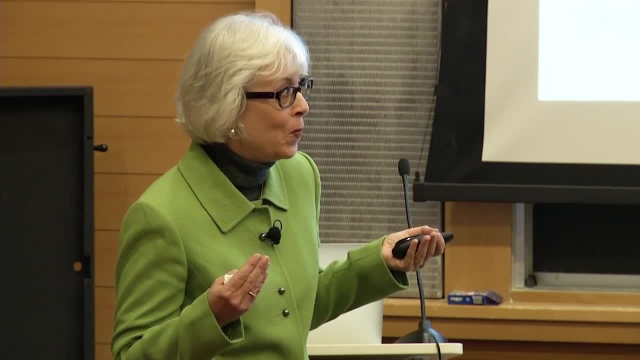 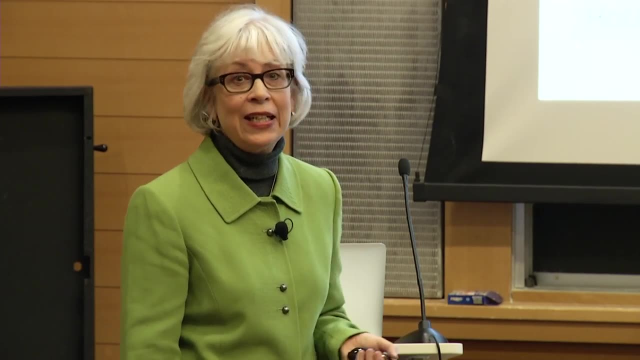 at the time that we collected them. So, for example, we thought at one point that measuring organophosphates in saliva was the way to go, but it turned out not to be. We have collected and stored over a hundred thousand samples- A hundred. 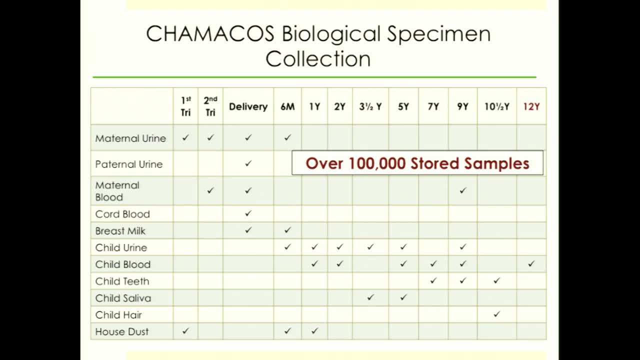 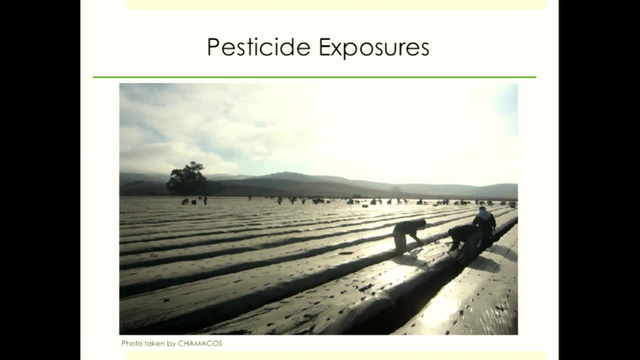 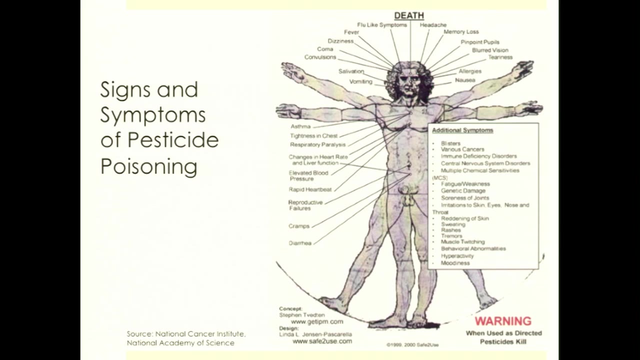 thousand samples, which means that we have lots of samples to do future studies, Genetic, epigenetic, biomarker studies. So let me talk about pesticide exposure. It is well known, like it was with lead, that high doses cause neurological problems. 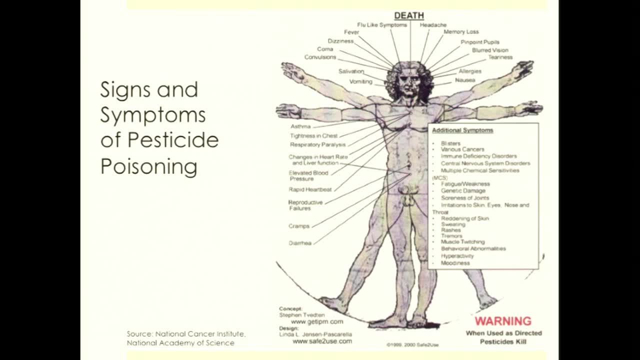 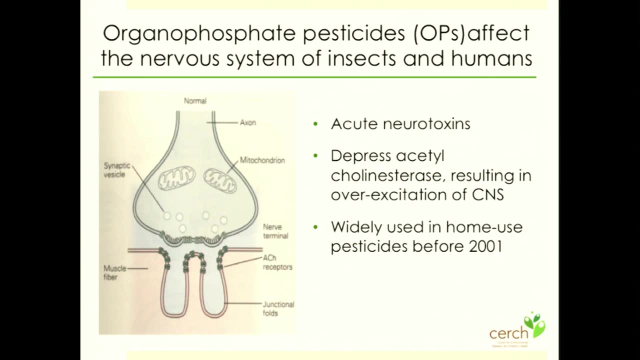 People enter into coma every year from pesticide poisoning. We know this. We also know the mechanism by which these pesticides affect the nervous system. This is well established. The question is whether low dose exposure also affects the nervous system. So let me tell you a little bit about the 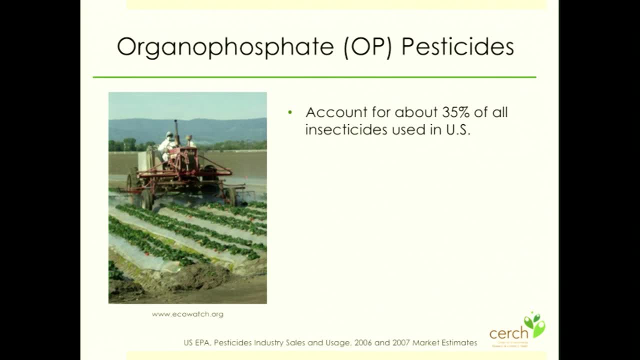 organophosphate pesticides. They account for about a third of all insecticides used in the United States. There are more than thirty million pounds used per year. They are most used in California because California is the leading agricultural state in the nation. They 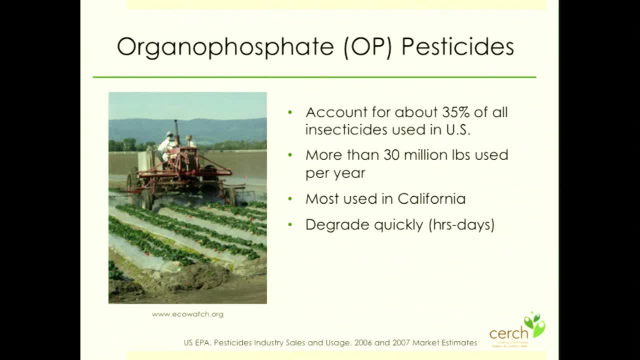 degrade quickly in the body and in the environment, which makes them harder to test for, And they are excreted in urine as something called dialkyl phosphate metabolites. I'm going to talk about them as either OP metabolites or DAPs. 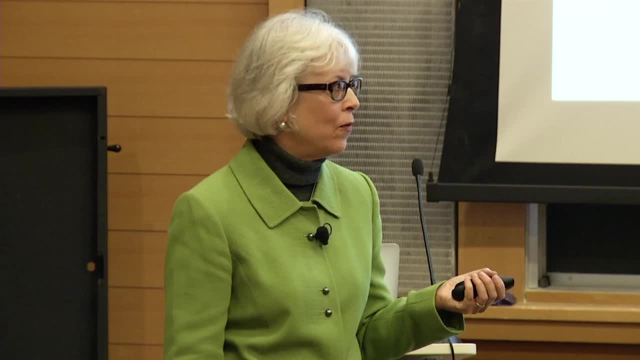 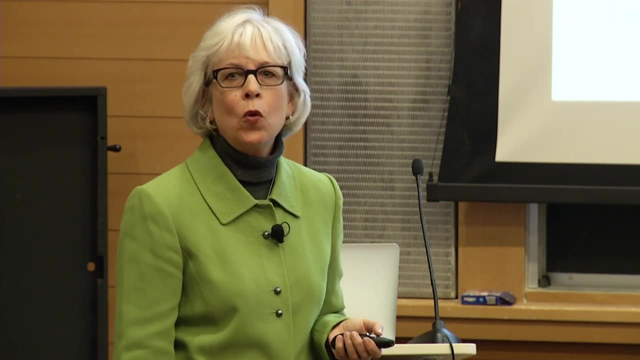 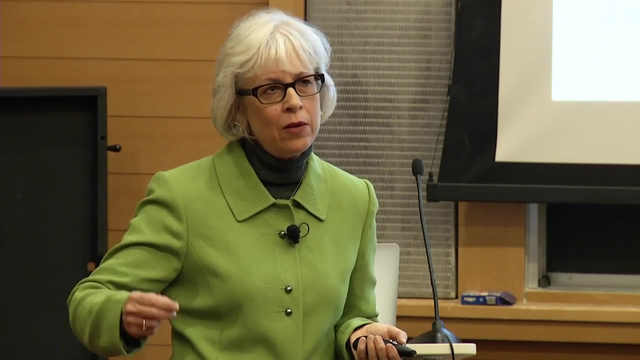 So if you hear me talk about DAPs, they are the metabolites of organophosphates. We are very fortunate in California that it is required by law that every pesticide application the time date, the amount, the kind of pesticide and the 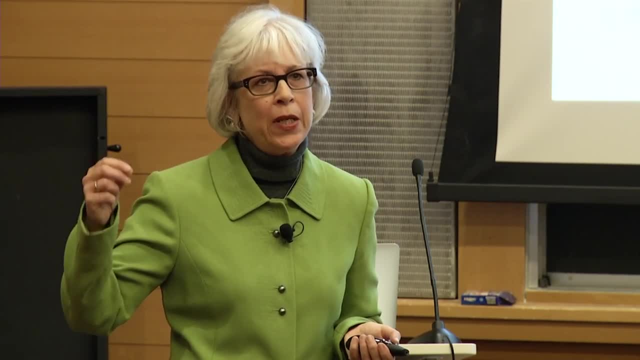 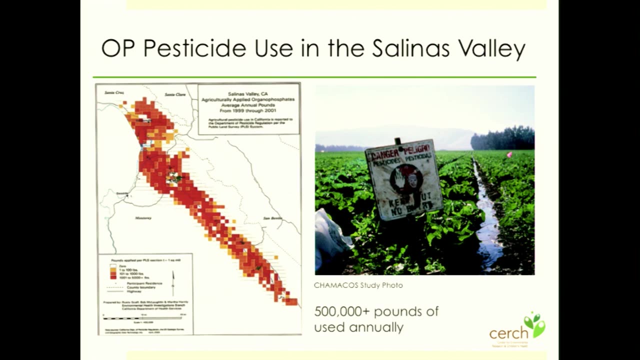 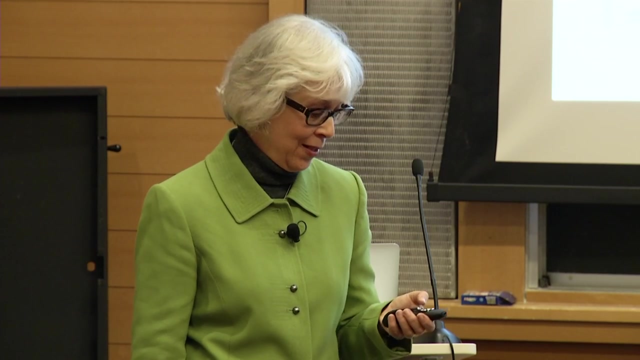 location of that pesticide application needs to be reported to the Department of Pesticide Regulation. We are the only state in the nation and the only place in the world that this happens, which makes it great. if you're doing a study on pesticides, We determine. 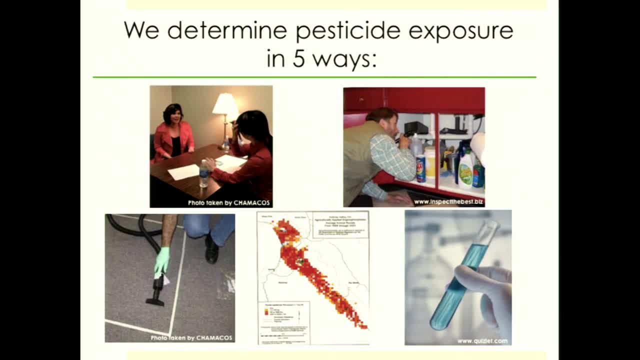 pesticide exposure in five ways. We interviewed the women, we did home inspections and we looked for pesticide containers in their homes and their garages and we recorded the EPA registration numbers so we knew what chemicals were in that pesticide. We collected dust samples. 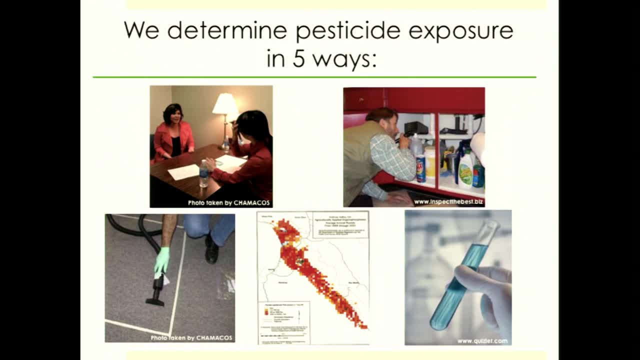 and we measured pesticides in some of those dust samples And because of that required reporting of the pesticide use in agriculture. we could get the GPS coordinates of every woman's house when we went to their home and plot it on a map and see what pesticides were applied. 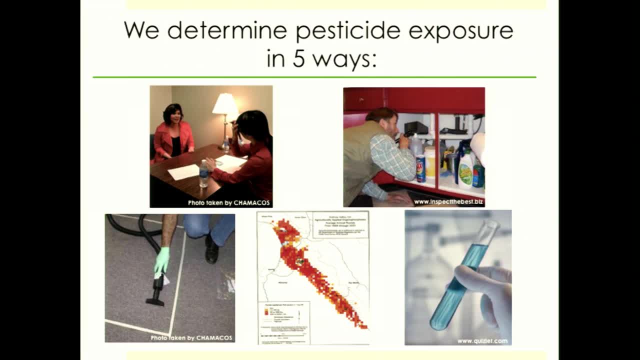 near where she lives And so we could look at geographic mapping- and we have a prime medical geographer right here, Mike Jarrett, who's been helping us figure this out- And we also collected these biological samples. So what did the biological samples look like? Remember? 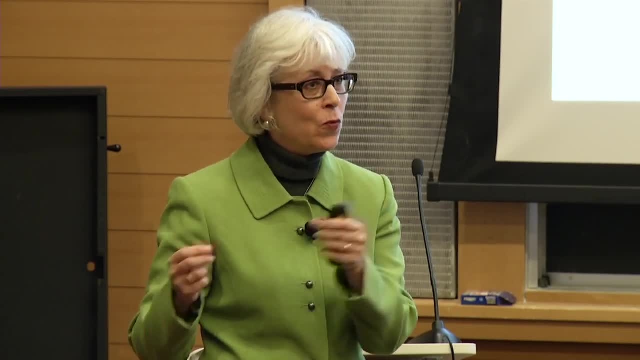 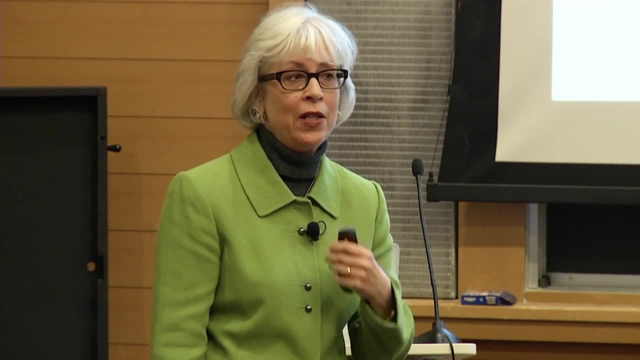 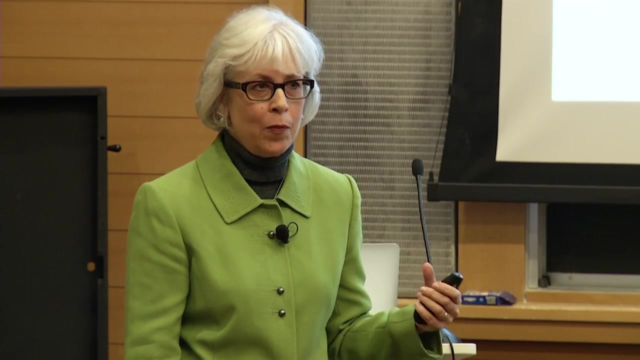 I measured. we measured the dialkyl phosphate metabolites, which are metabolites of organophosphates, the DAPs, And so we are fortunate that the same laboratory that analyzed our urine samples also analyzed the samples for the general US study. 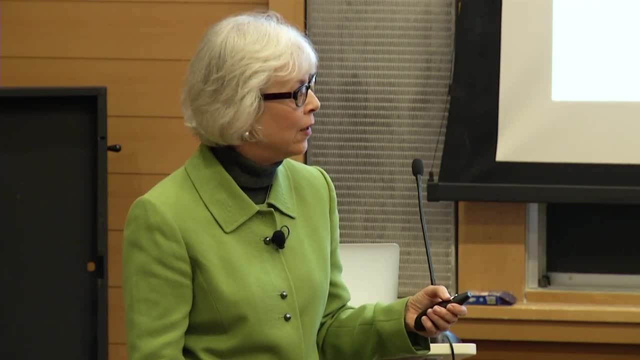 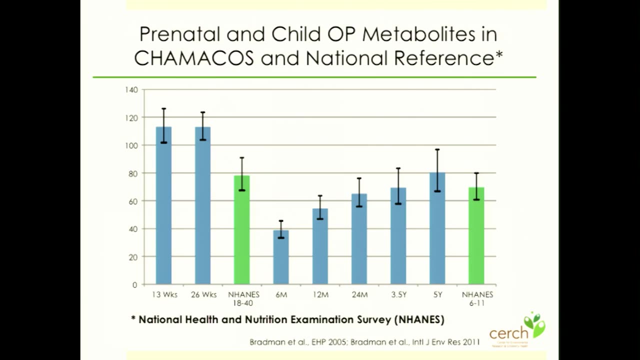 population and that's the National Health and Nutrition Examination Survey. that's done every couple of years, And so we could compare the results of the Chimacos women which are in the blue compared to the general US population of women of reproductive age, And so 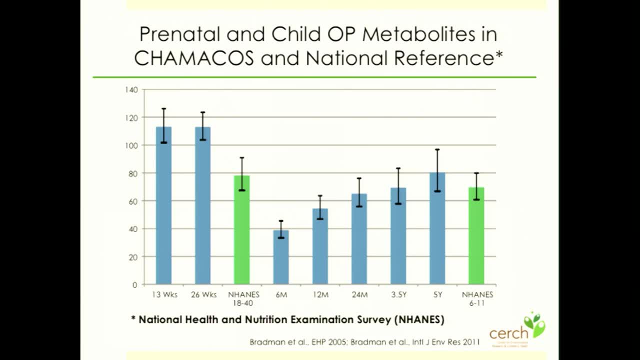 you can see that the women in Chimacos had significantly higher DAP metabolite levels, or the OP metabolites, than the national reference data. You can also see in the children the urines were measured six months, 12 months, 24 months. 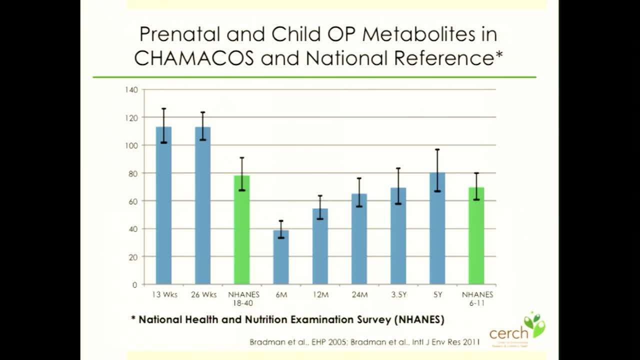 three and a half years and five years that there was a steady increase in the amount of DAPs in their urine, But by five years our children had significantly higher levels than the children at six to 11 years of age, because they didn't look at children younger than. 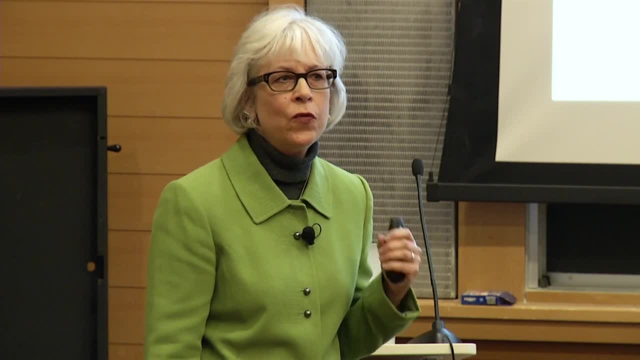 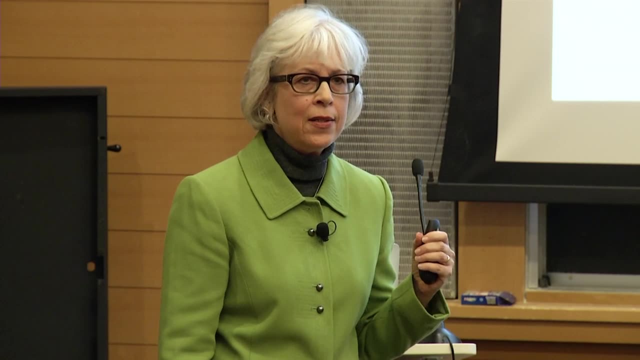 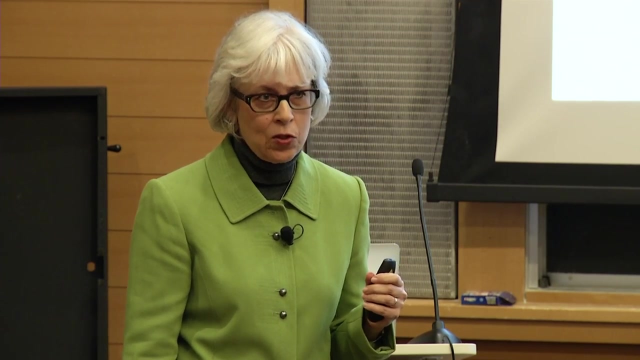 six in NHANES. So we have significantly higher pesticide exposure, based on the OP metabolites, in the women and in the children relative to the general US population. Not very surprising, given that these children and women live in an agricultural community. So were these? 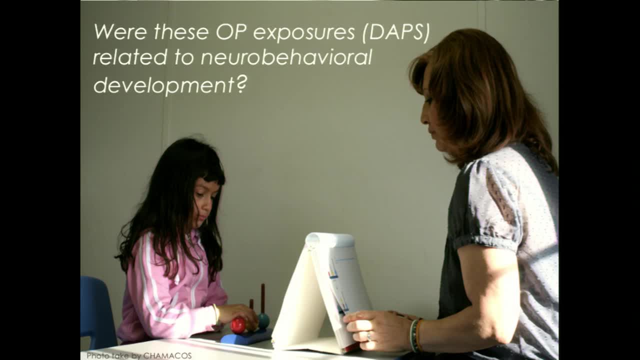 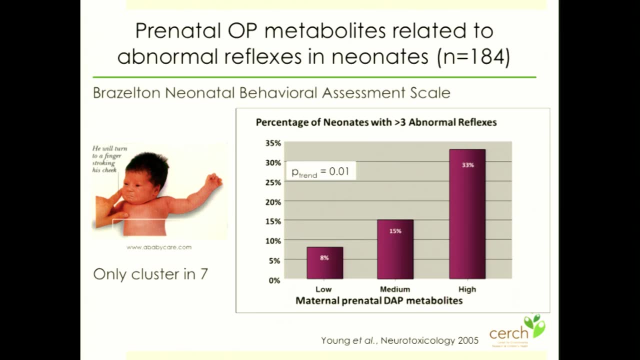 OP exposures that is measured by the DAPs related to neurobehavioral development. When the children were newborns we did something called the Brazelton Neonatal Behavioral Assessment Scale on the children and there are seven different clusters of behavior that are measured. 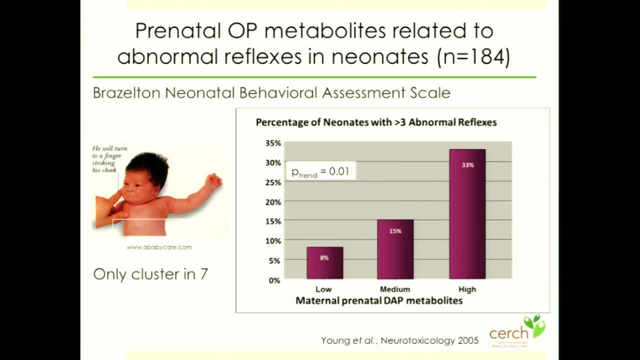 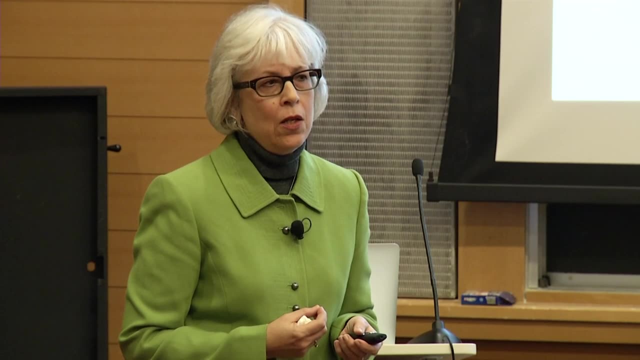 by the Brazelton. We found a significant dose-response relationship between the mother's DAPs in her urine during her pregnancy and whether the child had abnormal reflexes at one month of age. So this sounds like okay one out of seven clusters. 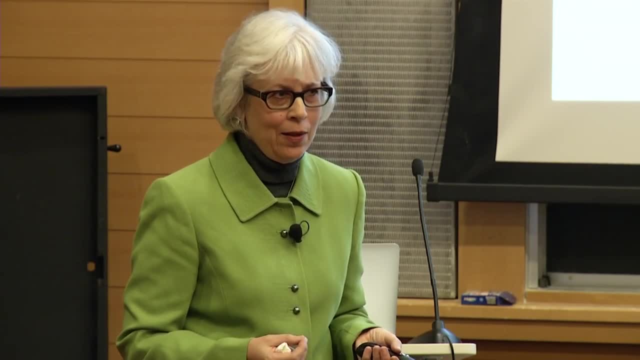 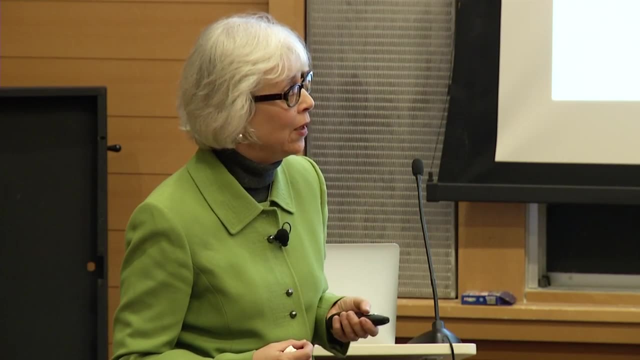 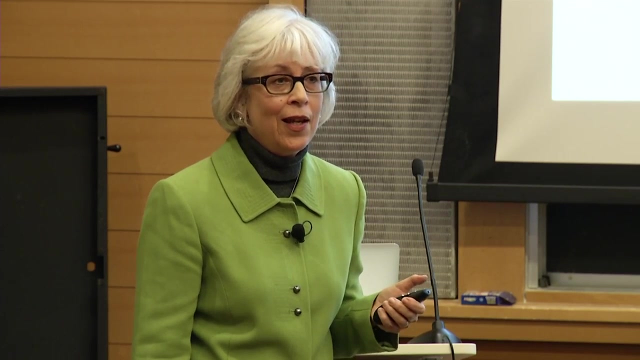 being significantly related doesn't sound like very important results. However, right after we published this, a study came out of Mount Sinai doing the exact same thing- Mount Sinai, New York- where they looked at the OP metabolites in children living in New York City and 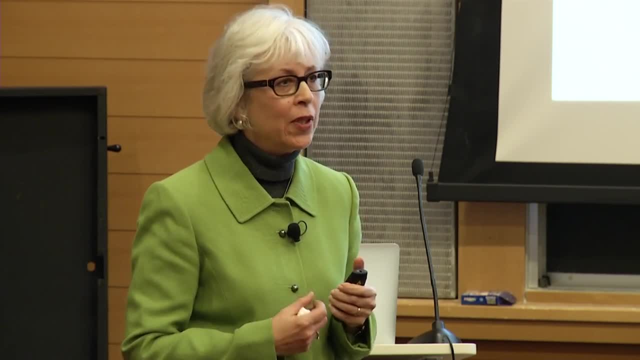 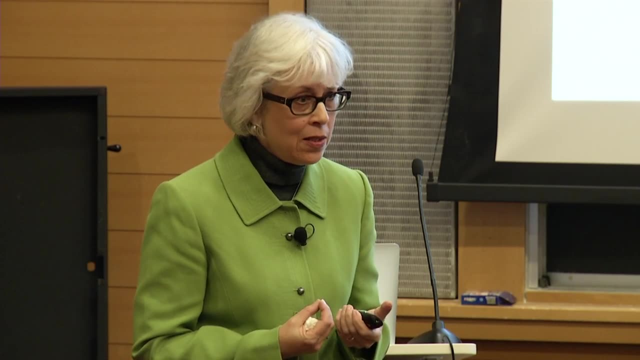 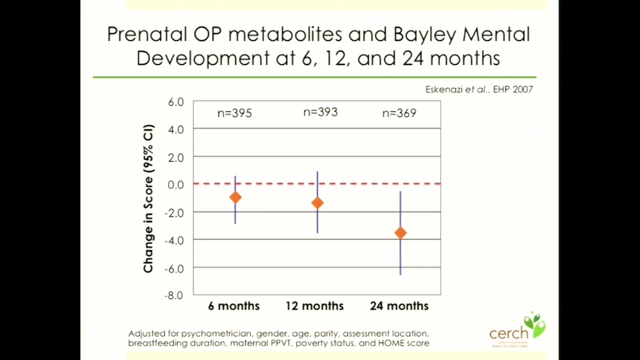 also found a relationship between these OP metabolites in the mother during pregnancy and abnormal neonatal reflexes in the child. So we had an independent confirmation of the result. Now the children are older, At six months, 12 months and 24 months. 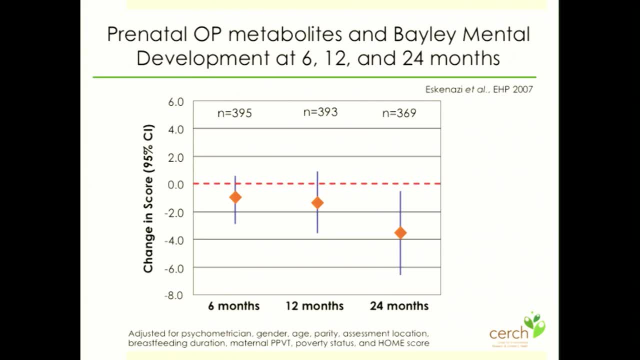 we did the Bailey Scales of Infant Assessment And that scale looks at both cognitive development in the child as well as psychomotor development in the child. So motor development- We did not see any associations with motor development in terms of in relationship to the mother's levels. 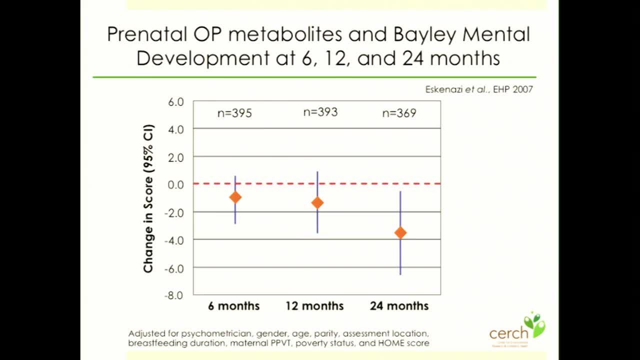 of these metabolites in her urine during pregnancy. Nor did we see an association with mental development when the children were very young, at six months or 12 months, But at 24 months we did. Now let me walk you through. I'm going to show you lots of figures like this: 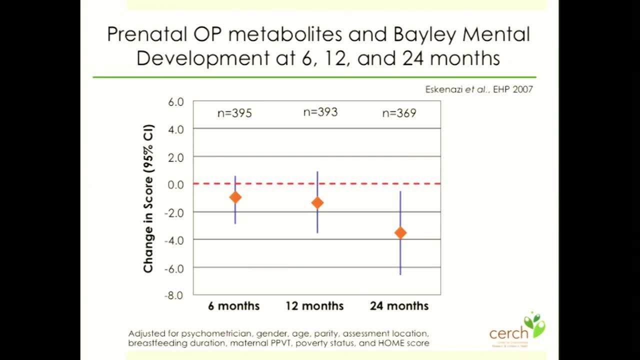 so if you're not used to seeing them, I just want to walk you through them. This is what I'm going to call the no effect line. This is a change in score, So if you see a decrease in the average, this point is like the. 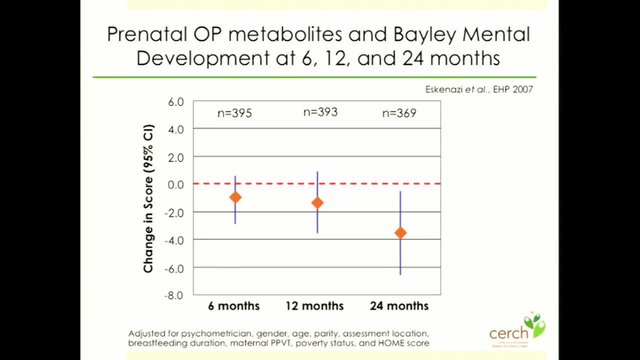 average for the group, then it means that you're seeing it go down. If the top of this point here crosses the no effect line, it means it's not statistically significant. So it means that it could be due to chance. Okay, So what? 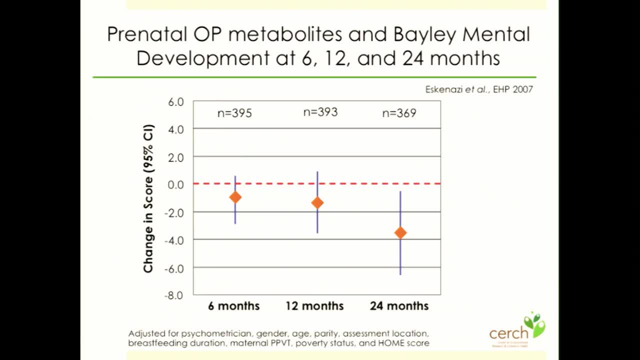 we see here is that six months of age. for every tenfold- and this is on a log scale, so excuse me if I say this in a very wordy way- for every tenfold increase in the mother's levels of these DAPs in her urine, these OP. 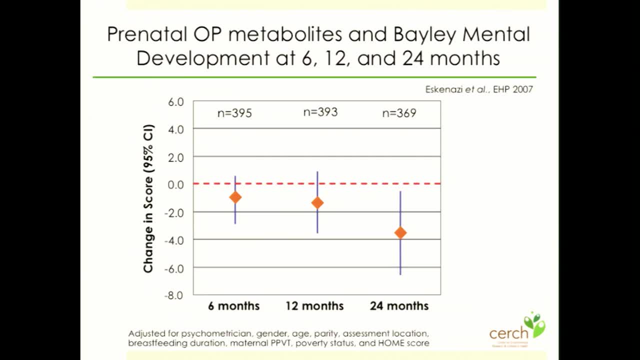 metabolites in her urine. we see a non-significant one-point decrease in the child's mental development. At 12 months a little bit more, but still not statistically significant. But at 24 months we see a four-point drop And for those 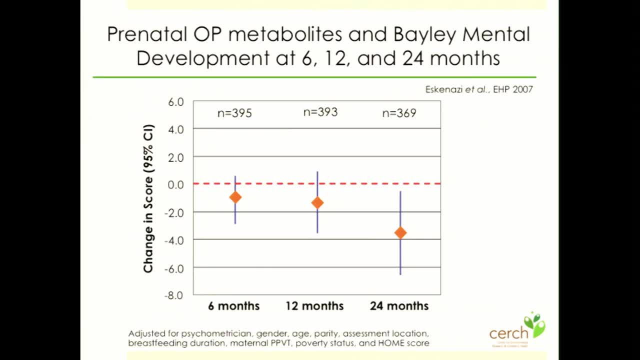 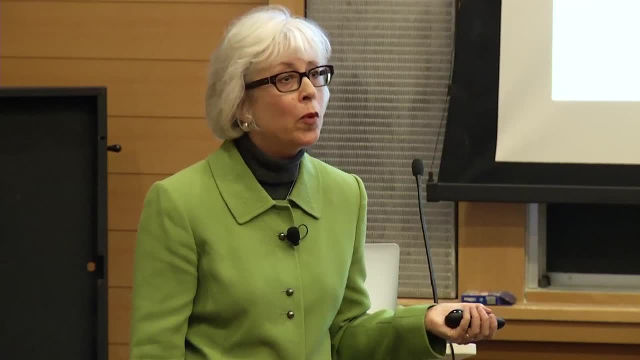 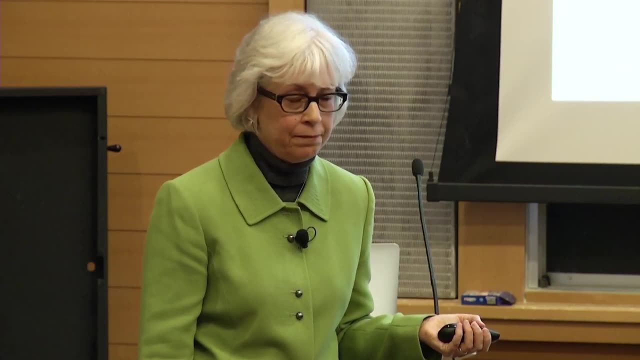 of you who are interested in standard deviations, it's about 15.. So it's about a quarter of a standard deviation here. So again, not much to write home about, except another couple of centers. children's centers confirmed the same result. Now the children are school age. 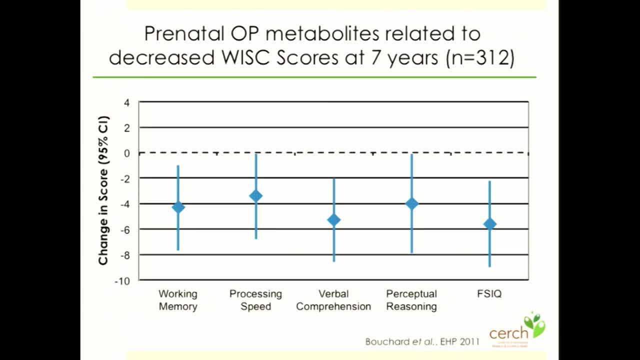 Now we have results that might actually have some predictive validity. Looking at a two-year-old may not actually tell you how they're going to function later on, But when you're looking at seven-year-olds it has greater predictive validity. And what we're seeing? 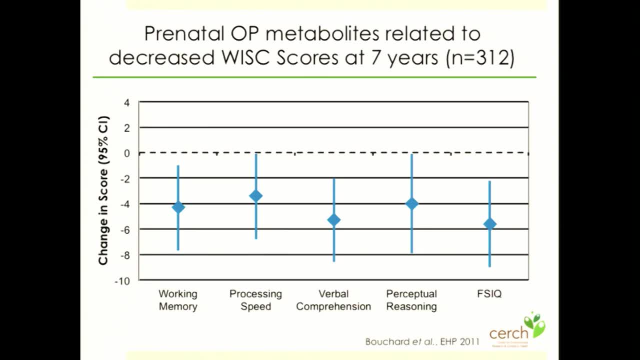 is that the prenatal exposure to the OPs measured in the mother during pregnancy are associated with decreases in IQ at seven years of age. And here again is the no effect line. Here are four different domains of subscales of the Wechsler Intelligence Scale for children. 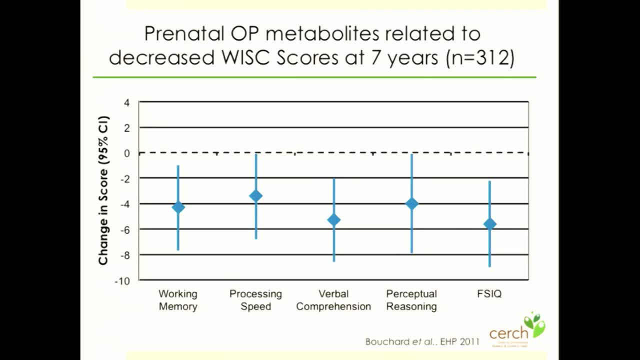 Working memory, processing speed, verbal comprehension, perceptual reasoning, and these four together comprise the full-scale IQ. Okay, And you see a significant drop in every one of these domains associated with the maternal levels of those OPs during her pregnancy. We do not see an association. 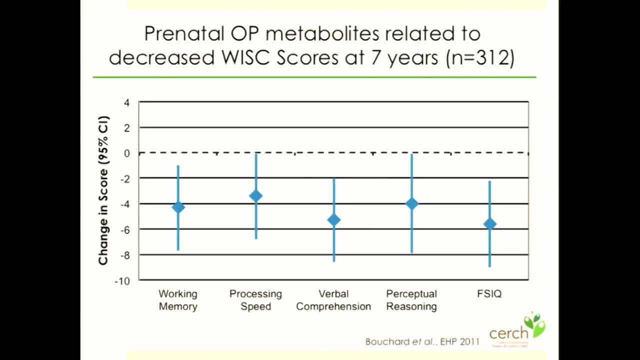 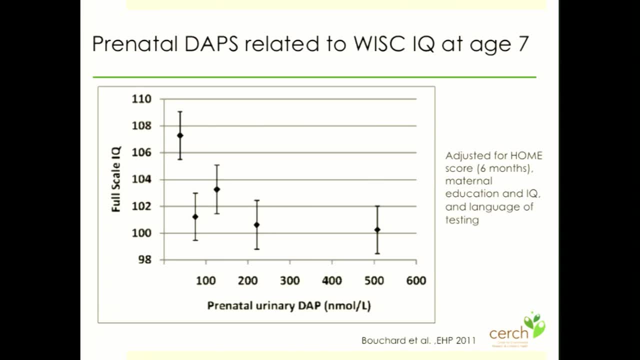 with the child levels. So the association is with prenatal exposure. Another way to look at this is if you divide the population into five equal groups And you have those that are the least exposed, the lowest 20% and the highest 20%. 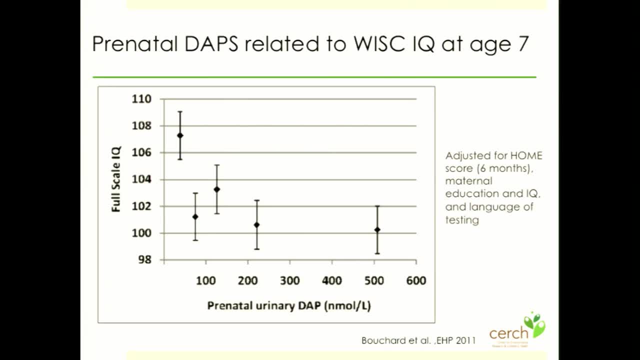 You see about a seven IQ point difference or, for those of you who like statistics- about half a standard deviation in those that are highly exposed in utero versus less exposed in utero. That is not only clinically significant, it's significant on a population. 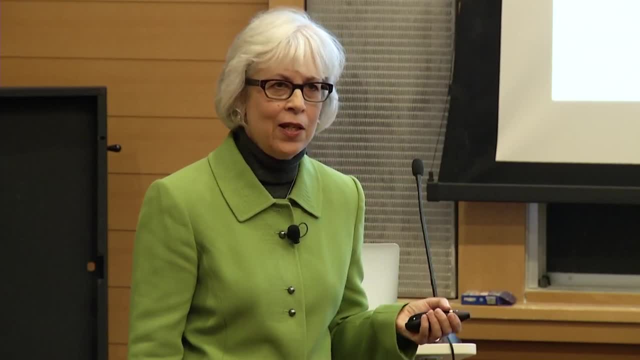 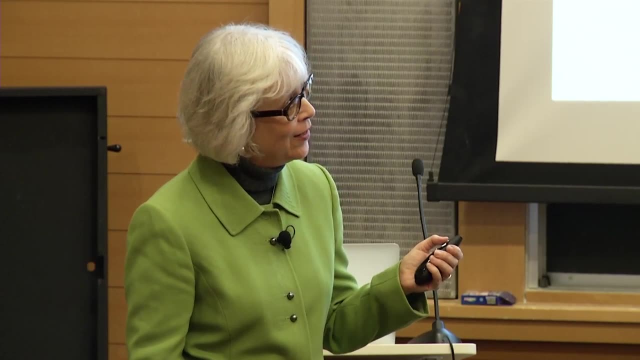 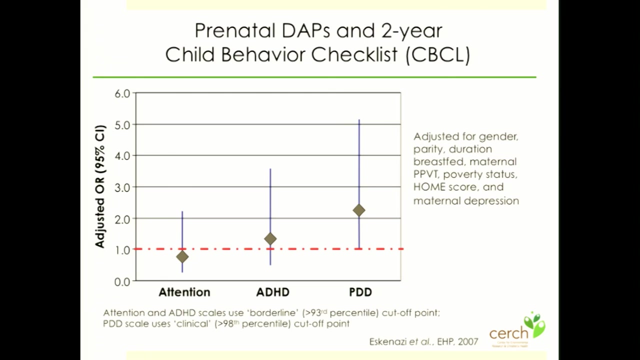 level, And again similar results in two other studies published at the same time as this paper. In fact, today, yesterday, we found out that this paper won the paper of the year for the journal. Let's turn to behavior. Not just cognition, but behavior. 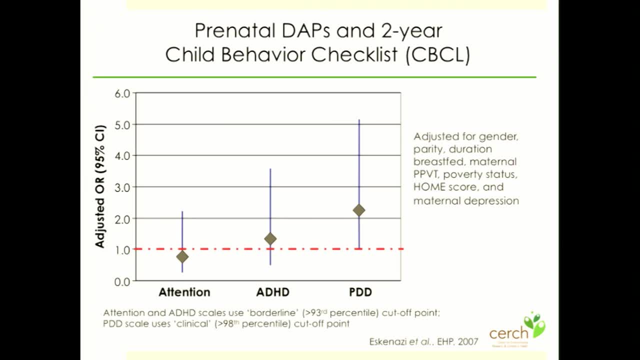 At the time that the children were two years of age, we asked the mother: so tell us about the behavior of your child, And we used a standardized scale called the child behavior checklist. We asked the mother at two and a half years about the child. two years. 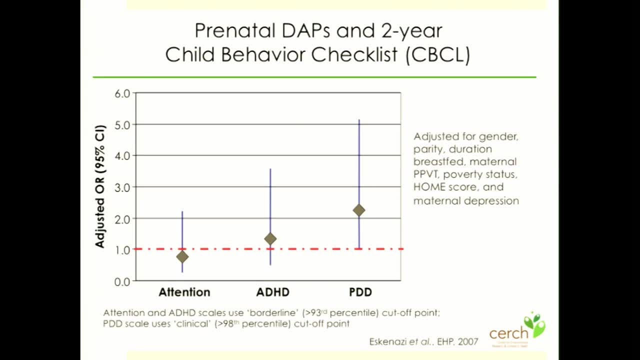 about the child's attention, attention deficit disorder and hyperactivity and symptoms of pervasive developmental disorder. And here is that no-effect line and we adjusted for all sorts of things statistically So you can see there was no association between prenatal exposure to these OPs as measured by the 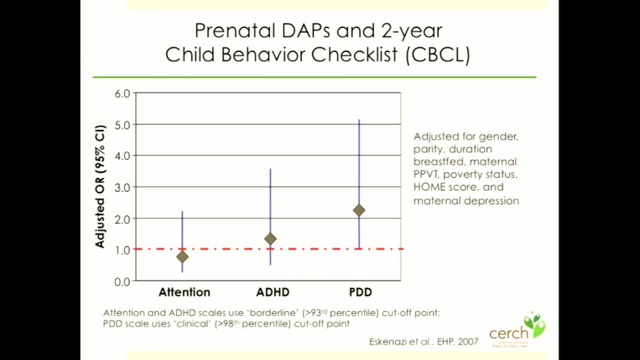 DAPs and the attention of the child reported by the mother, and we know maternal report is not necessarily unbiased And there was no association with ADHD at two years of age. But there was a statistically significant, although very wide, not very good precision. 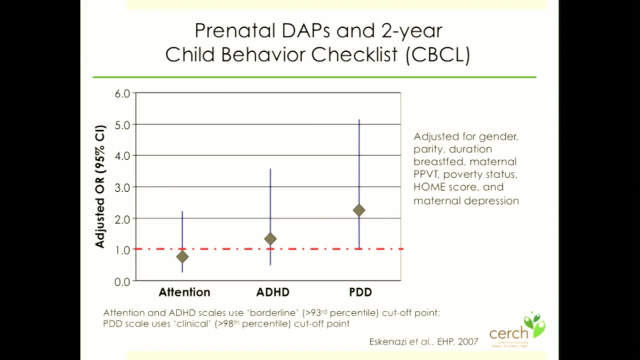 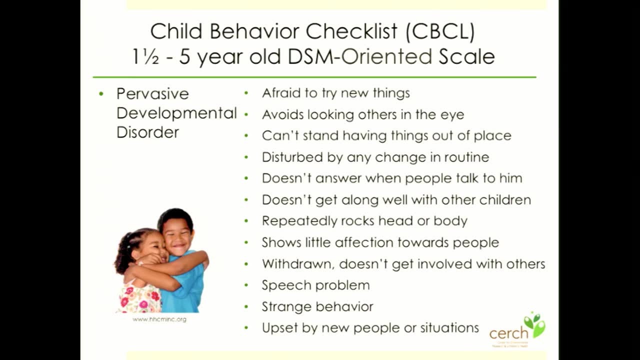 of pervasive developmental disorder and the maternal levels of these DAPs in pregnancy. So what do we mean by pervasive developmental disorders? for those people that are not psychologists in the room, These are the actual questions that are on the child behavior checklist. Is your child? 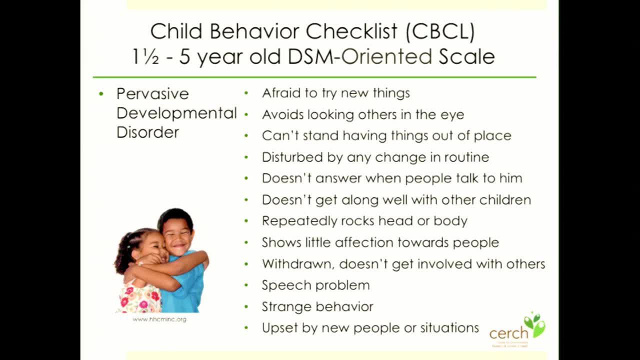 afraid to try new things, Avoids looking others in the eye, Can't stand having things out of place. Very much like autism spectrum. So we're seeing an association between the maternal DAPs during her pregnancy and the child being reported by the mother. 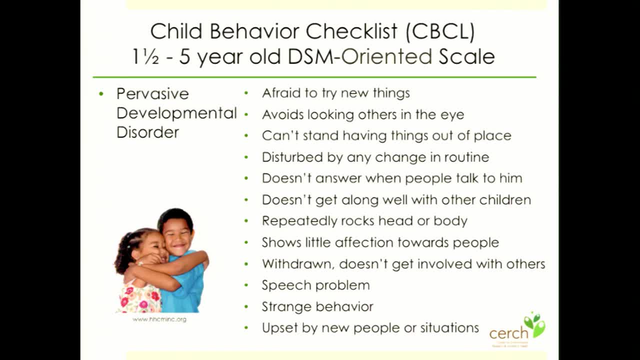 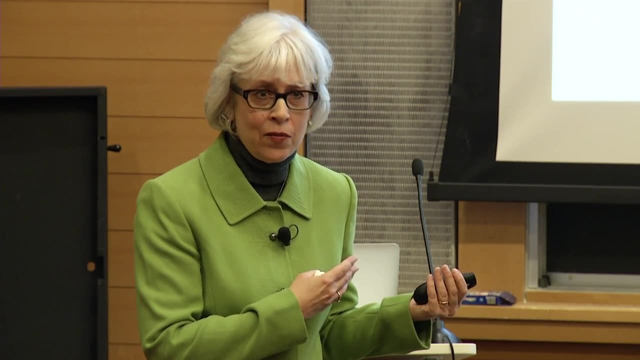 as having autism spectrum type of symptomatology, Not only at two years, but we replicated this at three and a half years and at five years. What this means has to be replicated in a much larger study of children with autism, not in this kind of design. 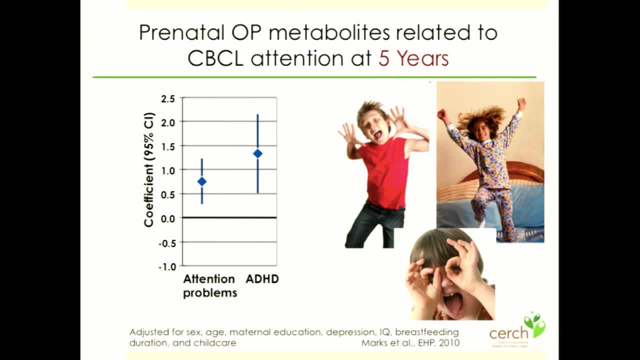 So what about attention? I showed you no association at two years, But by five years of age again on the child behavior checklist. this is based on maternal report. we see that there is a statistically significant increase in the number of attention problems reported. 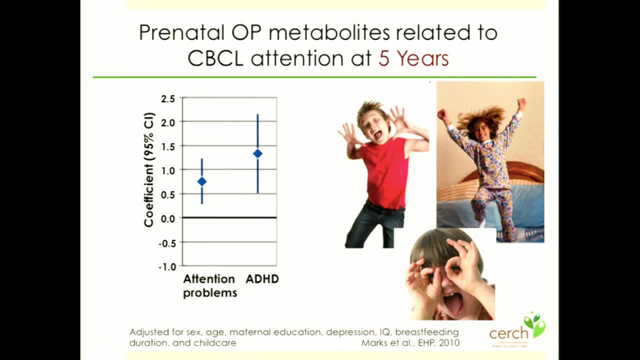 by the mother in relationship to her levels in pregnancy. Now she doesn't know what her levels are in pregnancy, So she is a blind reporter And also with increased problems of ADHD, And these problems were primarily in boys, Which is often what you see with 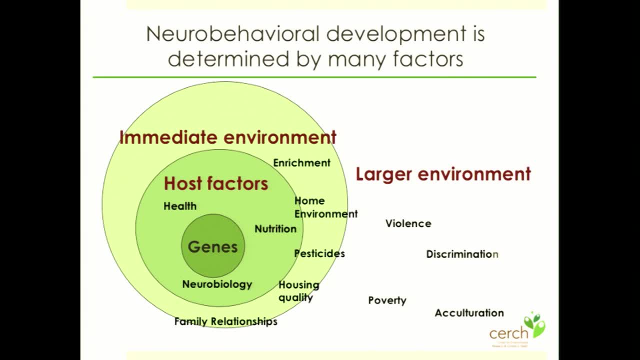 attentional problems. Now I just want to point out that we're looking at one small factor in relationship to a very complex- I call it my onion here- things that influence neurobehavioral development From everything, from the external larger environment, the violence experience, into the community, the 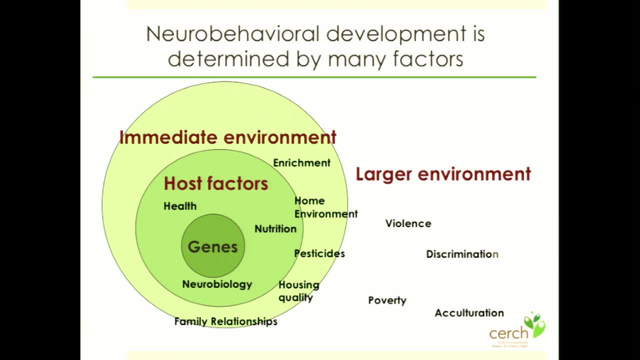 population, poverty, acculturation, how all of these things influence the child's development, Health, nutrition, neurobiology, and how all of these things interact with each other. But also the child's genes, the genetic makeup of the child. 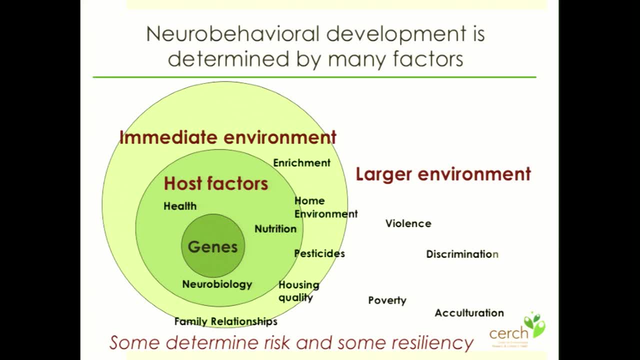 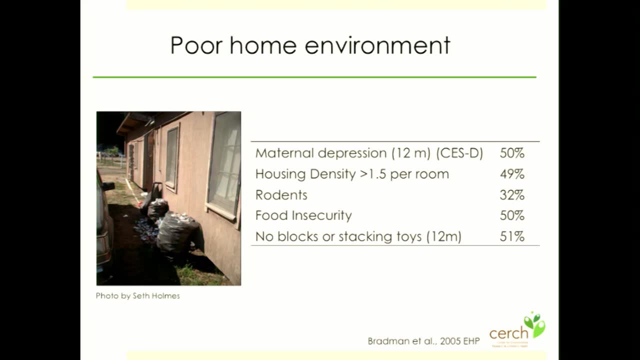 Some of these factors determine risk and some of these factors determine resiliency. So let me tell you a little bit about the home environments of these kids, The things that we have to consider, The noise that we have to consider to be able to look. 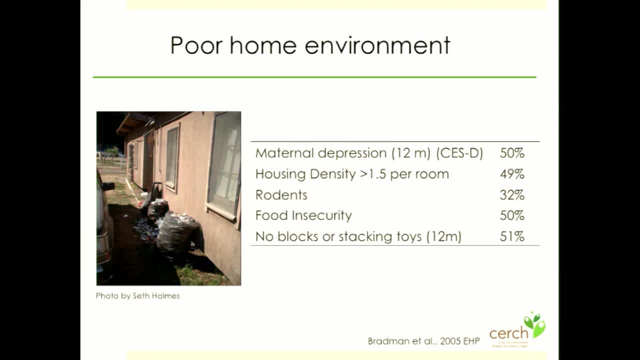 at whether a chemical is associated with a behavioral endpoint. Maternal depression is very, very high in this population. 50% of the women reached a level that was considered to be clinically notable on a scale of depression. The amount of housing density was extraordinarily. 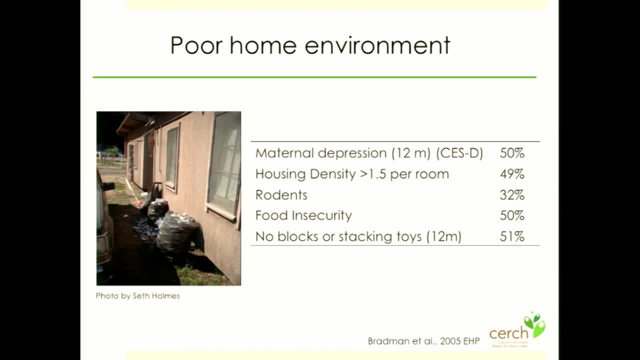 high in this population. It was not uncommon to see, in three bedrooms, three different families and then 12 farm workers sleeping on the floor in the living room. So the housing density is very, very high, much higher- 20 times higher than in the general US. 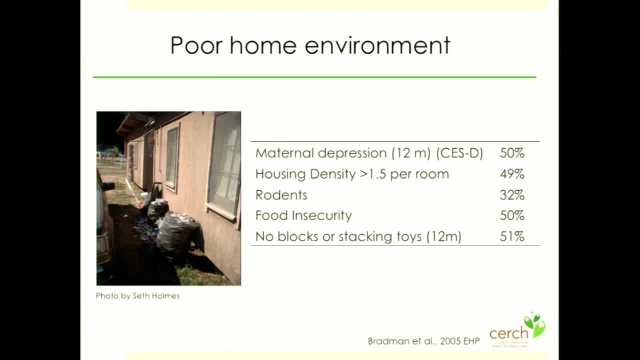 population. A third of the homes had rodents. Food insecurity is very high, ironically so that these people are farm workers, they have farm worker families and yet there are food insecure and many of them food insecure with hunger And when we went into the homes 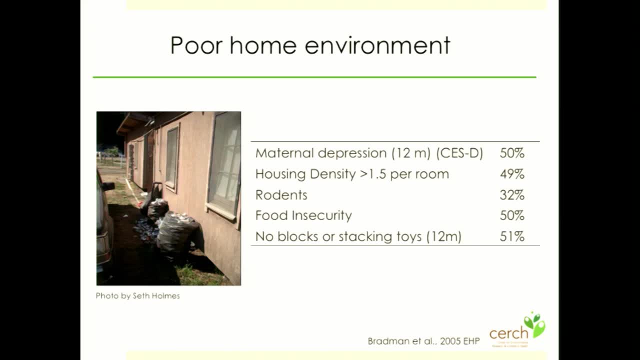 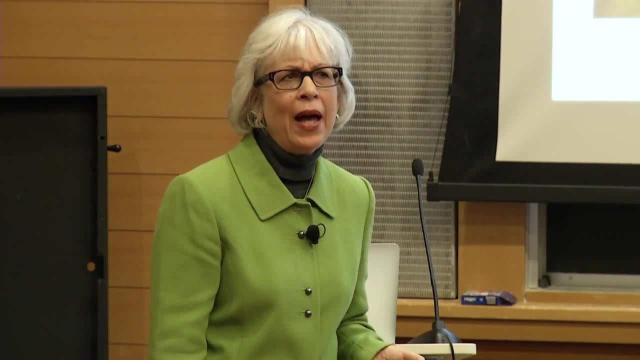 to look at. were there toys for the children? there were no stacking toys or blocks or anything educational, although most of the houses did have televisions and VCRs at the time. Now they're CD players. So going back to that experiment, 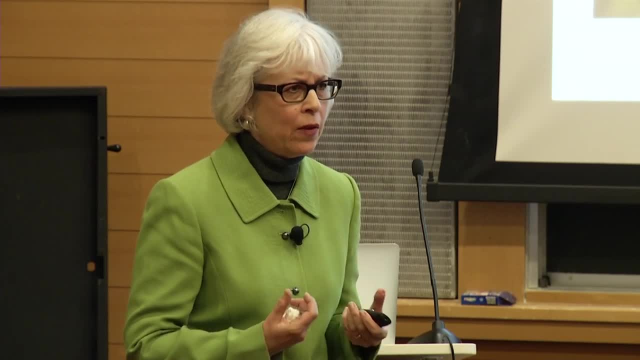 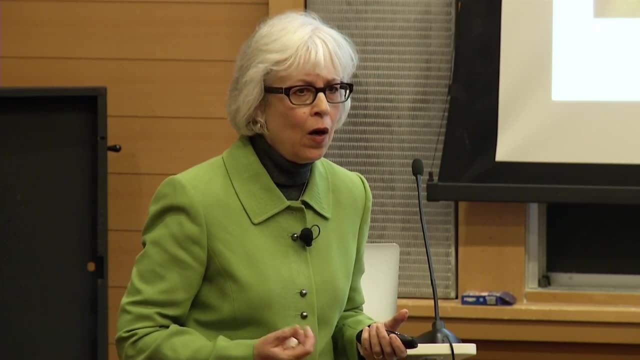 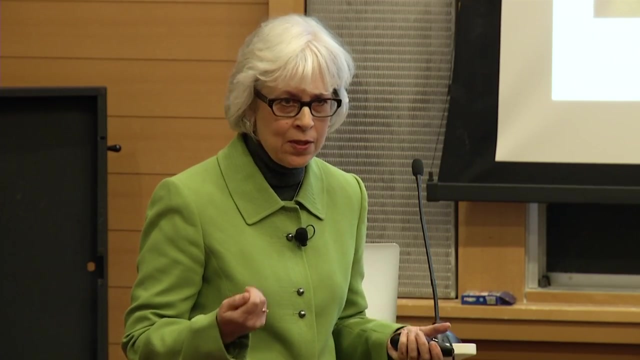 are we more? are some people more susceptible to the effects of organophosphate of pesticides in other people? If you and I are exposed to the same amount, are you just as likely as I am to show neurobehavioral problems, or are there differences? 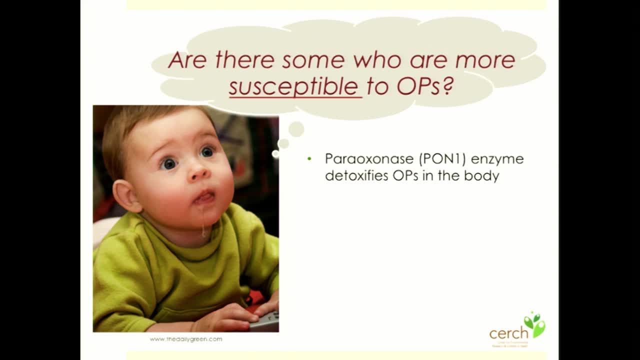 by different populations of people. We know that there is a group of genes called PON1 and that this cluster of genes is involved in coding an enzyme, peroxinase, that is important in detoxifying the organophosphates in the body. 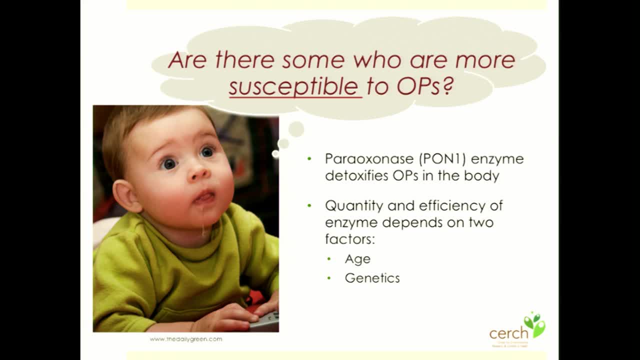 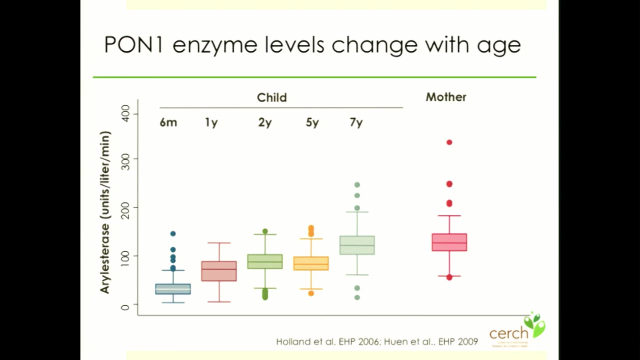 That the quantity and efficiency of the enzyme depends on two factors: the age of the person and their genetic makeup. At least these two factors, maybe more So let me show you some of the work that our center has done. When the children were six months: 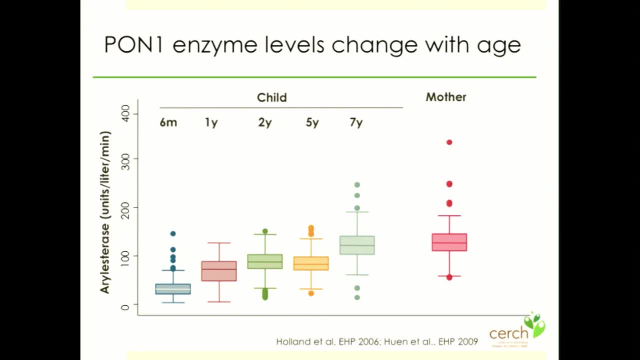 one year, two years, five years and seven years. we looked at the amount of enzyme that they had in their blood and we compared it to the amount of enzyme that the mother had in her blood. And what you see is that at six months, 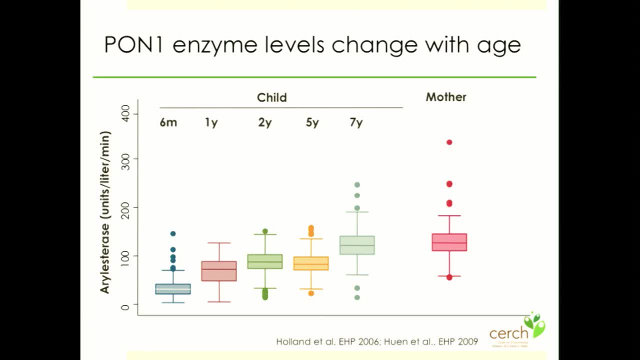 one year goes up two years, it goes up more, seven years. the children are approaching the maternal level of enzyme. It used to be thought that by two years of age a child had the same ability to detoxify a chemical as an adult did. 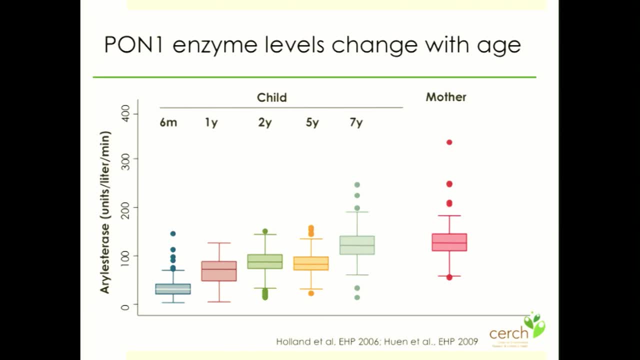 What this data is showing is that not until seven years of age, maybe even older- I think it was nine years- that we finally saw that they were really equivalent to the mother, that we see that children have adult levels of ability to detoxify these chemicals. 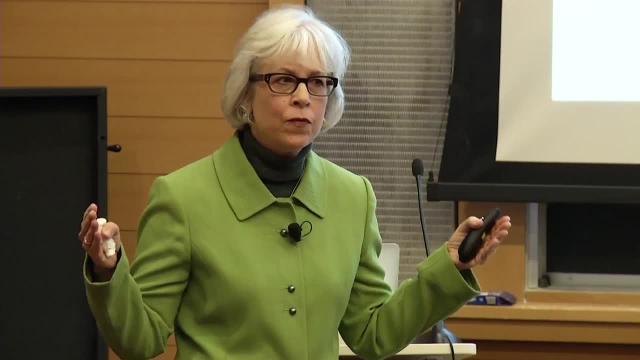 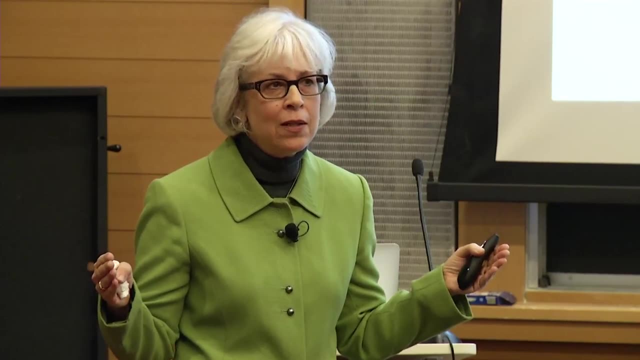 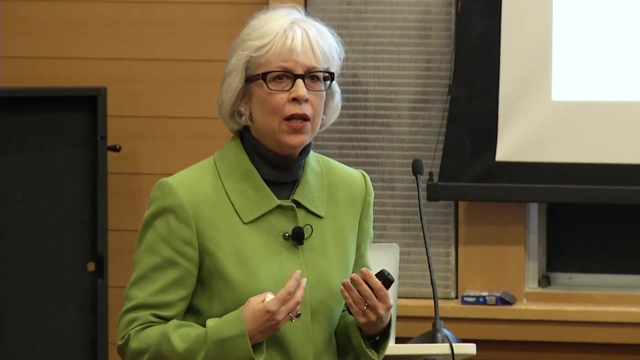 That means that the window of vulnerability of children is much, much wider than we ever thought. That means a child who is exposed two years old, three years old, four years old, doesn't have the same ability as those of us in this room to make those chemicals. 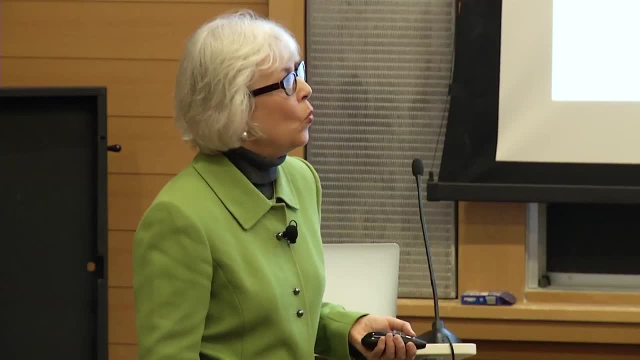 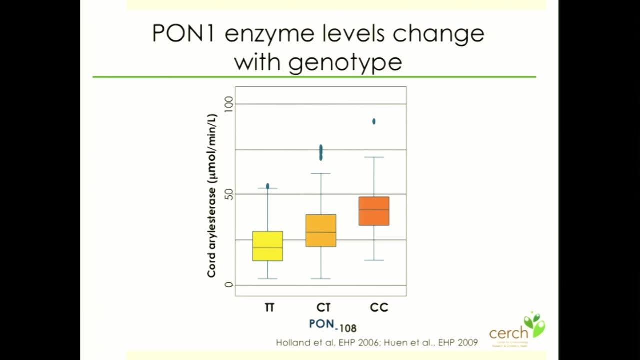 less toxic in their bodies. We all also know we genotyped all of the children in our study for this particular gene called PON108.. It's in the promoter area And we looked at the relationship of a child's genotype with how much of that enzyme. 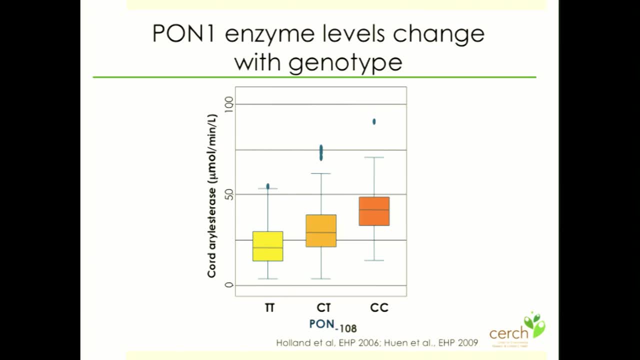 they had in their blood, And so if you have a different genotype you have different ability to detoxify these chemicals. So if you are a TT, you're going to be less fortunate because you have lower level of enzyme to detoxify those chemicals than if you have CC. 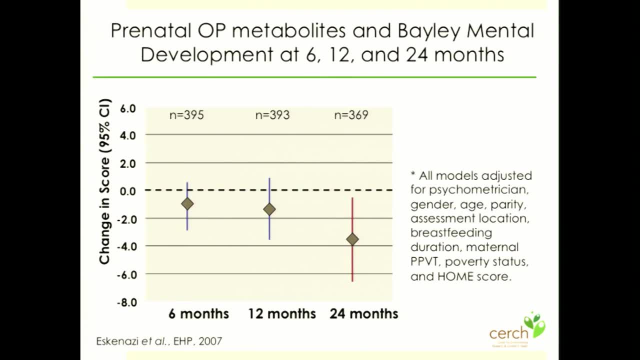 So that means if you and I are exposed to the same chemical, the same amount of chemical, but I have TT, does that make me more vulnerable to having a neurobehavioral problem than you? Am I more likely to be affected by that same level of exposure? 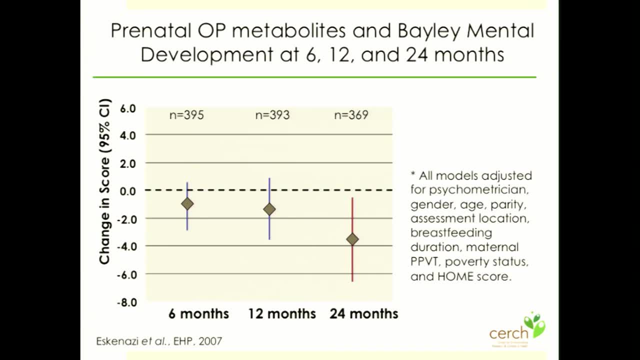 So remember, earlier I showed you this exact association. I showed you that there was nothing at 6 months in terms of the prenatal OP metabolites and mental development at 6,, 12 and 24.. Nothing at 12 months, But at 24 months. 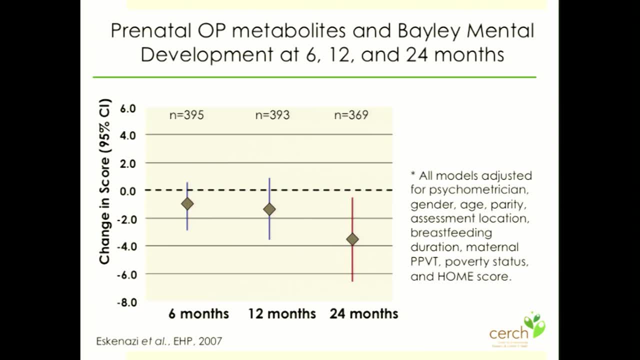 there was no significance. Now, what happens if we look at the relationship of these metabolites and mental development in children at 24 months? but now dividing up the children based on their genetic makeup? Okay, So in other words, what would you predict here? 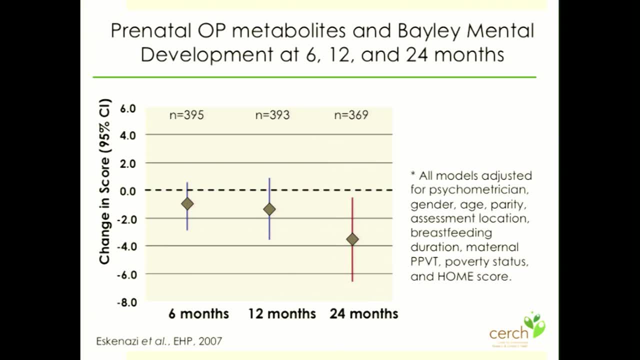 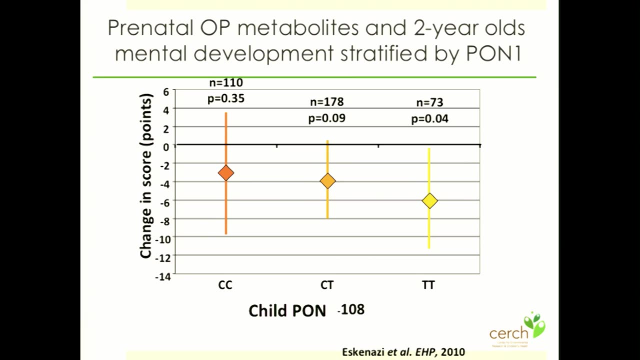 That the children with TT had the lowest level of enzyme, therefore the most vulnerable to be affected by the same levels of exposure, And we found evidence of that. The study gets very small when you divide up the group into three, But here are the kids with CC. 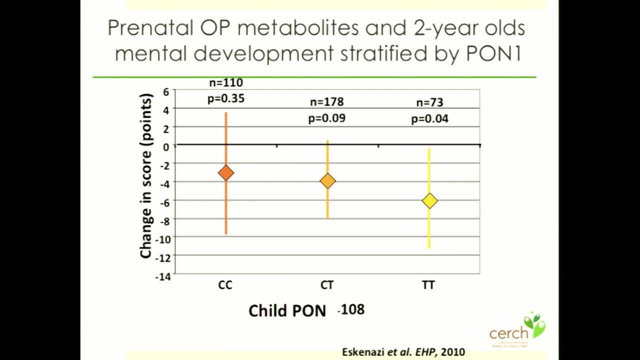 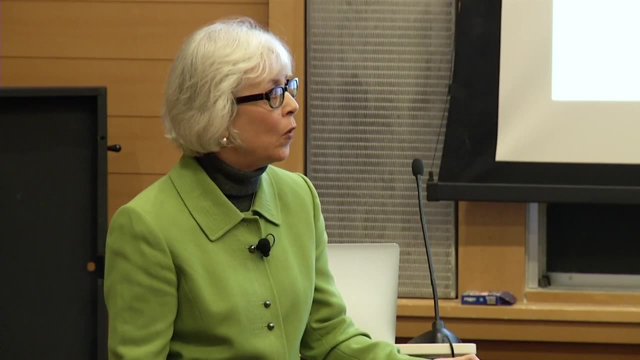 here are the kids with CT. here are the kids with TT. Now, this is the same thing I showed you before: The two year mental development in relationship to the DAPs in the group. now, by their genotype, We see not much going on in the children that had. 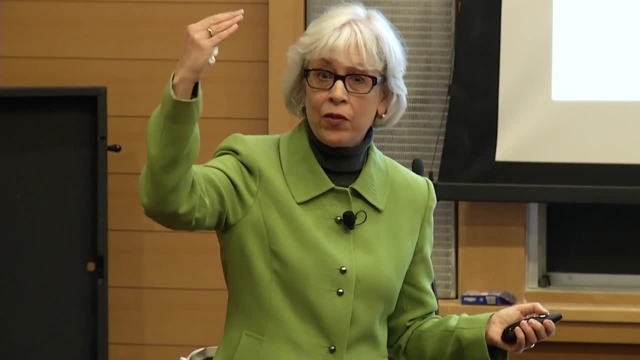 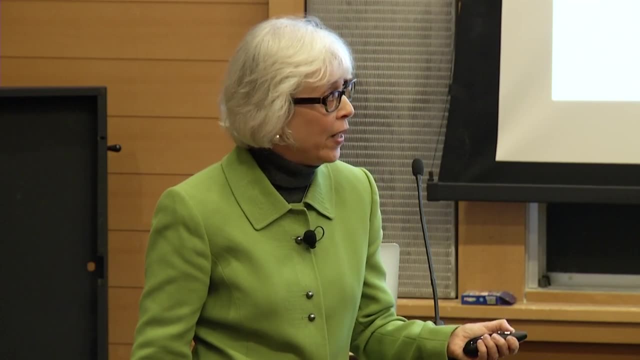 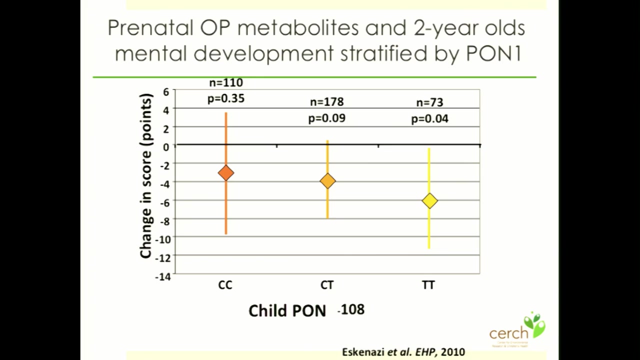 that genotype that is related to higher levels of enzyme. So there's little effect in that group. There is slightly greater association in the children that are heterogeneous for that gene And in the children that had the lowest level they had TT as their genotype. 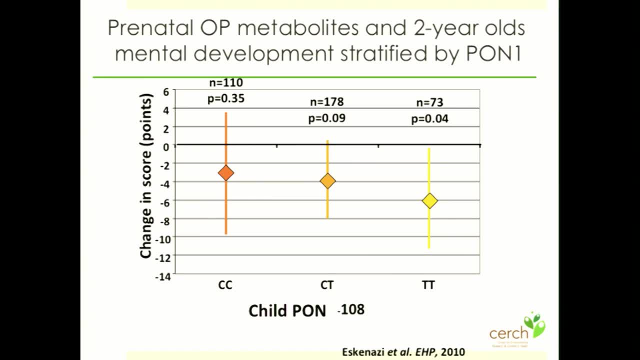 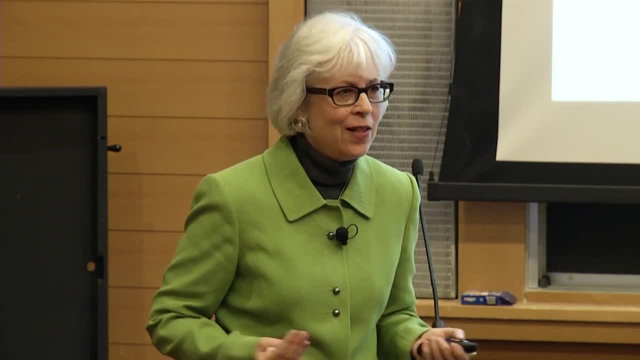 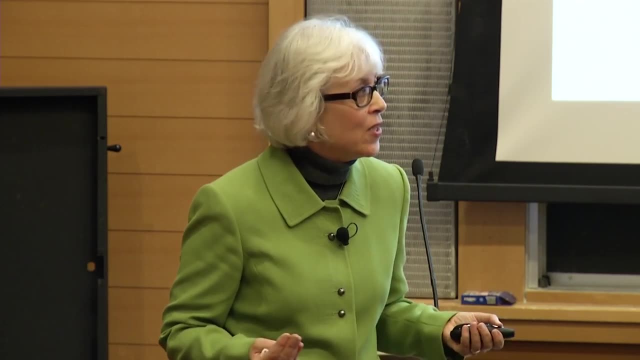 That's where we see the statistical association. This suggests that not everybody is created equal, That not all of us who are exposed to the same chemical are equally susceptible. But this kind of study needs to be replicated, needs to have multiple studies looking at the same thing. 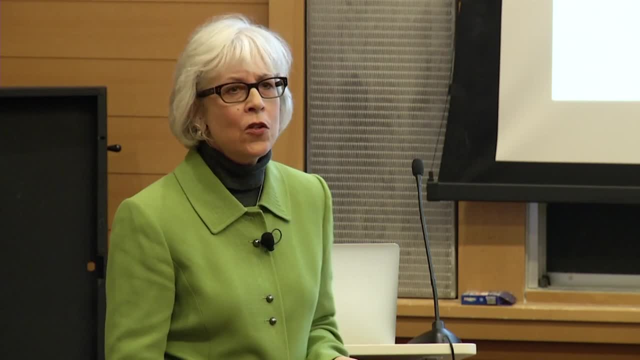 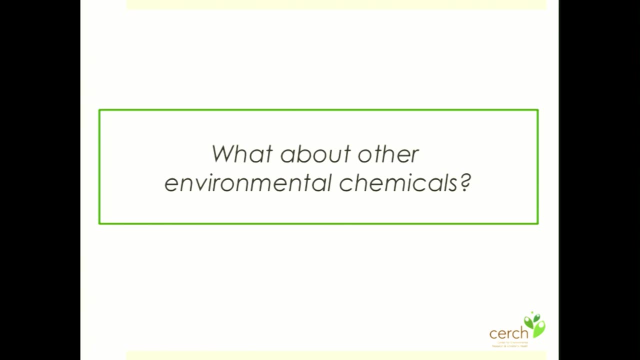 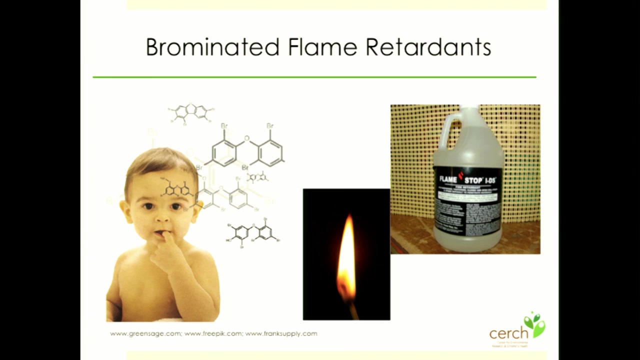 to show that there truly are true associations. What about other environmental chemicals Today? I don't know how many of you read the Chronicle, but we reported on brominated flame retardants in relationship to IQ and neurocognitive development in the children. And I'm going to be talking. 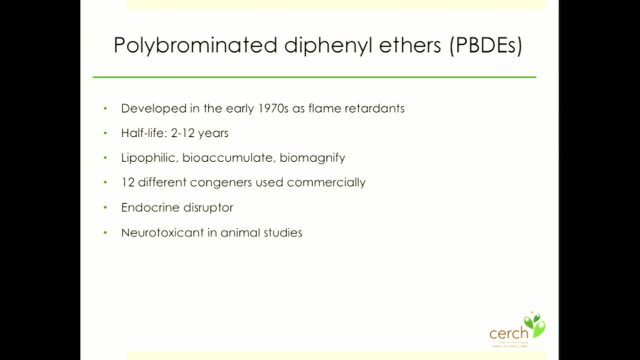 about those results today. So polybrominated diphenyl ethers were developed in the early 1970s as flame retardants. They have a very long half-life in the body and in the environment, unlike the organophosphate pesticides. The half-life 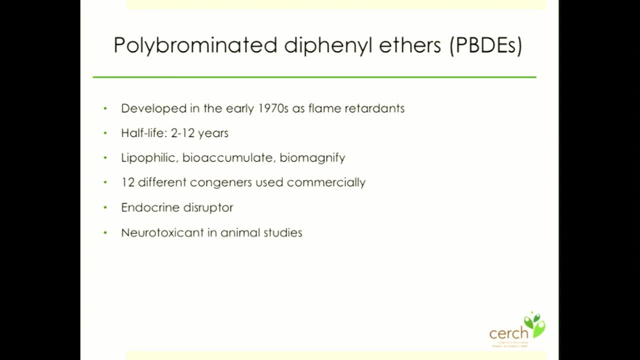 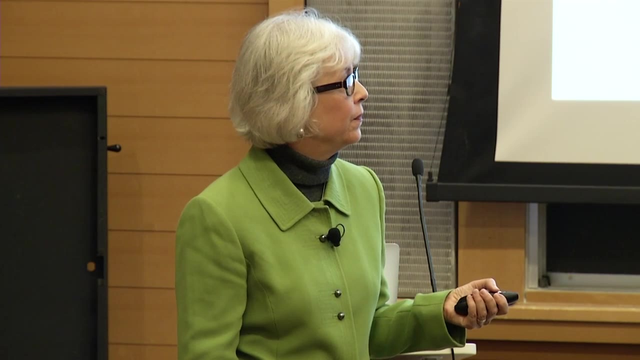 meaning that it takes about 2 to 12 years for half of it to go away is very long. These chemicals are lipophilic, which means they accumulate in the fat, They bioaccumulate in your body and they biomagnify. They're endocrine disrupting. 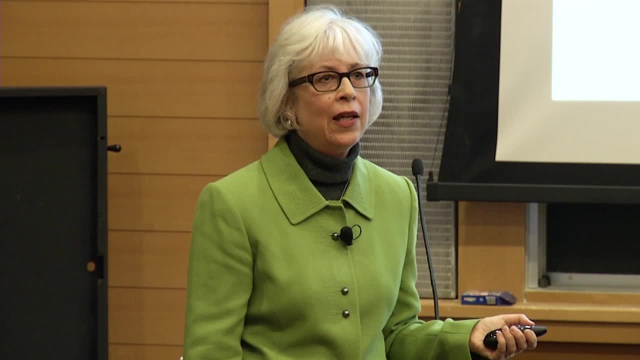 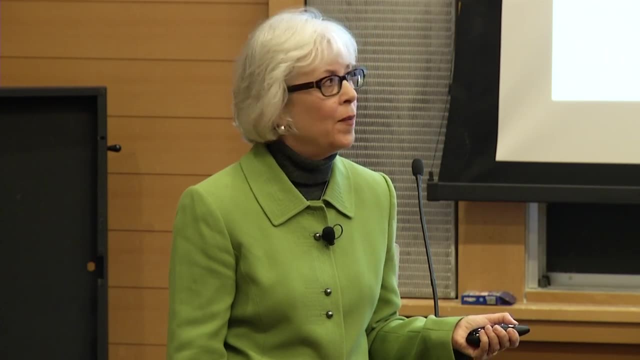 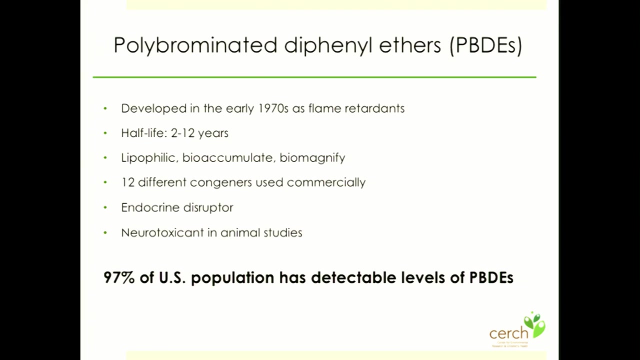 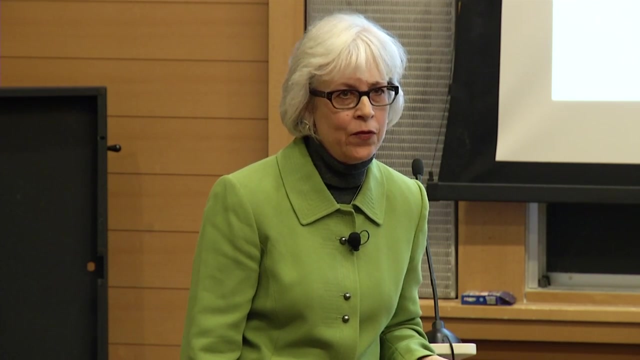 chemicals, meaning they can look like hormones, They can alter hormones And so we have concerns about them because they are hormonally active In animal studies. they are neurotoxic, meaning they affect the nervous system of animals And 97 percent of the US population. 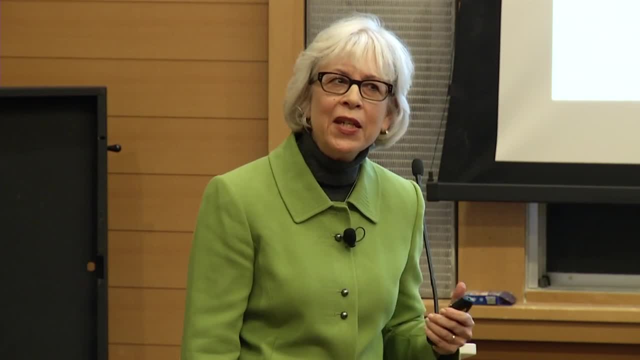 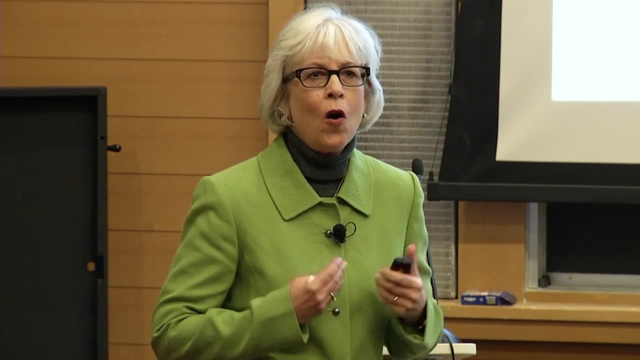 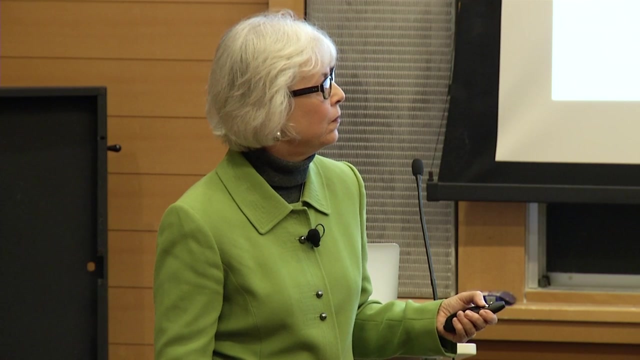 have flame retardants in their blood. When something is detected, it doesn't necessarily mean that it's bad. So what we need to understand is: are these detectable levels? are these levels associated with health effects? What are the sources of PBDE exposure? 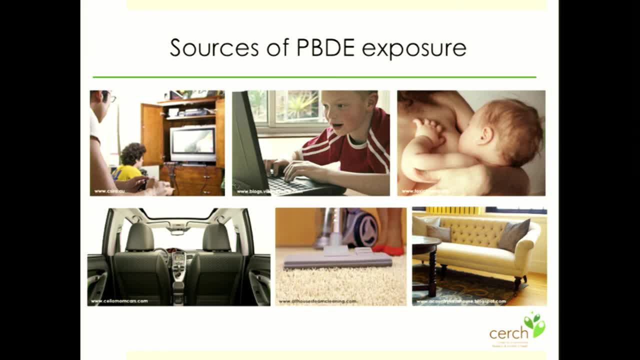 Well, you're sitting on one right now. The foam in these chairs, I'm sure probably a lot of you have seen, But the foam in couches, the dust on your floors, in your cars, in your computers and to the baby, it's in the mother's breast milk. 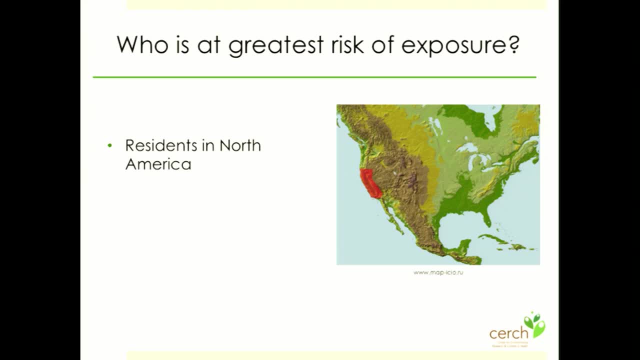 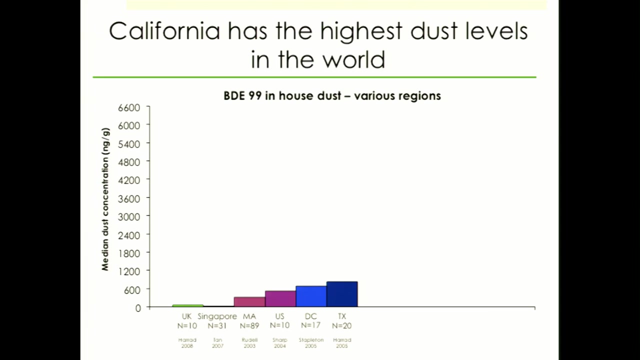 Who's at highest risk of exposure? Residents in North America, Particularly California. There's a dubious distinction of having the highest levels in the world, With few exceptions, So let me show you exactly what I mean. These are dust levels of one particular. 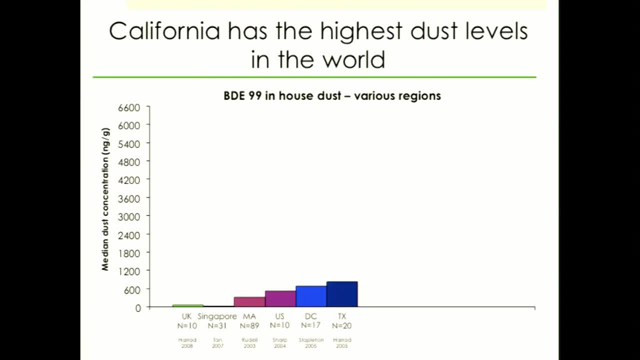 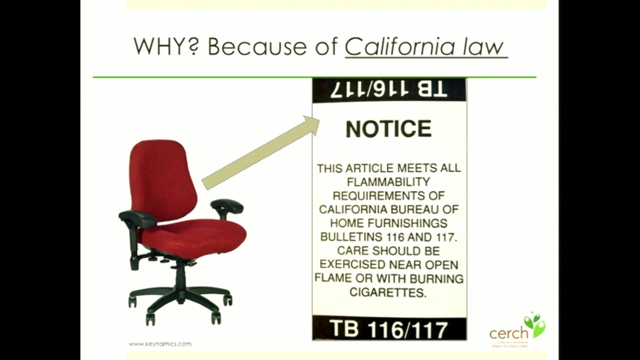 congener of flame retardants and these are dust levels in the UK, Singapore, Massachusetts, the general US population, District of Columbia, Texas, California, Salinas. Why? Because of California's flammability standard. Remember that tag. 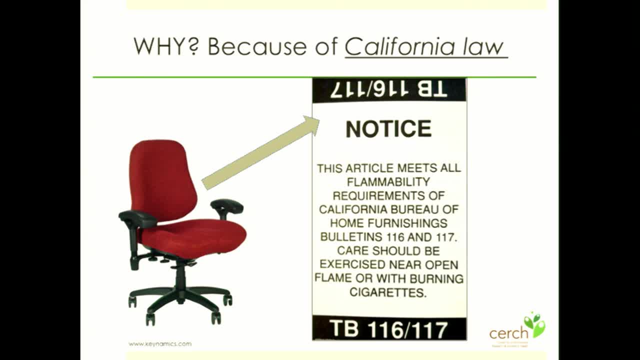 that hangs down that you never know whether you're supposed to remove it or not. It's because of the flammability requirement of the California Bureau of Fire Regulation. Many manufacturers added these flame retardants to especially foam and the padding under carpets, and to computers. 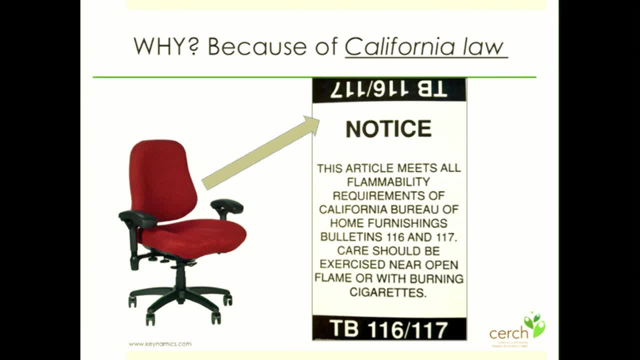 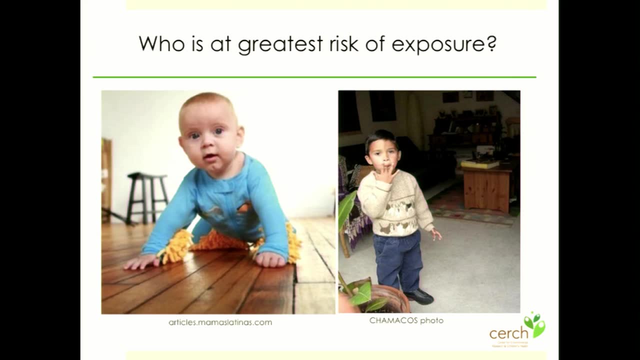 and everything else to prevent fire. However, the flammability standard is really not clear, whether it actually saves lives from fire, which I'll talk about a little bit later. So let's talk about the risk of exposure to these PBDEs. 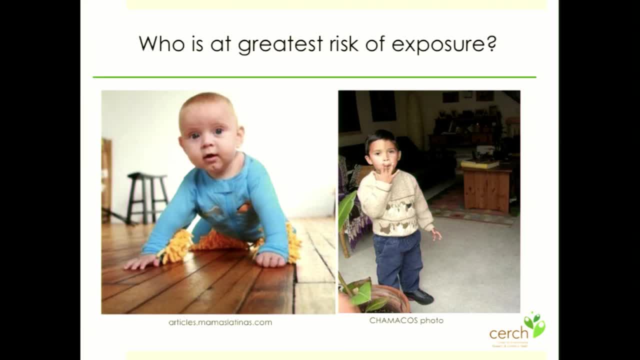 or these flame retardants, Children. I love this particular picture because this shows you how much we already know that children pick up a lot of dust. This company actually invented a little coverall with little dusters on the coverall, So you might as well get your house cleaned. 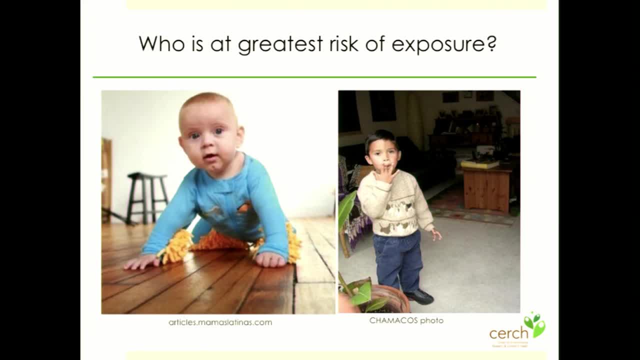 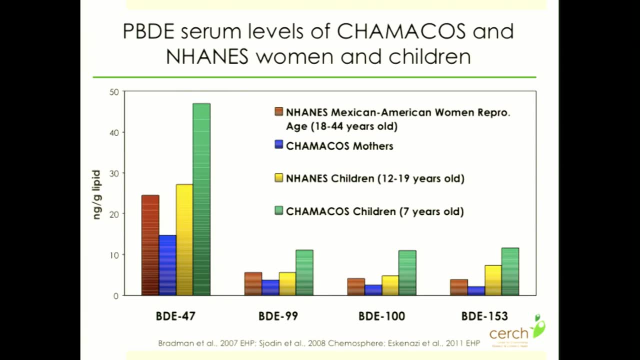 and they also put their hands in their mouth a lot leading to higher levels of exposure. And this is the PBD serum levels of the Chamacos cohort in relationship to the general US population. So let me walk you through this. 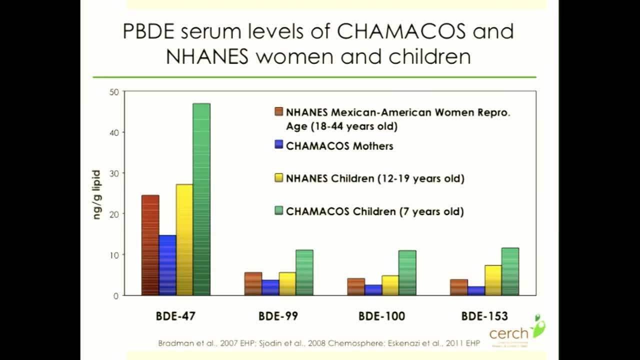 This is the NHANES. This is the National Health and Examination Survey. in red, These are four different congeners, the most common congeners, of something called the Penta PBDEs. This red is higher than in the Chamacos women. 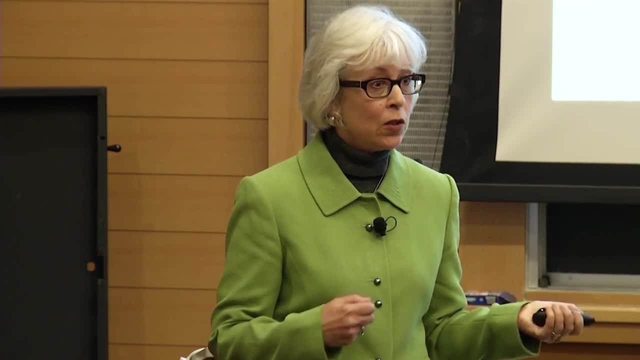 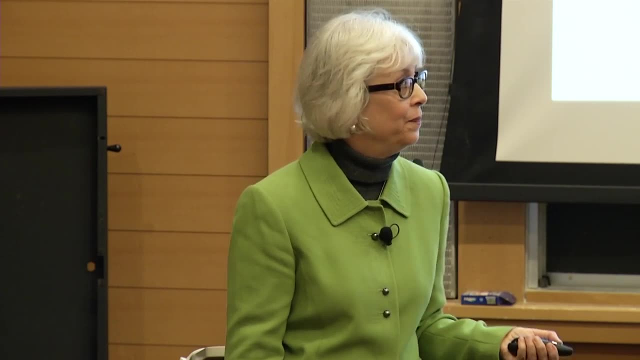 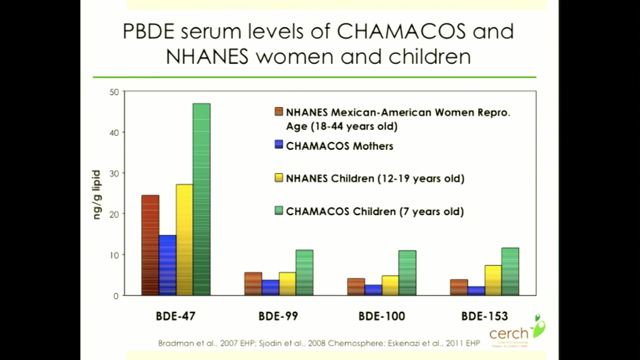 for all congeners. So the Chamacos women actually had lower levels of PBDEs in their blood than the general US population. These are the NHANES children. These are the Chamacos children. So their mothers didn't have. 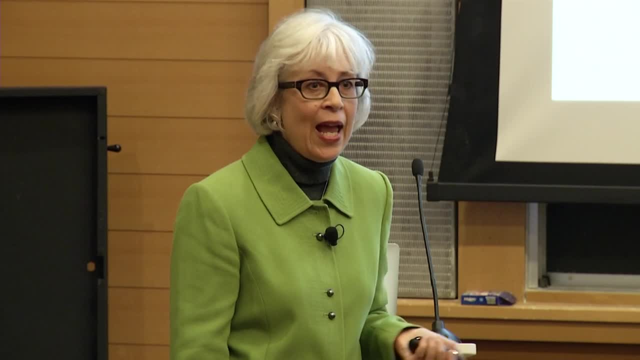 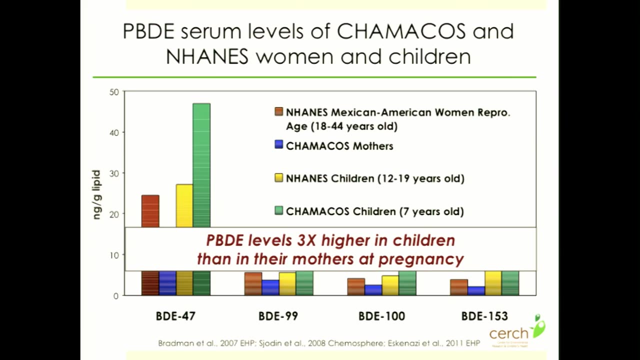 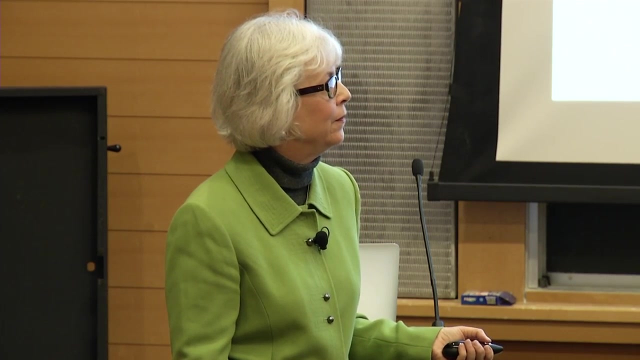 particularly high levels. but the children in Chamacos had incredibly high levels And you may ask why, Which I'll tell you in a second. The children's levels were three times higher than their mother's levels- Three times higher. So we didn't understand at first. 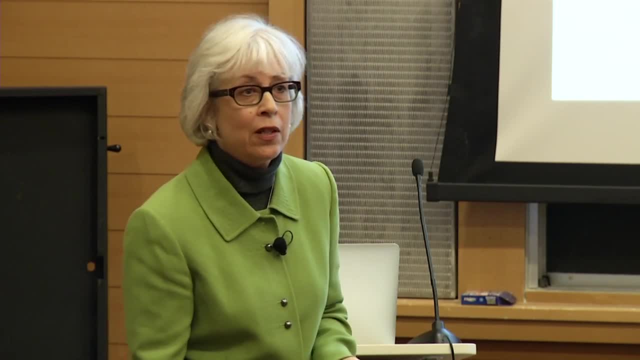 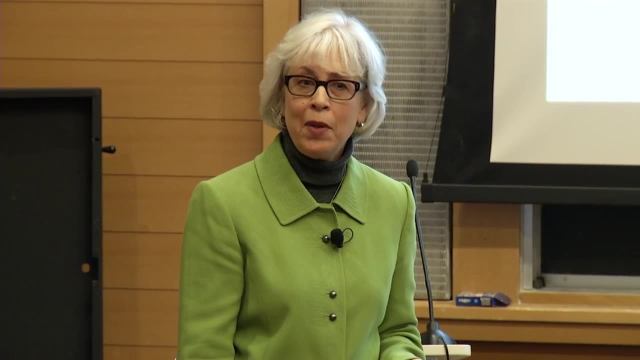 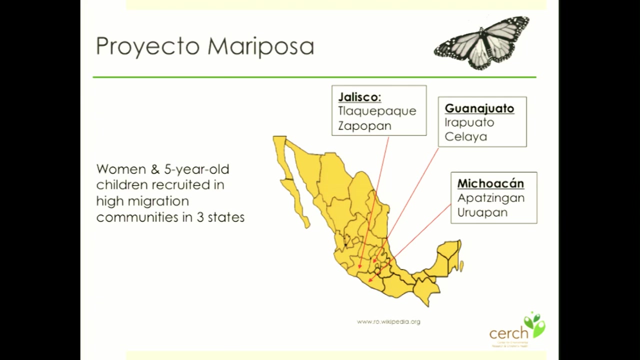 why our children had higher levels than their mothers. but then we thought maybe it had to do with the fact that the Chamacos women- 50% of them- were born in Mexico And half of them- sorry, 85%- were born in Mexico. 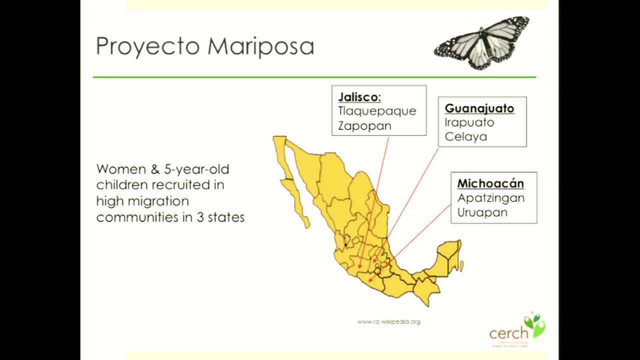 half of them had lived in the United States for less than five years. So we went to Mexico and we said let's do a study, collecting blood samples from the communities where the Chamacos women came from. So we went back to the sending communities. 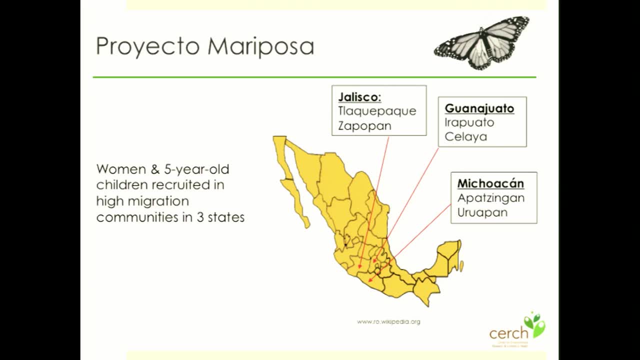 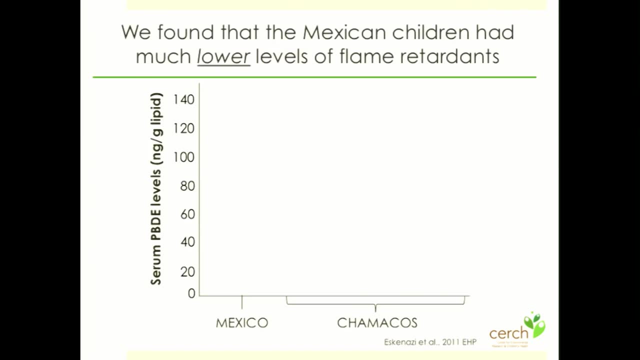 in those communities in Proyecto Mariposa, and we analyzed the Mexican kid bloods against the Chamacos bloods. Okay, we found that the Mexican children had much lower levels. This is the levels of the children in Chamacos whose mothers had been: in the United States for less than five years. All the children were American. all the children were born in the United States. This is, those children whose mothers were less than five years in the United States. if the mothers lived five to 15 years in the United States. 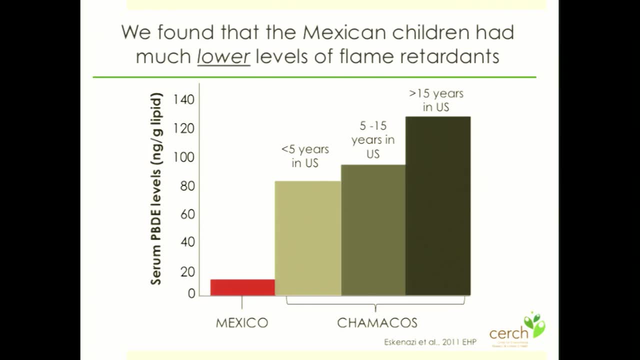 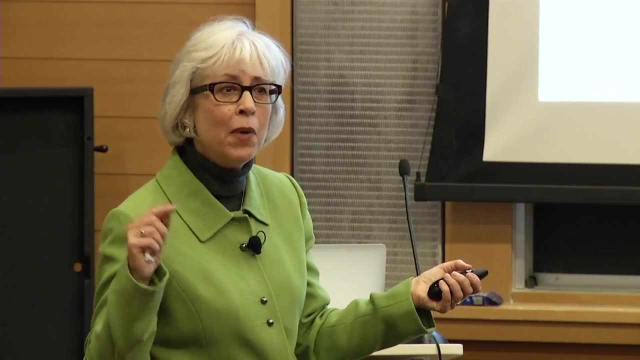 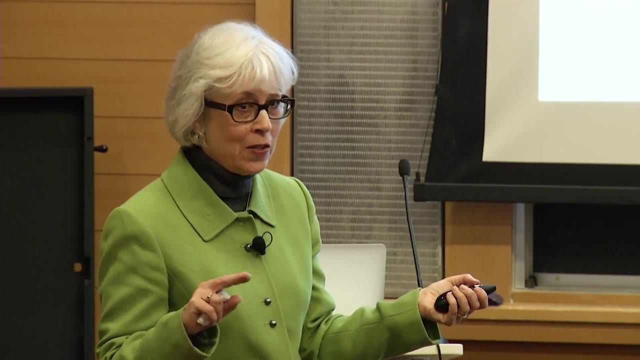 and if the mother lives greater than 15 years in the United States, So that we saw a higher level in the child based on how long their mother had lived in the United States. And remember they're being breastfed. Almost every child in our study was breastfed. 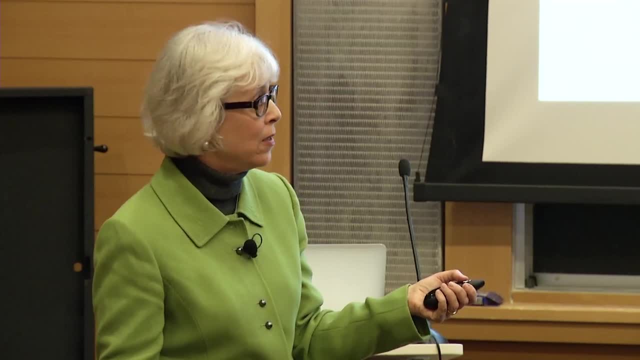 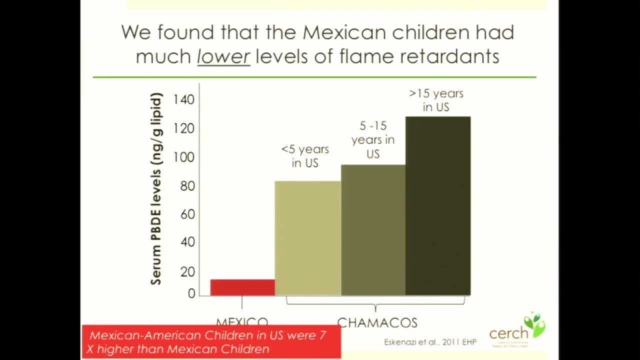 and breast milk is a major source of exposure to these kids, as well as the dust in their homes. The Mexican American children in the United States were seven times higher than the Mexican children in terms of their blood levels of PBDEs. But it's not just. 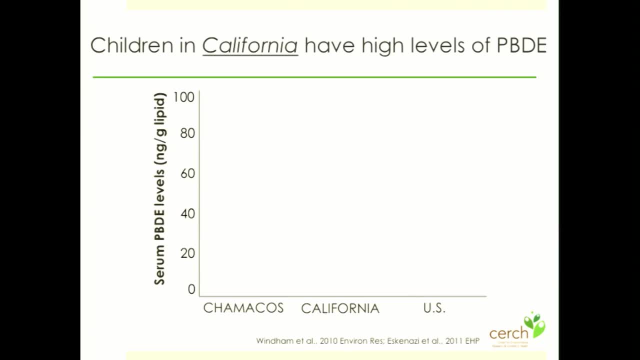 the Chamacos children. It's not just that our children had high levels. Those are the Chamacos children. This is a study done out of Kaiser California children and that's the general US population of children, So it's not just. 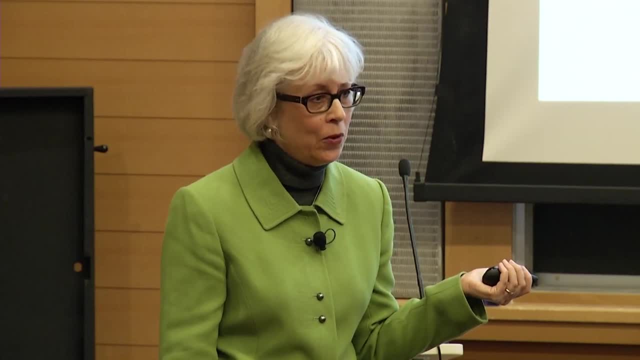 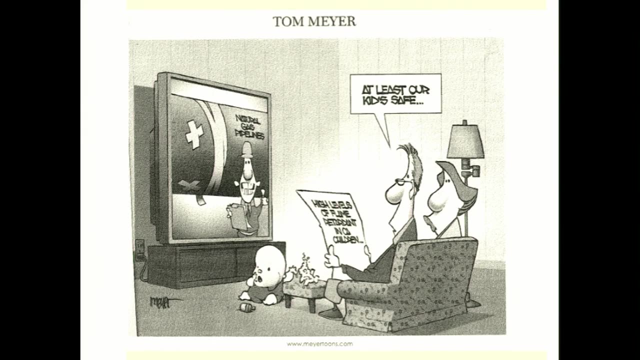 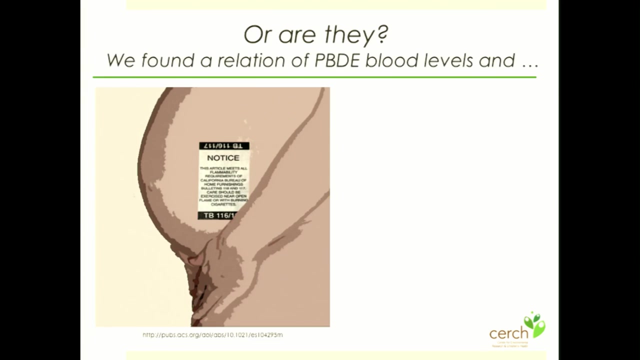 the Chamacos children. It's children living in California, It's our children. So at least our children are safe. High levels of flame retardants. Our children are safe from fire, Or are they? Are they safe? We have found a relationship. 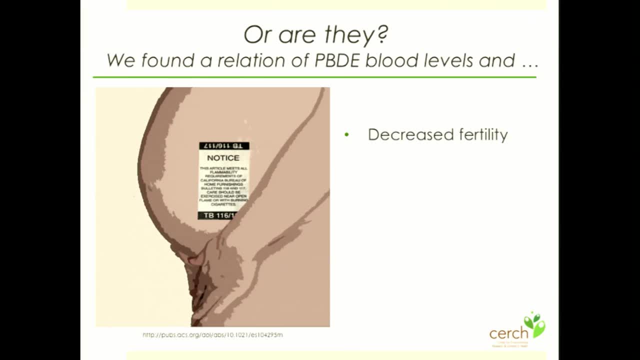 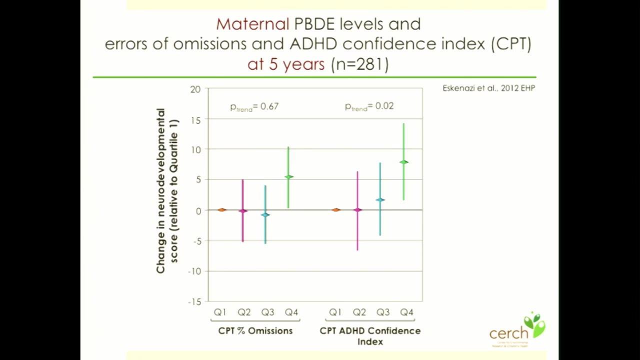 of the PBDE blood levels and decreased fertility in the women, lowered birth weight in the children, alteration in maternal thyroid hormone and now neurodevelopment. So now I'm going to walk you through the studies that were published today And environmental health perspectives. 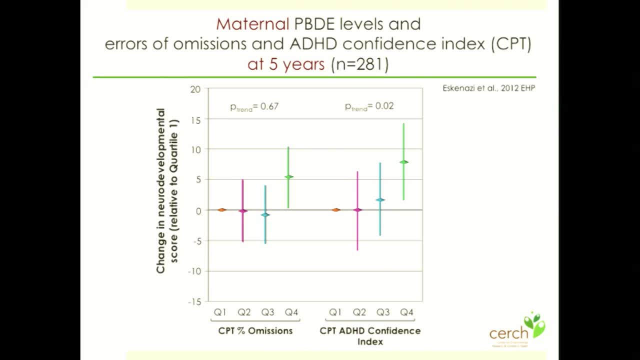 And first let's talk about the maternal PBDE levels. And we did a test called the continuous performance test. This is a test of child attention, Every time a child sees a particular stimuli on a computer screen, let's say a soccer ball. 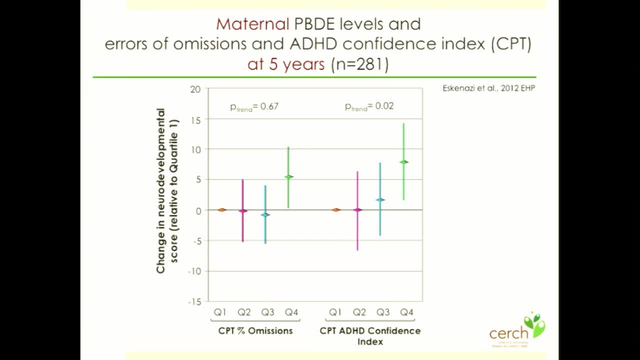 they're supposed to press the space bar, But when they see a camera, they're not supposed to press the space bar. They're supposed to look at the child's attention. errors of omission: meaning they forgot to press when they should have pressed. 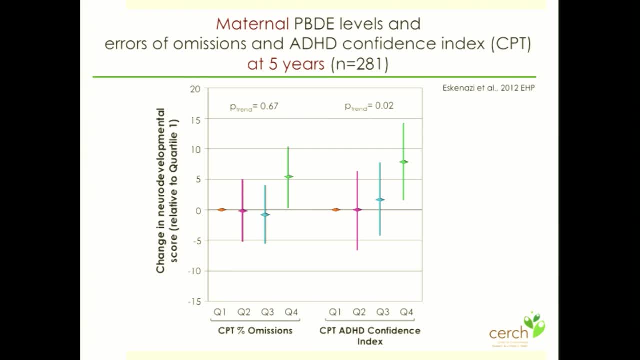 and errors of commission. The kid is constantly pressing when they shouldn't be pressing And what we find is that here is again the change in neurodevelopmental score. This is that no effect line. We have divided now the children into four levels of PBDE, based on. 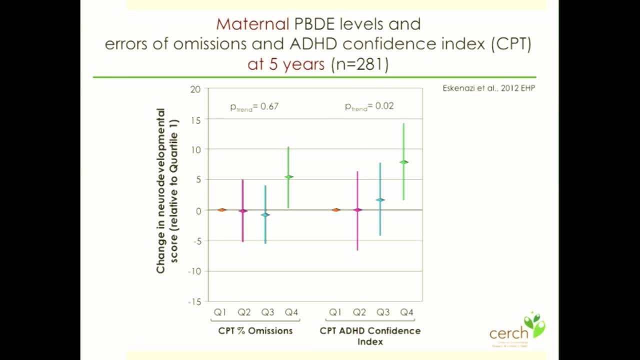 the mother's level. So this is the lowest 25%, the next 25%, the next 25% and the last 25%, And you can see that the children whose mothers had the highest levels of exposure had statistically significantly more errors of omission. 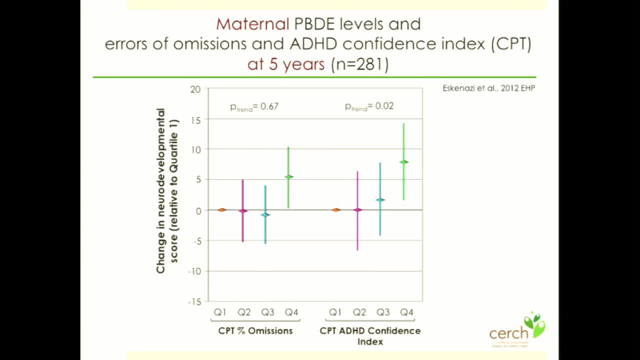 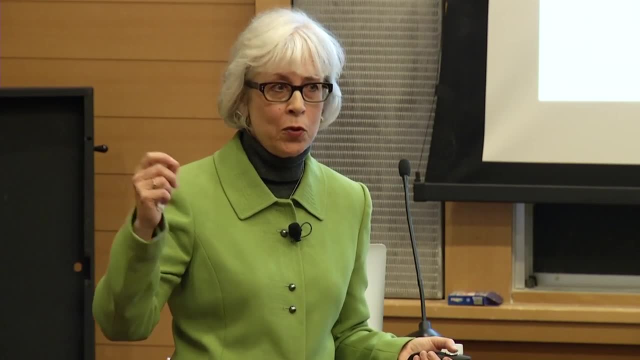 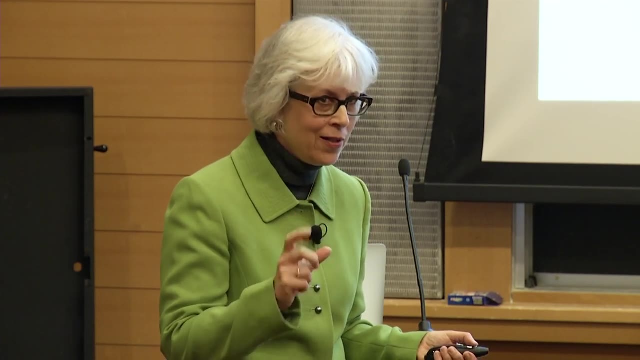 They forgot to press the bar when they were supposed to. And on this test they give you a confidence index on how confident you would be that this child has ADHD. But it's not a clinical examination. So I'm not trying to say this is a clinical evaluation. 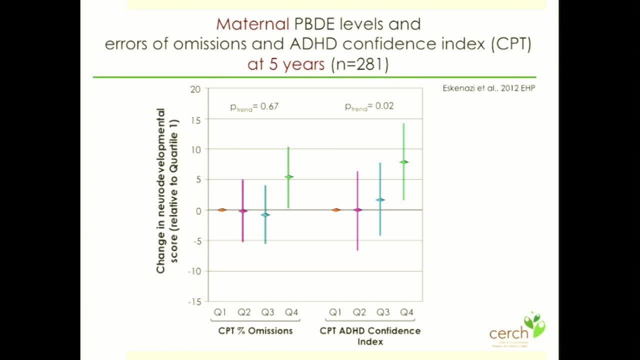 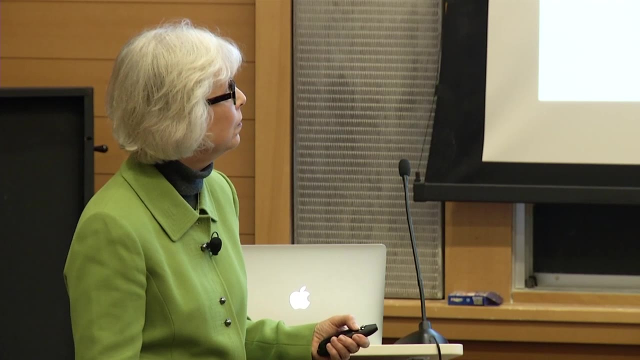 Again, those kids whose mothers had the highest quartile of PBDE levels during the pregnancy. the kids were more likely to have for us to be confident that they had ADHD. We also remember asked not only the mothers, because mothers aren't really. 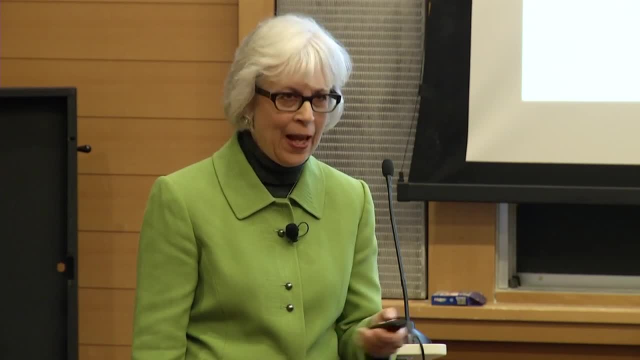 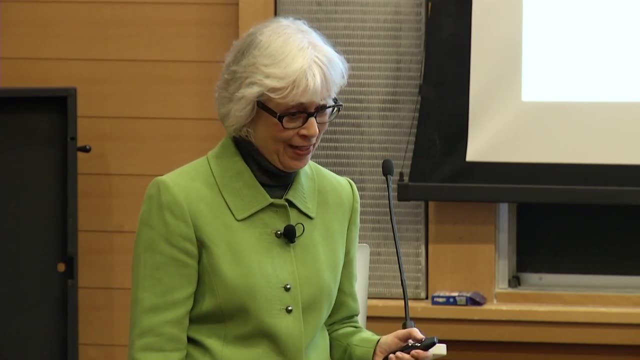 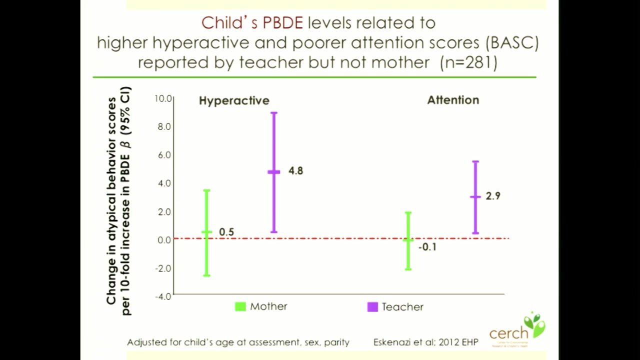 good reporters, but we also asked the teachers, And maternal report and teacher report aren't really very correlated. Is that a surprise? So if you look at the child's PBDE levels, remember I told you that the child's PBDE levels 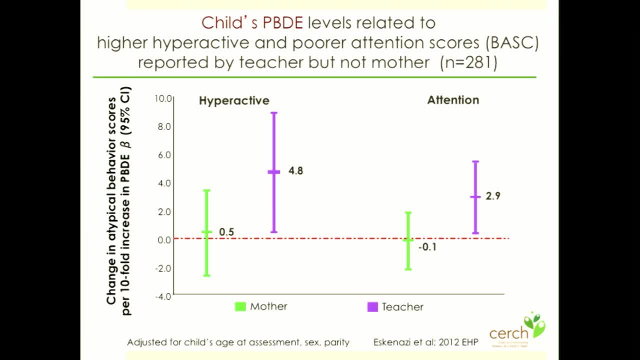 are three times higher than the mother's. We see a relationship with hyperactivity and attention on something called the BASC, which is another test that looks at behavior. It's based on maternal report or teacher report And we see that children who have higher levels 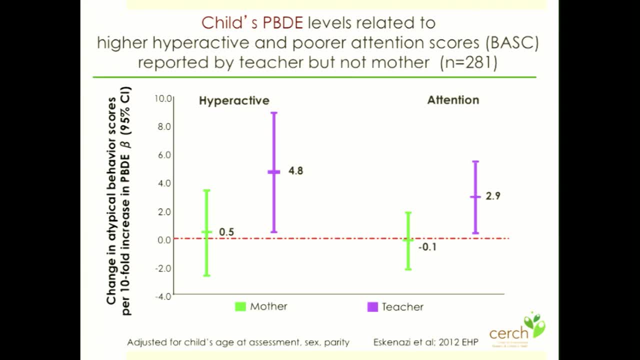 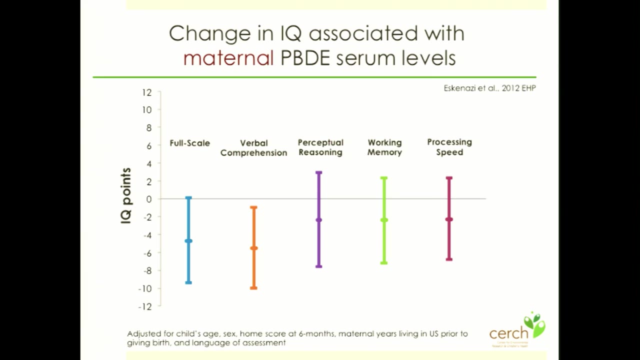 of exposure to these PBDEs are more likely to be reported by their teacher and hyperactivity, But not by their mother. Let's turn now to IQ. This is the IQ points. This is the change in IQ points. This is the no effect line again. 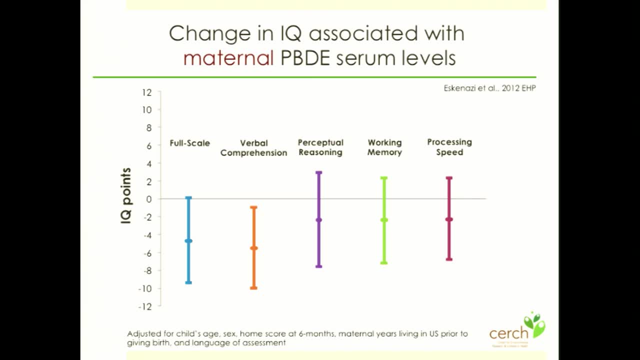 This is now looking at maternal PBDE levels. We see a statistically significant decrease. Notice, first of all, that all of them are below that line, showing in the direction that there are more deficits associated with the PBDE exposure, But only statistically significant associations. 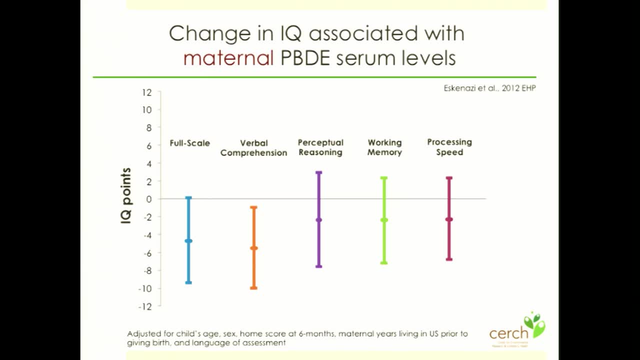 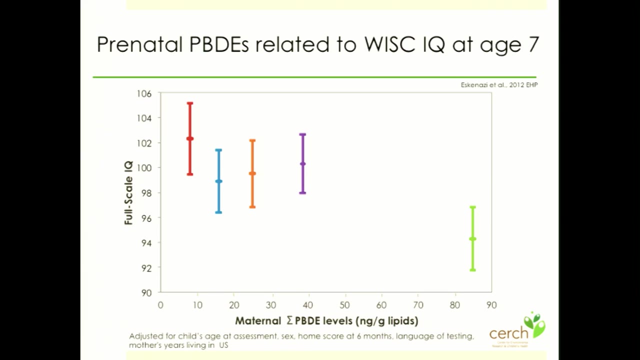 with the maternal PBDE, exposure and verbal comprehension and borderline for full-scale IQ. And again, these four comprise this. So another way of looking at this- I've showed you something similar before- is you divide the group into five quintiles. So lowest 20%. 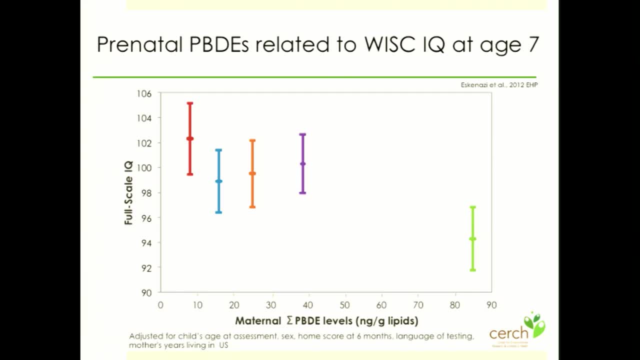 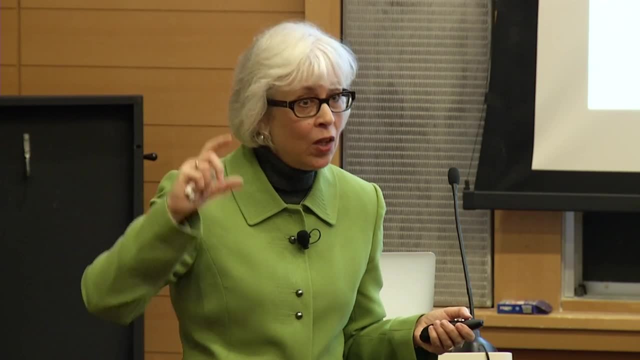 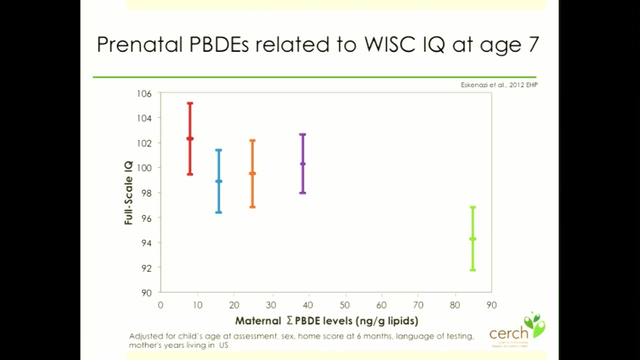 next 20%, next 20%, next 20%. And we're looking now at the mother's PBDE levels which, remember, are a little bit lower than the general US population. So this is not just about California kids now. 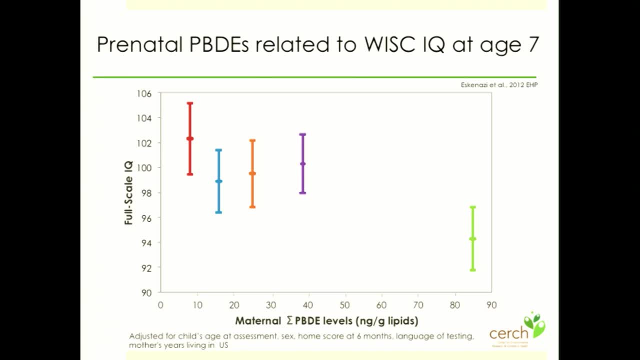 And we see that there is a difference of about eight IQ points, which is little more than between those kids whose mothers had the lowest levels of PBDE in their blood versus those children of those mothers with the highest PBDE in their blood. And 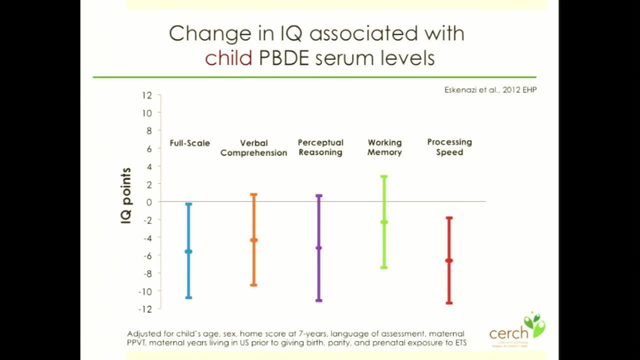 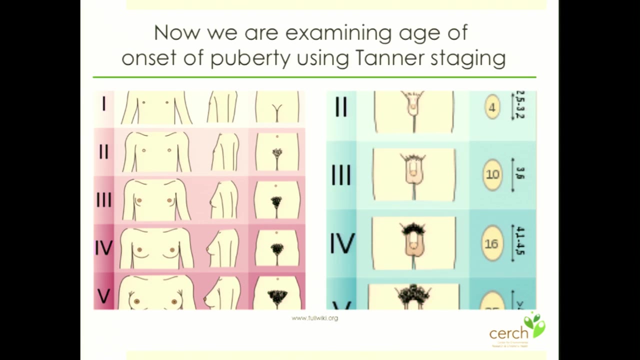 if you look at the change in IQ associated with the child's levels, you see even lower, more differences associated with the child's levels. So now we are following up the children. I've only showed you their results at age five and age seven. 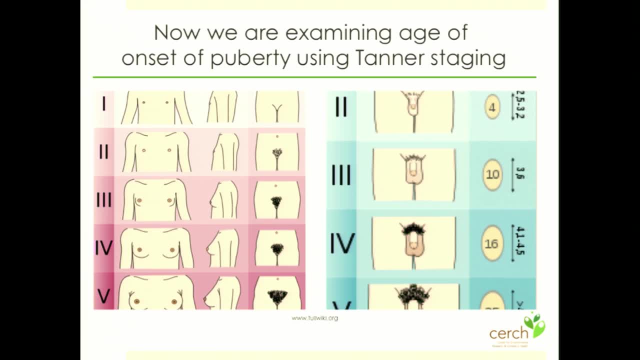 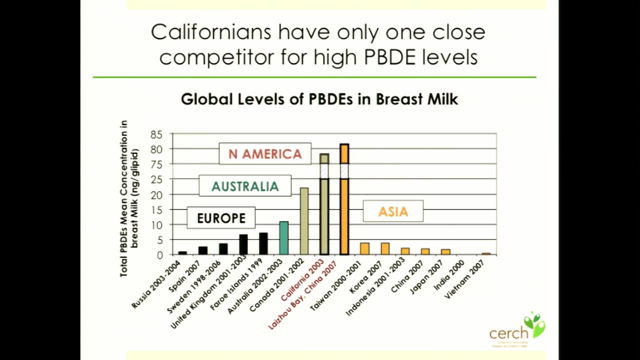 We're now following these children and they're now 12 years of age. So how does their neurocognitive functioning change with puberty? We'll be able to tell you more about that in the future. So Californians have only one close competitor for high PBDE levels. 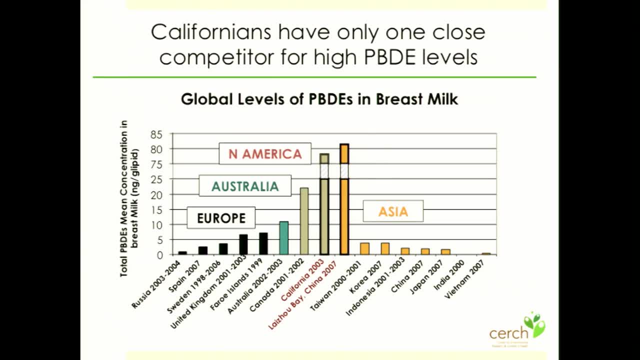 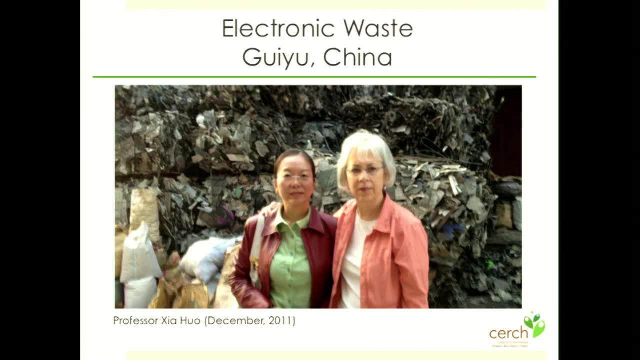 And those are people from China And this is my picture from- excuse me for saying this- Guoyu, China, where I went to see where those computers are winding up. Our computers are winding up in an electronic waste dump in China. 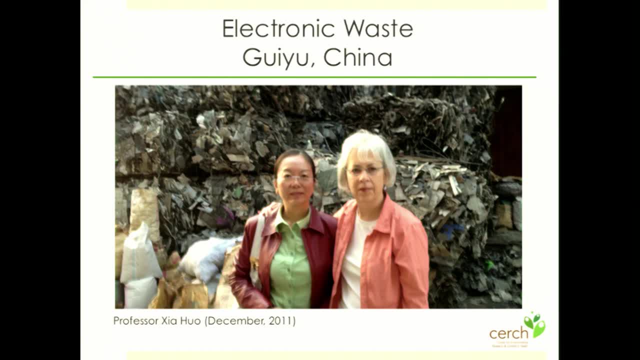 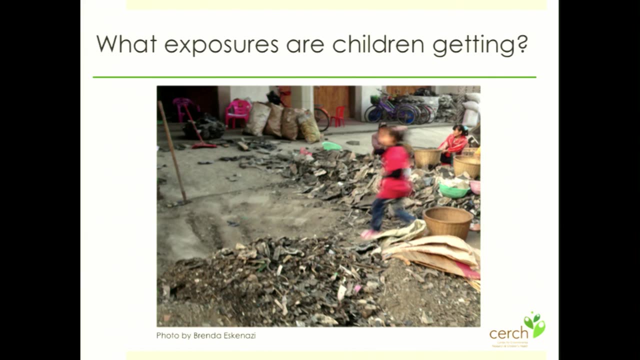 And someone is picking out little pieces of important recyclable residues that can be used in future electronics. But what exposures are the children getting? We are exporting those flame retardants to China And right now there are a bunch of studies that are going on. 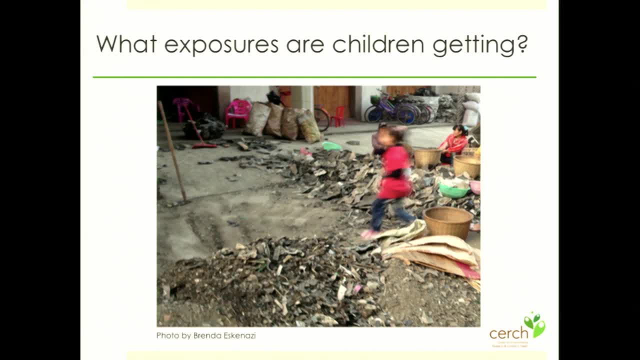 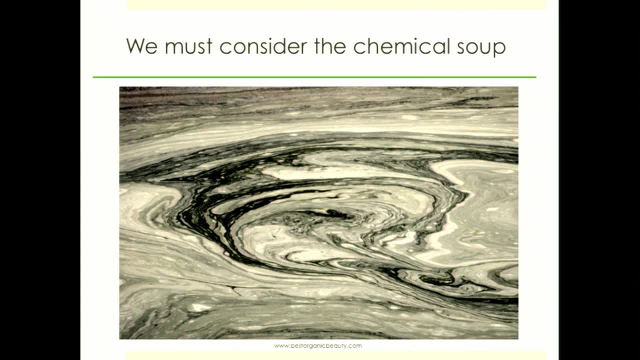 looking at a different class of PBDEs in relationship to the neurocognitive development of those children in China. You can't just look at PBDEs or organophosphates and think you've got the whole picture of what people are exposed to. 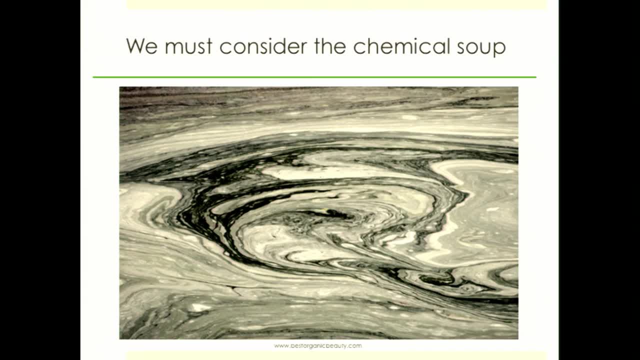 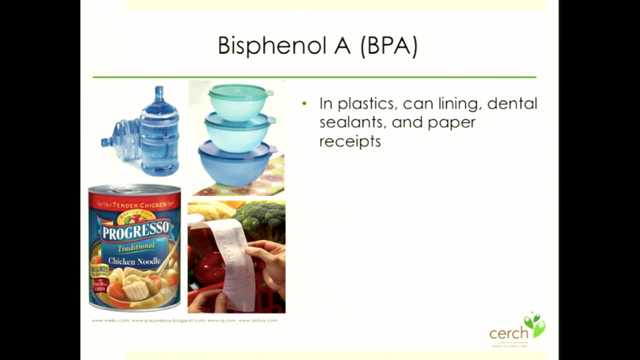 We live in a chemical soup And somehow, statistically, we need to consider that when we're looking at the relationship of one exposure to an outcome. We are now studying bisphenol A. It's in plastics, can linings, dental sealants and 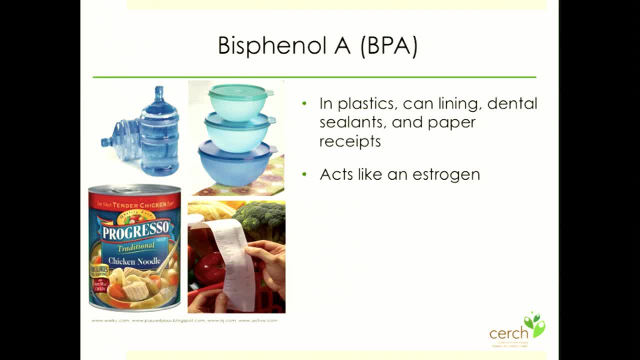 paper receipts, It acts like an estrogen. There are animal studies which have shown a relationship with obesity, puberty and neurobehavioral development. It's detected in 93% of Americans And Chimacos will be the first study looking at in utero exposure. 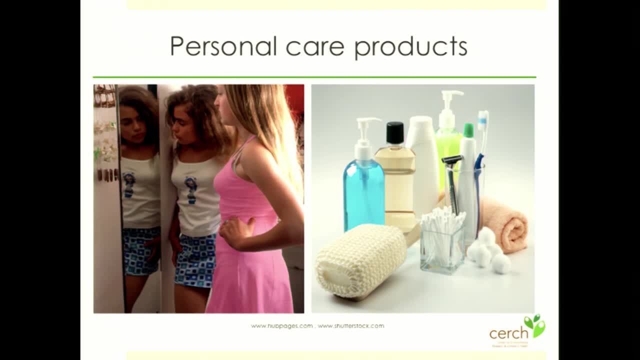 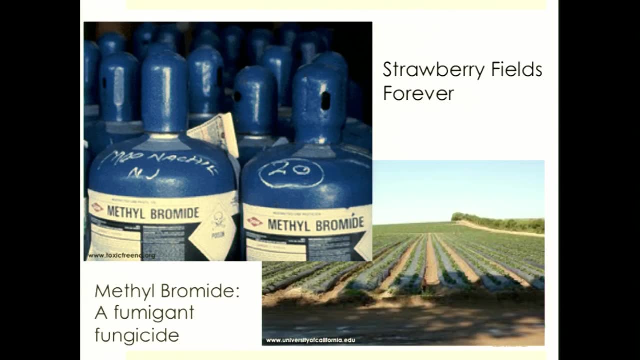 and neurobehavioral development. We are also looking at personal care products And methyl bromide, which is allowed to be used in agriculture right now. It's a fumigant fungicide. Many of you may have passed agricultural fields down in the Salinas Valley. 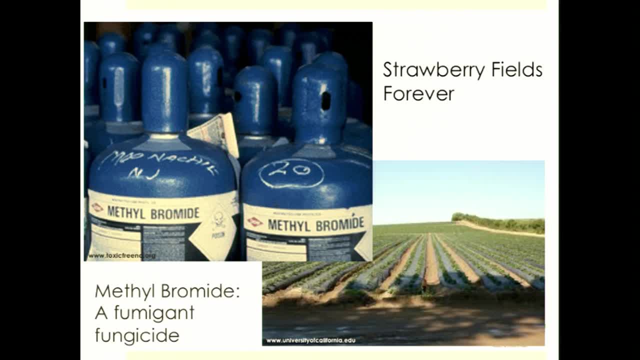 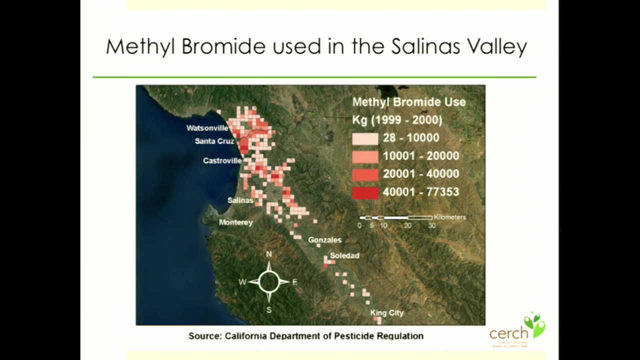 where you've seen plastic. Sometimes that plastic is over the fields because it's just been fumigated with methyl bromide. Sometimes it's just to keep the moisture in. We are now looking at the relationship of where people live in relationship to where methyl bromide 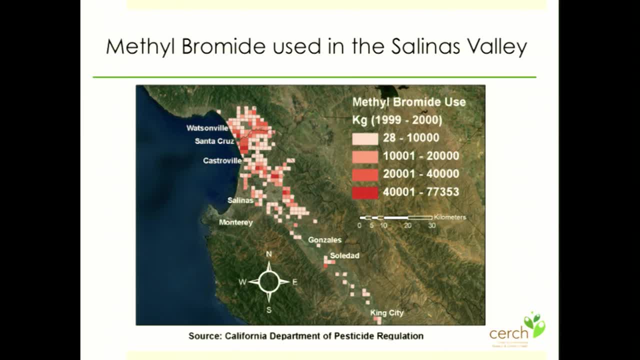 was used, And the reason why what Mike does is so important is that there's really no good biomarker of methyl bromide for the body, which means we have no way of measuring it in the body, And so the best thing that we've got 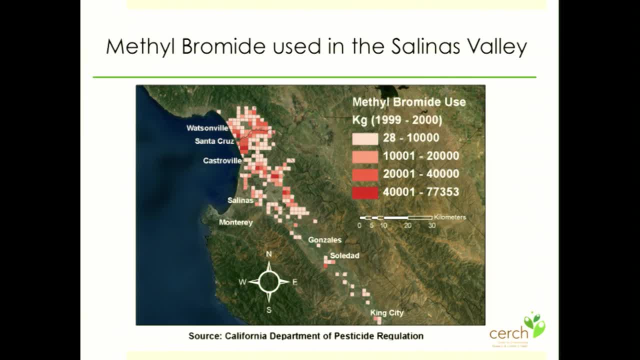 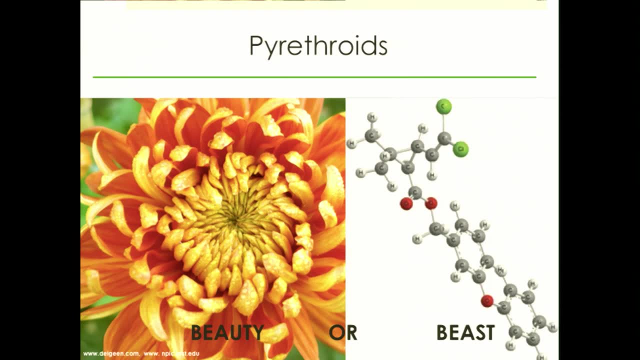 is looking at where you live, in relationship to where those sprayings occurred. We are also looking at pyrethroids And many people used to talk about: oh, they're a natural pesticide, because the original ones came from chrysanthemums. 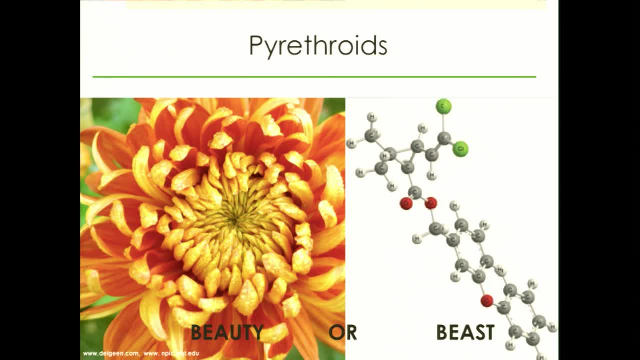 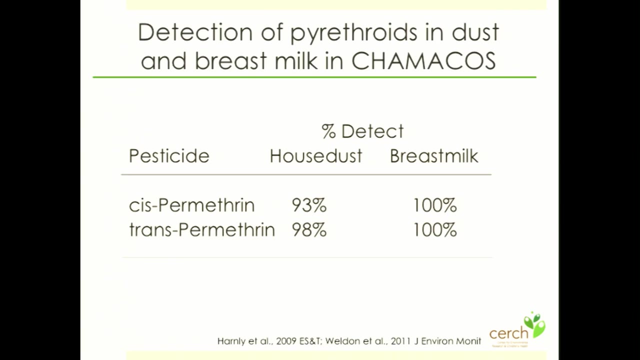 But they've been synthesized And we really don't know anything about the health consequences of these very widely used pesticides. We know virtually nothing. We do know, however, in the Tremaco study, that we pick it up in every single home and in all the breast milk. 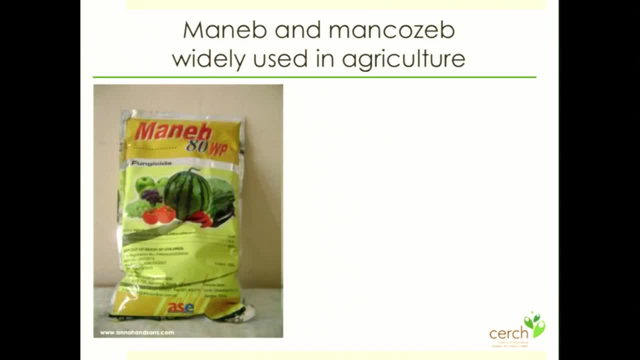 samples we've tested. We're also looking at another class of chemicals that are widely used in agriculture. They are fungicides. They work against funguses, Fungi- They are used mainly in lettuce and salinas- And compared to organophosphates. 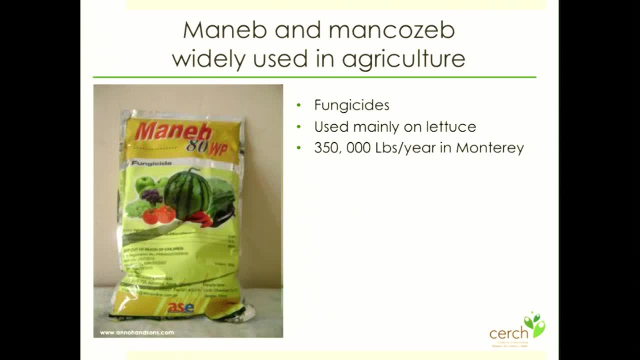 where there's about half a million pounds applied in the Salinas Valley. for these two chemicals alone, 350,000 pounds a year are applied in Monterey. They are 21% manganese by molecular weight, And should we be concerned about that? 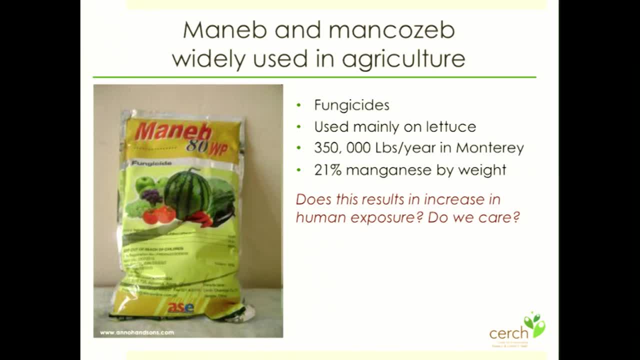 Does this result in increase in human exposure? And do we even care? Manganese is an essential nutrient, So why should we care? But it's only an essential nutrient in high doses In animal studies. there's a lot of evidence to show. 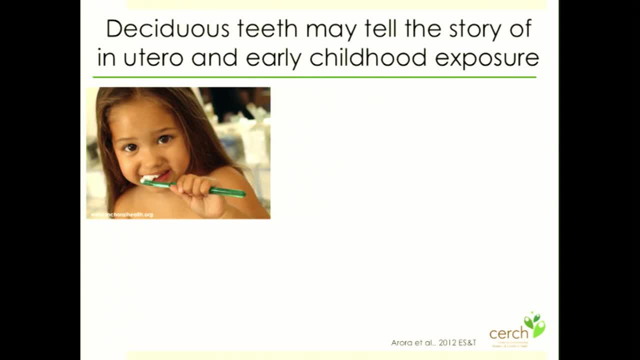 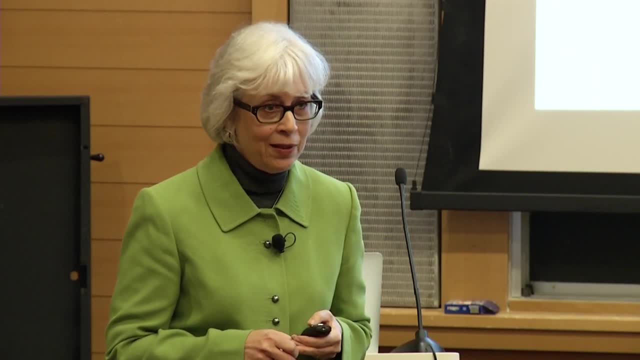 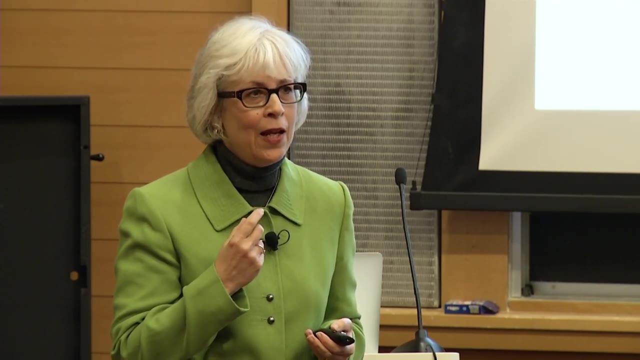 that manganese is a neurotoxicant. It affects the nervous system And we are doing something that is very unusual. Remember I said in 1979 Herb Needleman took teeth and he ground up those teeth and looked at lead levels in teeth. 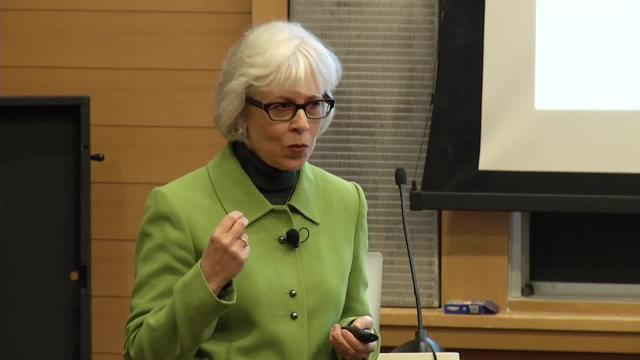 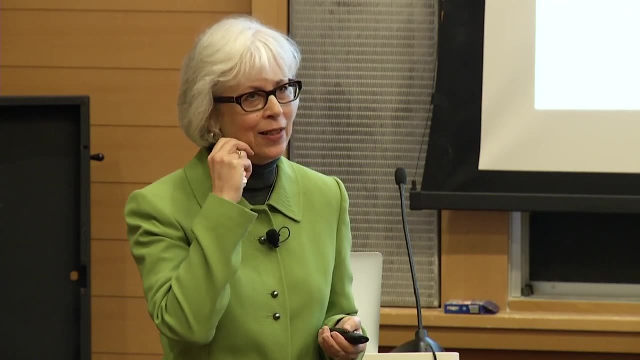 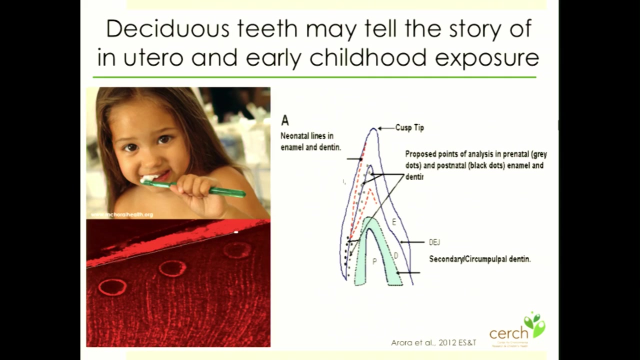 We are working with probably the only environmental dentist in the world. His name is Manish Arora And he asked us to collect. well, we had already collected the teeth, but he asked to analyze our teeth, And what he's doing is he's doing laser ablations. 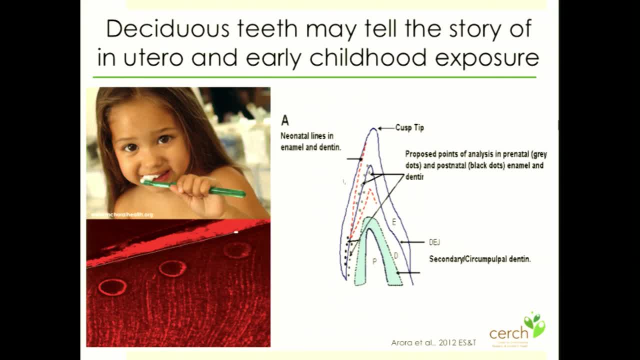 along something called the neonatal line. So the moment a child is born there is a change in the crystallization of the tooth, And so you can actually see in a tooth under a microscope where the formation had occurred before the child was born and what happened. 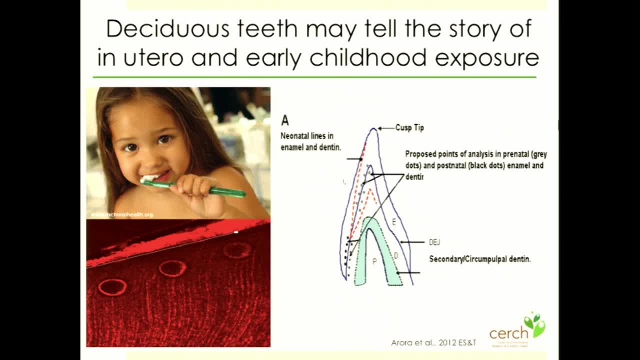 after the child was born. Does it sound familiar? Like the rings of a tree, Right, Depending on where you do an ablation, you actually can get a different weak gestation, just like the rings of a tree. So what he is doing? 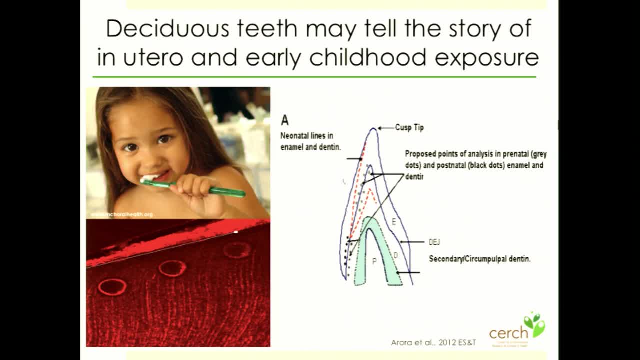 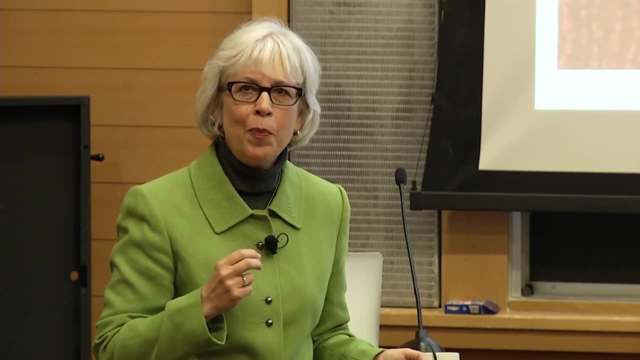 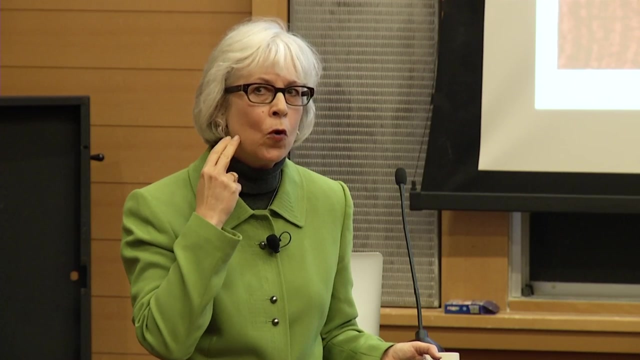 is, he is creating a little dust in those teeth and analyzing those dusts for manganese and other things as well. So we can now take a kid's tooth and tell the story about in utero and early life exposure. So, for example, the incisor begins to form. 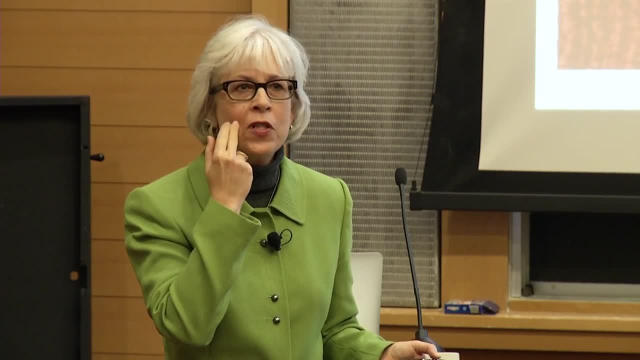 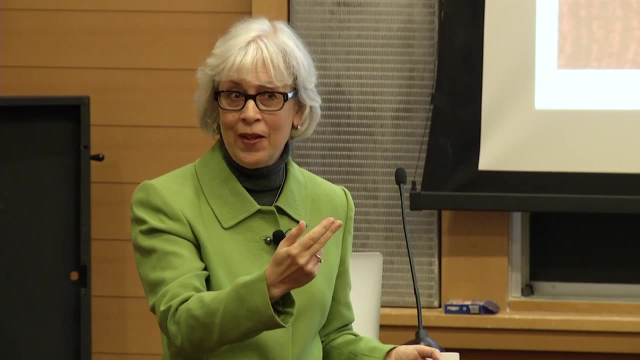 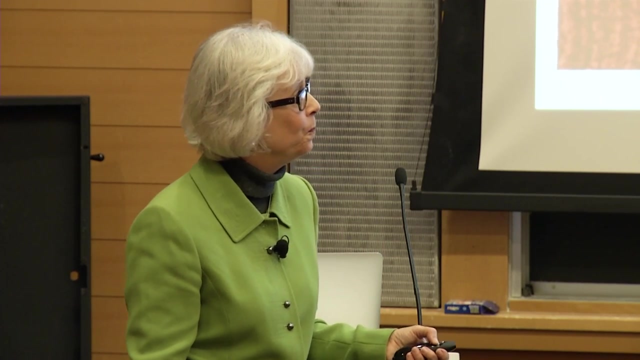 prenatally and continues to form for the first six months postnatally. Different teeth in your mouth develop at different time frames, So if we get incisors, we can learn something about the latter part of pregnancy and the beginning part of pregnancy. 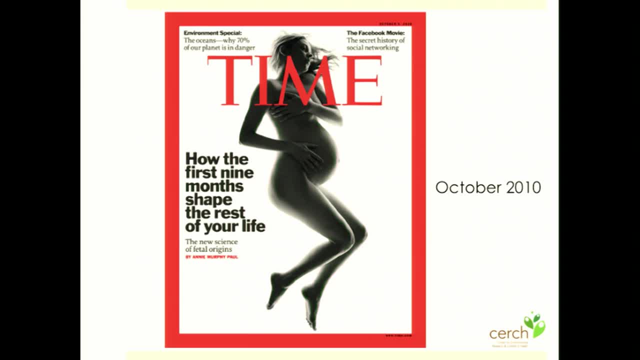 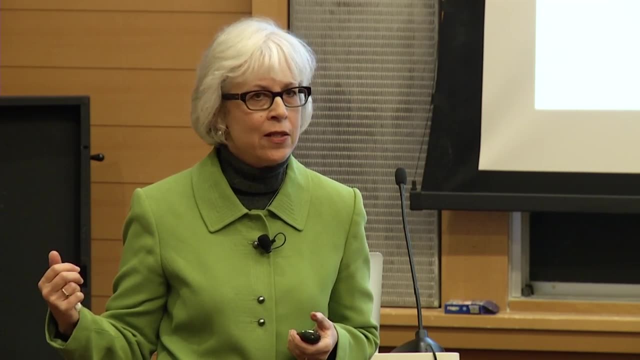 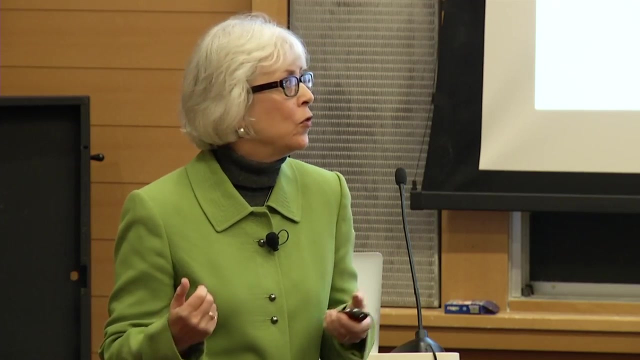 Now this is important. There is a real interest right now that what happens in utero has ramifications for not just that child's health but for future health. So in other words, what you're exposed to in utero may set the stage for cardiovascular disease. 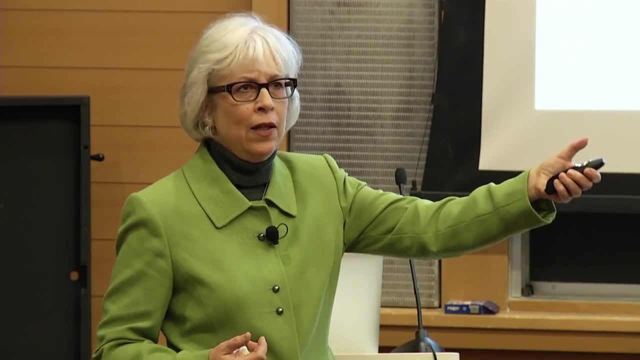 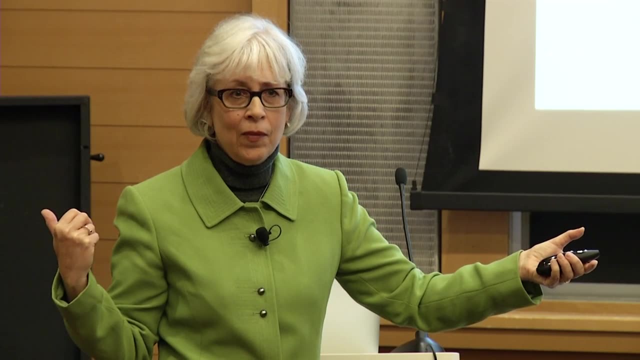 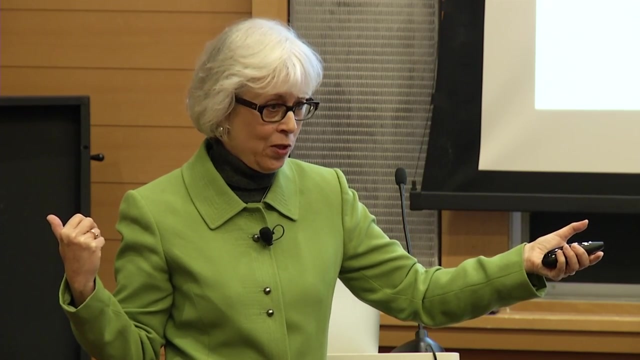 and cancer later, cancer of one kind, and you get a control group that don't have cancer. How are you going to know if they were exposed to prenatally? You're going to ask them. Will they even know How many people know? 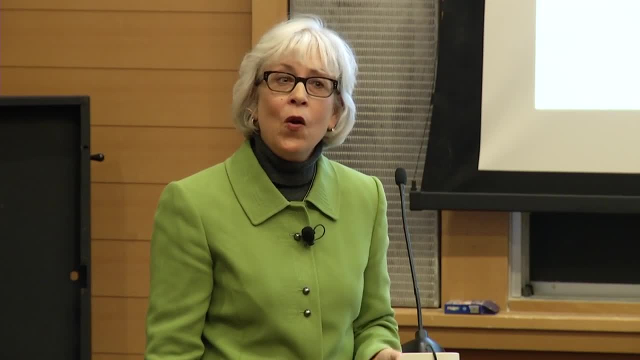 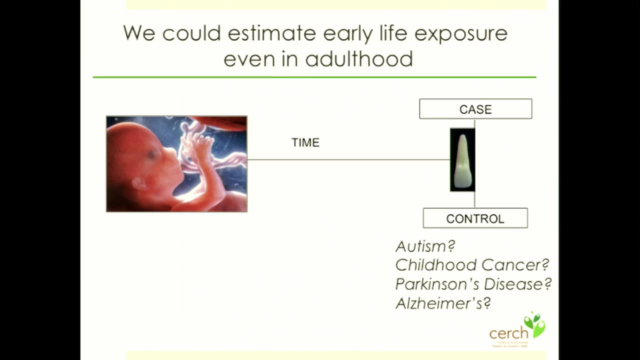 that their mother smoked or not, let alone whether they were exposed to manganese and at what dose. So we can now estimate if we can get someone's teeth like pulling teeth, even in adulthood. So it means that eventually we'll be able to look at. 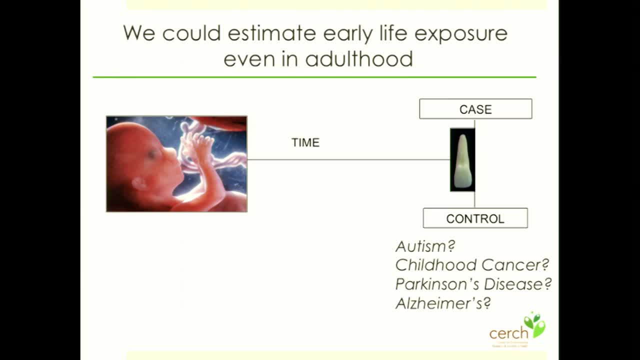 some of the things that people have hypothesized that haven't been able to fully test. Is autism really due to organophosphate exposure? Is it due to pyrethroid exposure? Is the relationship of different chemicals in childhood cancer or Parkinson's disease? 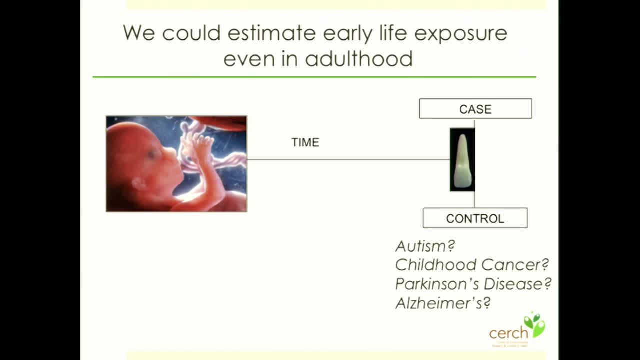 has been associated with Maneb and Mancozeb that are 21% manganese by molecular weight, Or Alzheimer's disease. All of these diseases have had implications that there had been early life exposures to some chemical. If we can get people's teeth- 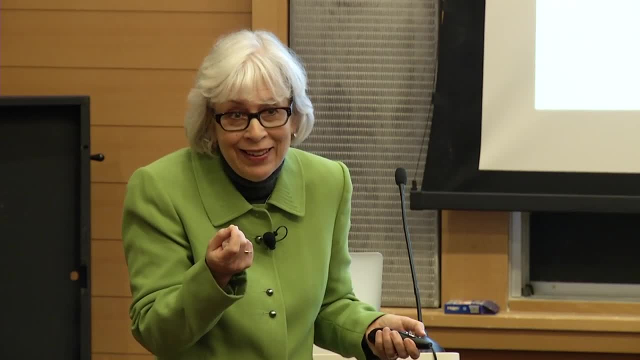 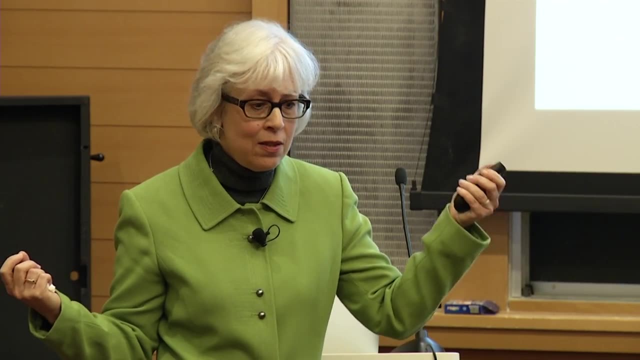 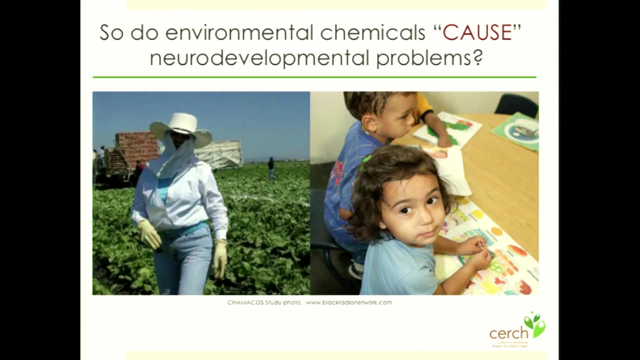 I hate to say this on autopsy even we can then look at prenatal exposure in relationship to adult onset disease, And that changes the game completely. So do environmental chemicals cause neurodevelopmental problems? I don't know. I cannot say they cause. 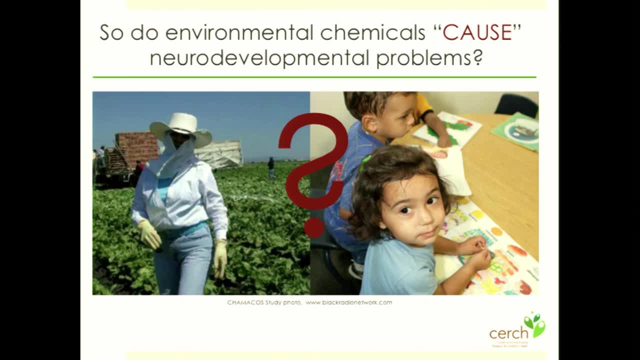 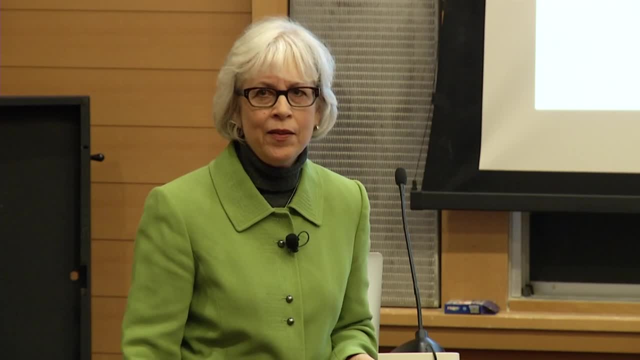 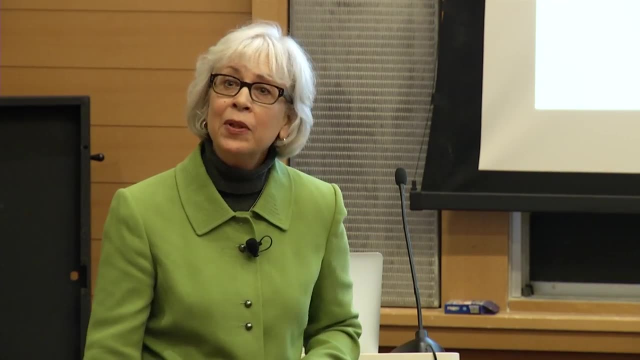 neurodevelopmental problems. I can only say that they're related, they're associated, but these are very complex endpoints And I can't say that a single thing, a single exposure, is causing that endpoint. But I believe as a public health professor. 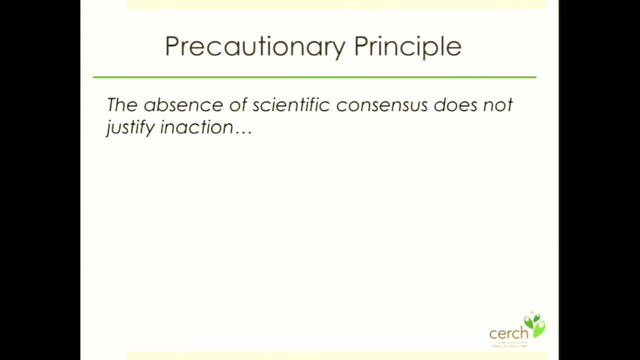 in the precautionary principle, which means that in the absence of scientific consensus does not justify inaction, That when an activity raises threats of harm to human health or the environment, precautionary measures should be taken, even if some cause and effect relationships are not fully established scientifically. 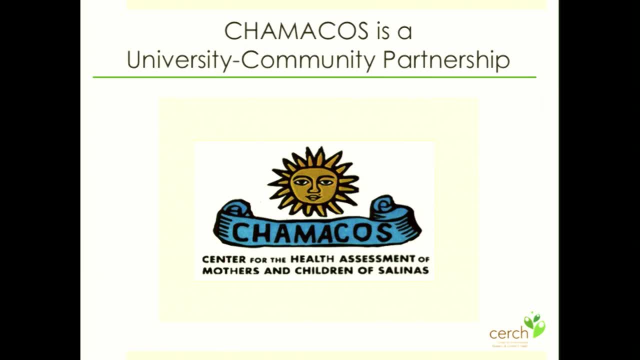 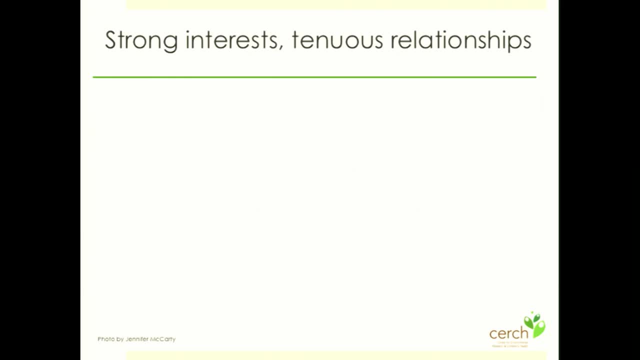 And that's exactly where our community-university partnership comes into play. As you know, the Salinas Valley has a long history: strong interests, tenuous relationships. California is the fifth largest supplier of food and commodities globally: It's a $37 billion industry. 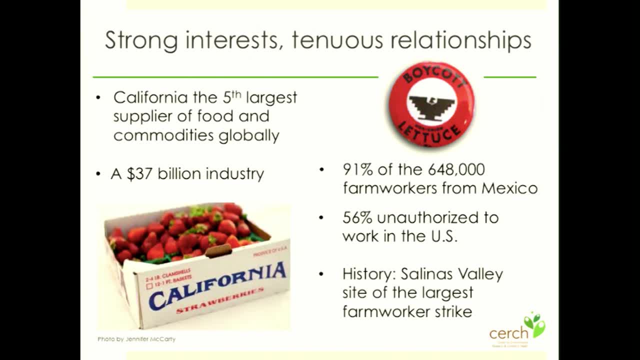 But it's also the home of many farmworkers And Salinas Valley happens to be the site of the largest farmworker strike ever. We decided- mostly Asa and I all those years ago decided that it was important to bring everyone to the table. 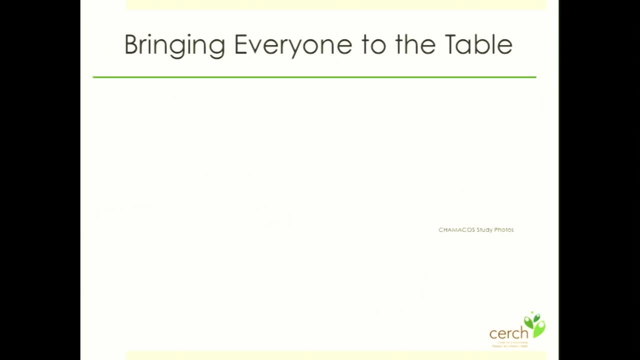 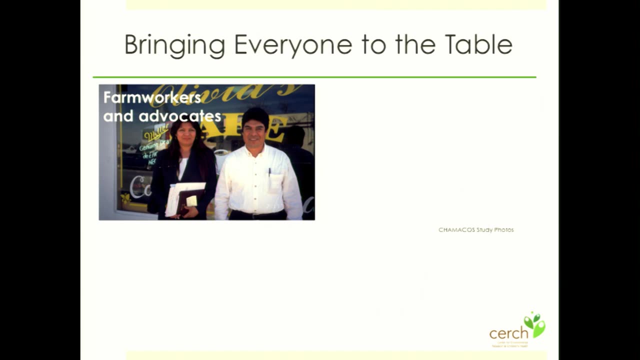 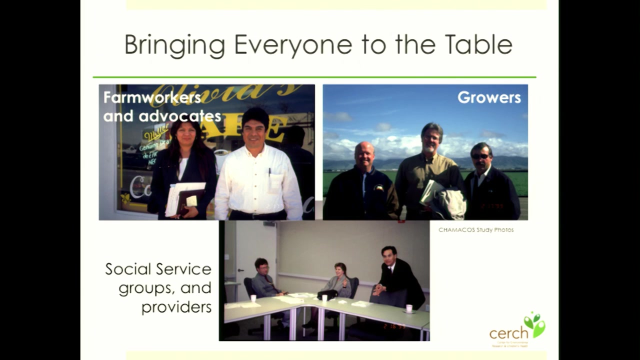 to see if we can improve the health and protect the health of children in the community. So we brought to the table farmworkers and advocates and social service groups and providers, But we also brought to the table the growers And we worked with the farmworkers. 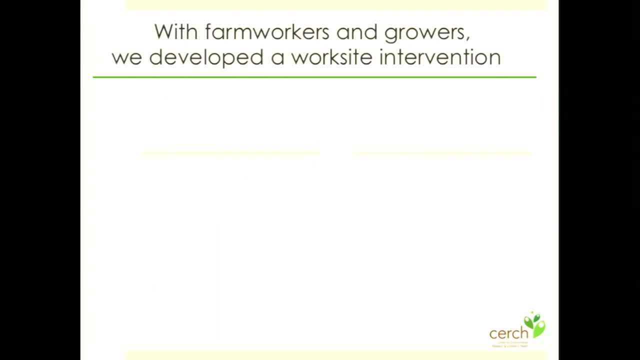 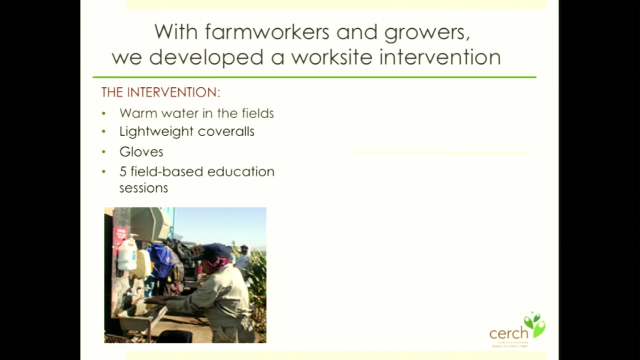 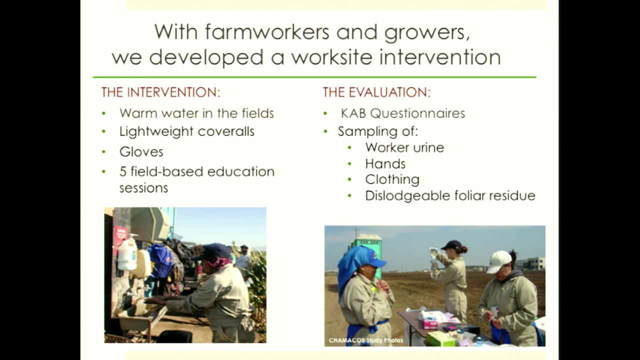 and the growers to develop interventions to reduce exposure to the workers and to the children. For example, we developed an intervention which was work site, where we brought warm water to the field and we gave gloves and coveralls And we showed that there was a change in exposure. 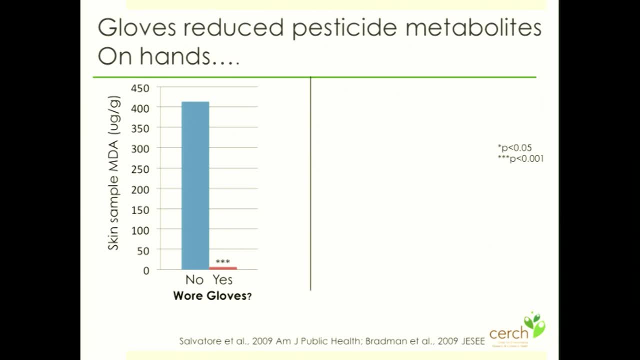 to the farmworkers And we showed that wearing gloves reduced pesticide metabolites on the hands of the farmworkers and also in their bodies. And now the Strawberry Commission- I'm not saying it's a result of our study, but maybe it's related- recommends the use of gloves. 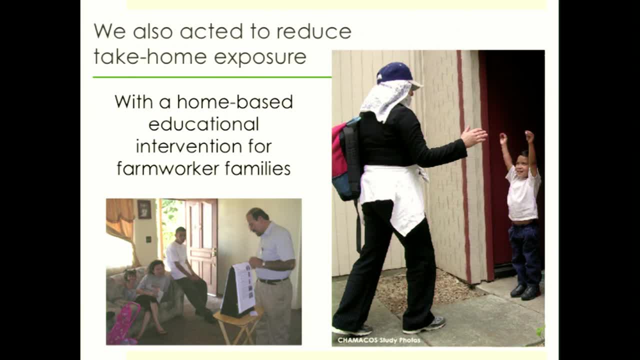 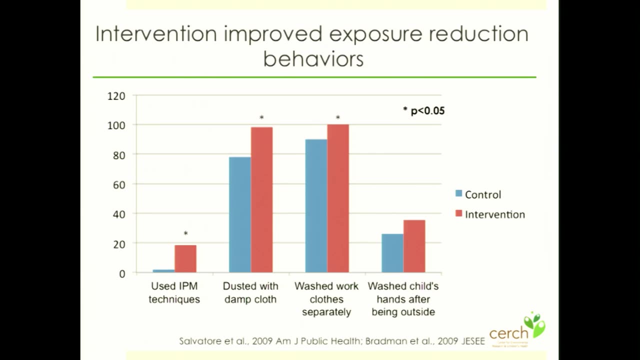 in the fields to strawberry workers. We also acted to reduce take-home exposure with a home-based educational intervention for farmworker families And we have shown that by intervening with farmworker families and we now, by the way, not in this study, but have educated. 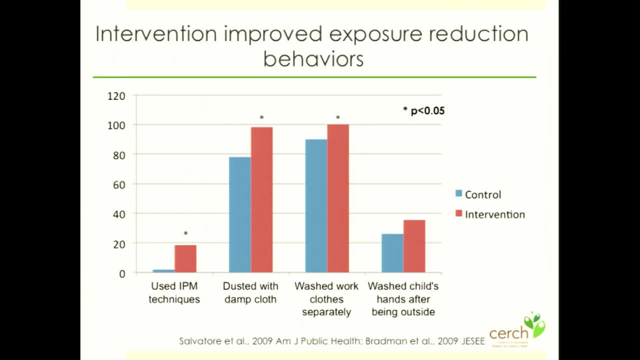 about 10,000. I think it's even higher than 16,000 farmworker families in the Salinas Valley. at this point We have shown in this study that we can actually improve exposure behavior, That we can increase the families using integrative pest management. 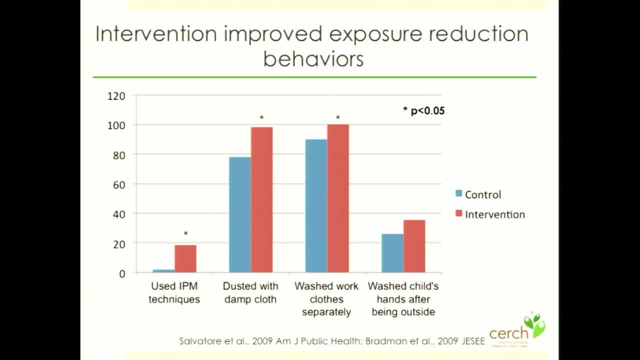 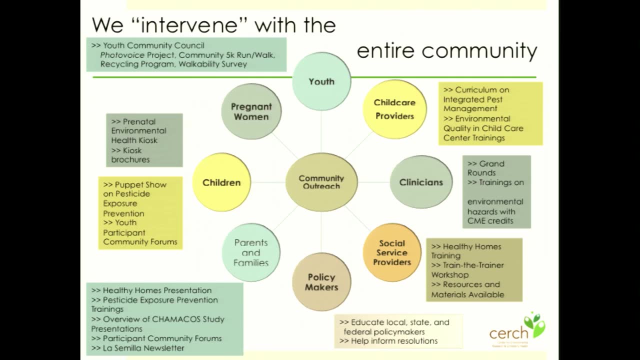 and dusting with damp cloths and washing work clothes separately and washing the child's hands. by our intervention, We have intervened with the entire community, Whether it's the child care providers, the clinicians, the social service providers, the policy makers, the parents and families, the children. 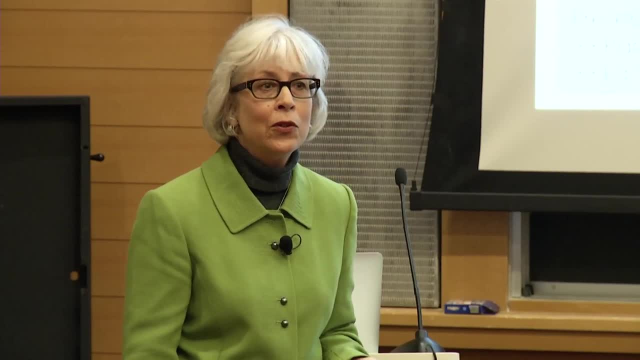 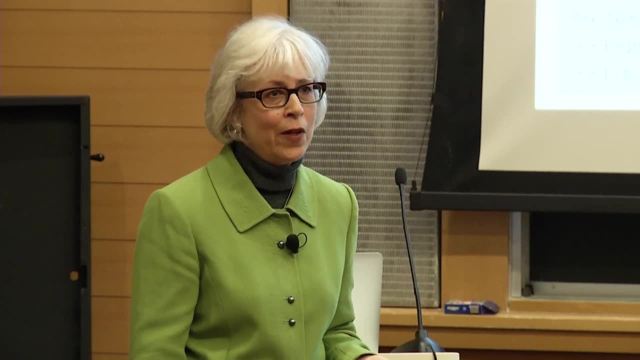 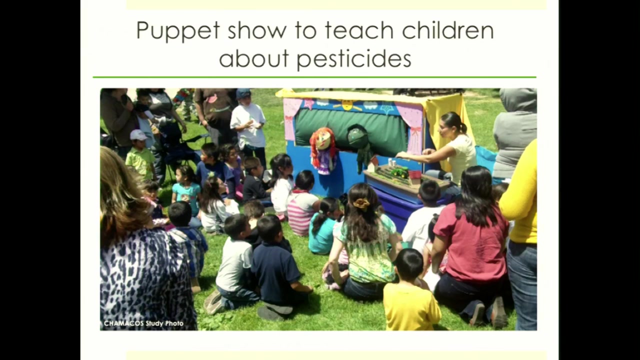 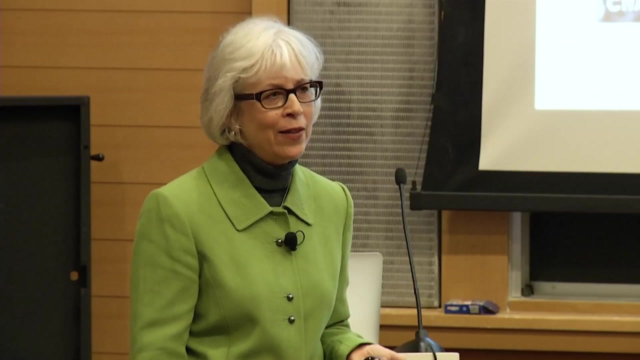 the pregnant women or the youth. One of my favorite projects is that we now have a youth community council made up of farmworker adolescents from local high schools, teaching them about environmental health and public health. We have also taught children, young children, through puppet shows, and we have found that these puppet shows 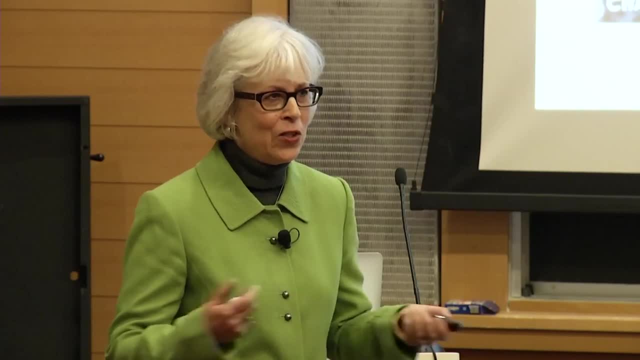 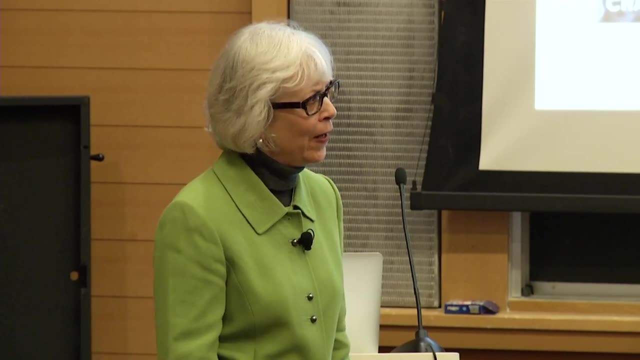 anecdotally are very effective. So I told you earlier that we've educated about 16,000 farmworkers and their families. but one farmworker father came up to us kind of angry and he said: my kid won't hug me when I come home. 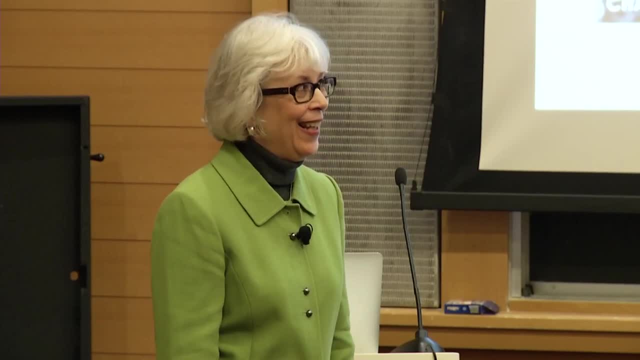 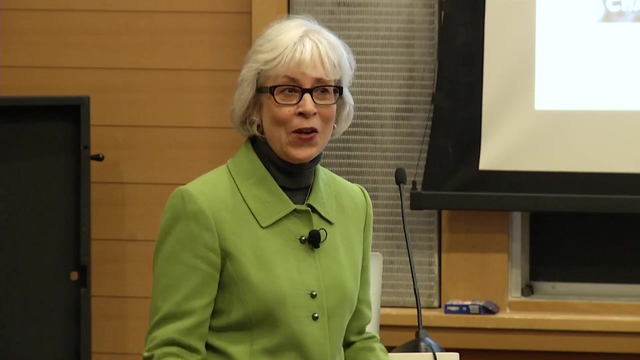 from work anymore and it's your fault. And then he started smiling and he says: and that's because my kid went to your puppet show last week and he learned that I'm not supposed to hug him when I come home until I take a shower and change out of my work clothes. 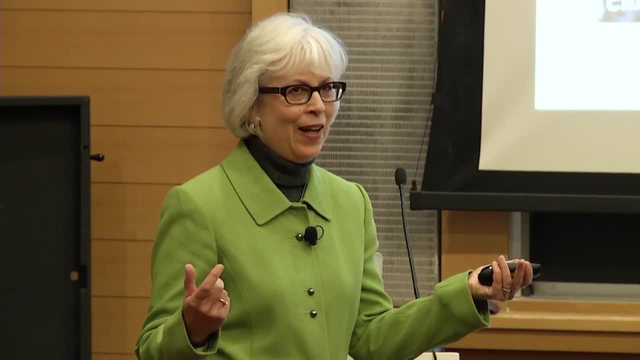 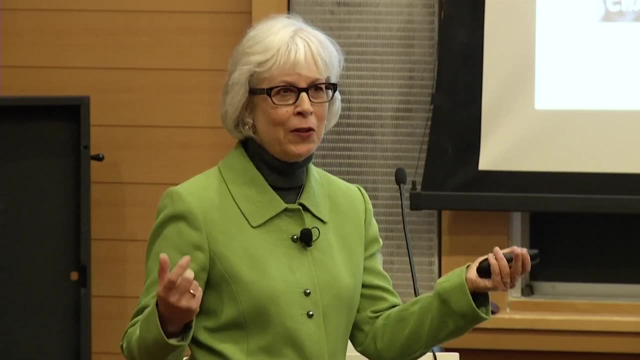 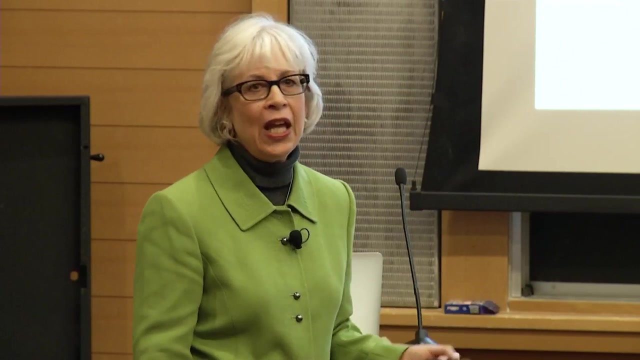 So, just like those of us who were told by our kids when they were young to put our seat belts on, that sometimes the most effective intervener is the child. So we're working at all levels to change behavior. We act globally too. We have been and we've gone. 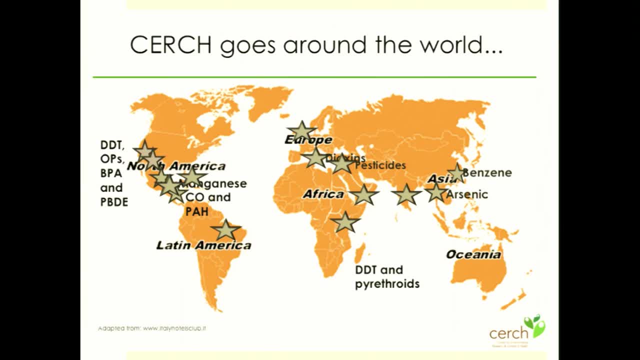 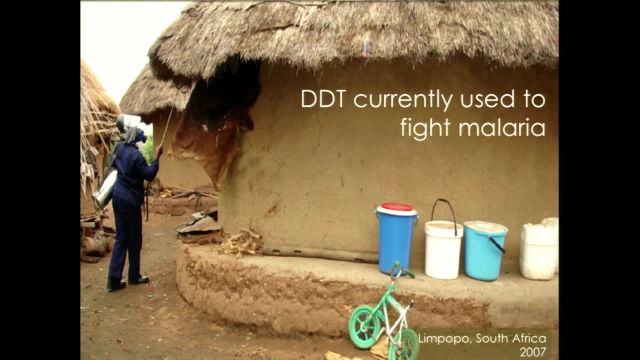 around the world doing different studies. We are engaged in a number of studies right now in different places in the world and most recently we are in Africa doing a study on DDT and pyrethroids. DDT, which has not been used in the United States. 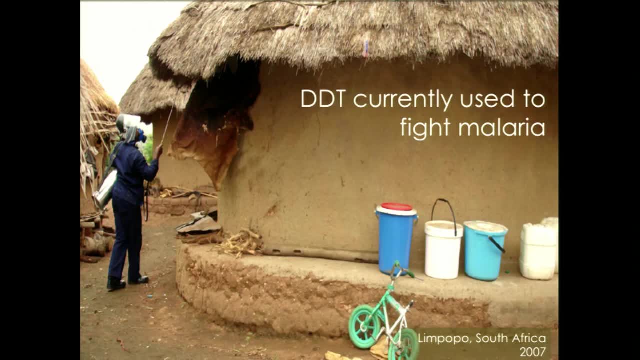 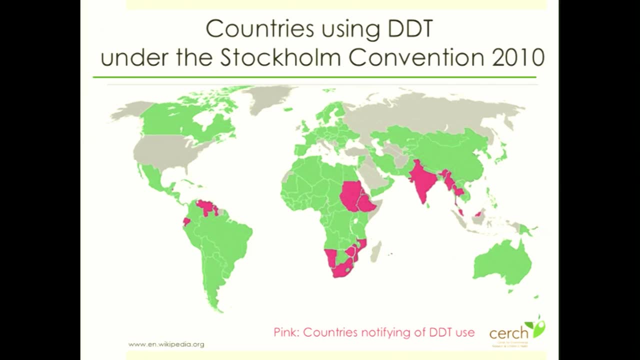 until the early 1970s, is currently used to fight malaria in 23 countries. legally, under the Stockholm Convention, which is a treaty, It is only allowed to be used for controlling malaria and dengue, So it's only for public health purposes. 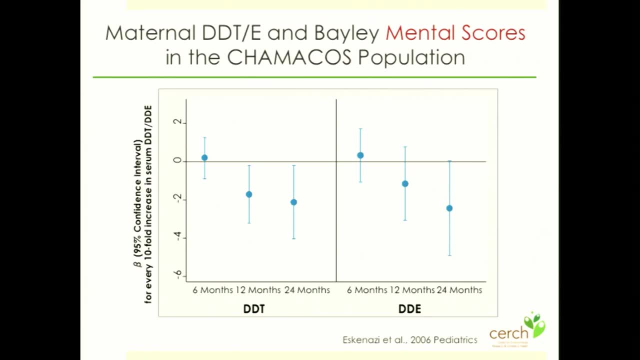 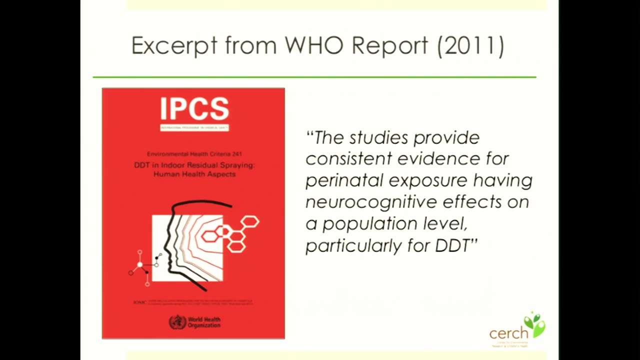 We have shown in an earlier study in Chamacos, which I haven't talked about today, is that there was a relationship between the mother's levels of DDT and lowered mental development at 2 years of age and 12 months of age. That report 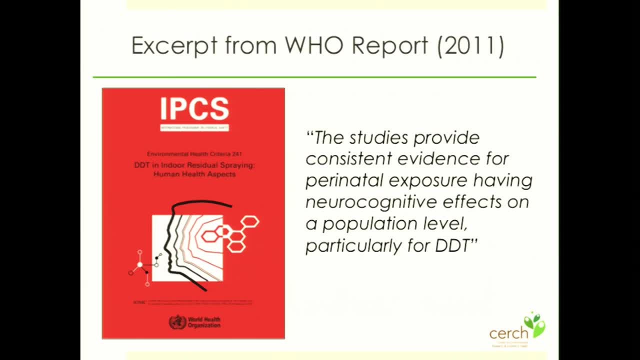 found its way into the WHO report, which says that studies provide consistent evidence for perinatal exposure having neurocognitive effects on a population level, particularly in DDT, And right now DDT is scheduled for phase out in the world In Chamacos. we have 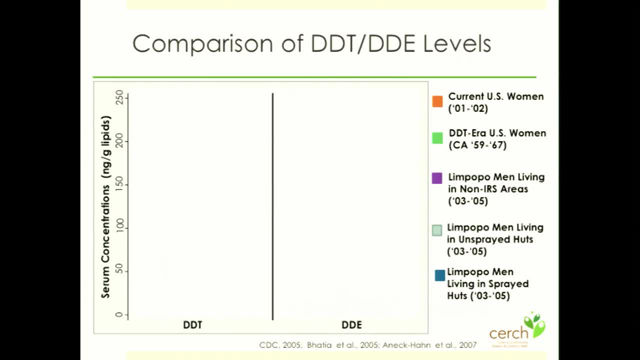 relatively low levels of DDT, but much higher than the general US population. Why? Again, because those women came from Mexico, where DDT was used for malaria control until year 2000.. But let me show you what the levels look like across the world. 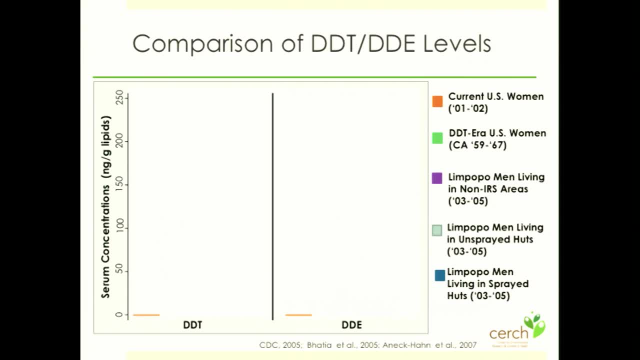 That's the current US population. that little blip down here of DDT, That's in the time when, in the 1950s, when DDT was widely used in the United States in women of reproductive age. This is of men living in communities where I am working. 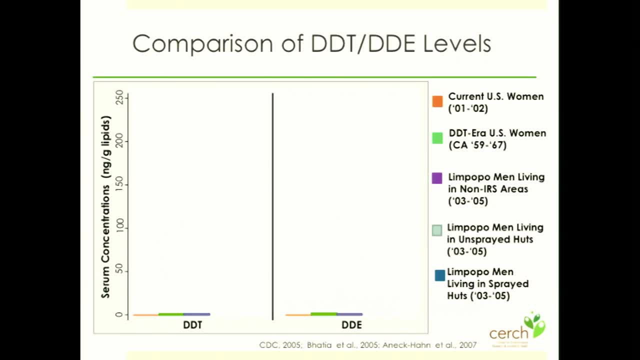 in Africa- Limpopo, South Africa- in places where they're not spraying with DDT. So they spray the indoors of the homes, the walls, the eaves inside the home. It's not the way it was used in the United States. when it was used, 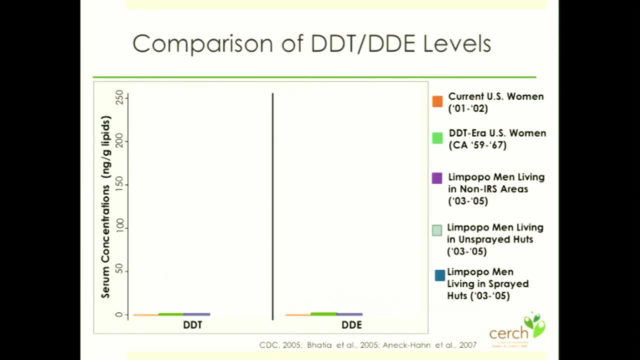 So that's in unsprayed villages, in unsprayed homes. This is the level in men where they live in unsprayed huts but in sprayed villages, And this is the level of DDT in men living in sprayed huts and sprayed. 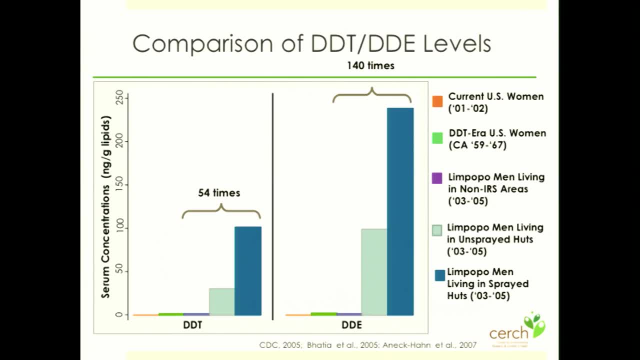 villages. These levels are unlike any levels in studies that have looked at neurocognitive impairment in children. So what we found in Chimacos, the levels were down here. What's going on with the kids who are exposed to levels up here? Our goal: 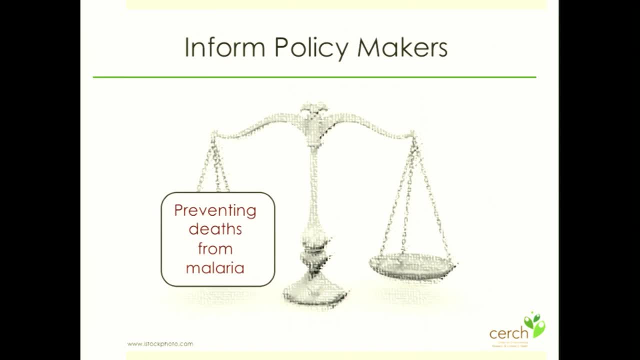 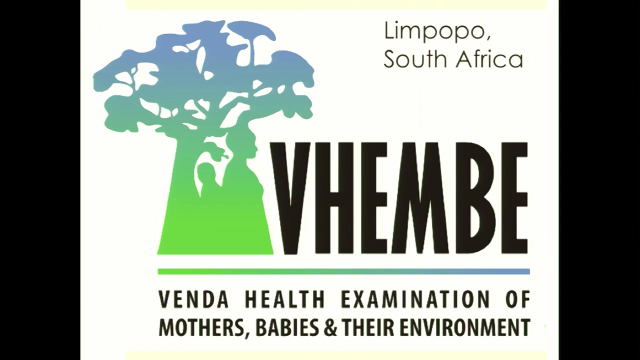 is to inform policymakers. This is a complicated issue. We need to prevent deaths from malaria, but we also need to prevent potential effects of DDT exposure, And that's why we're doing the Vembe study, which is the Venda. 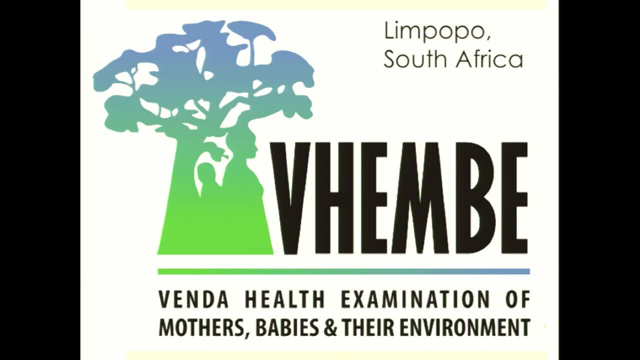 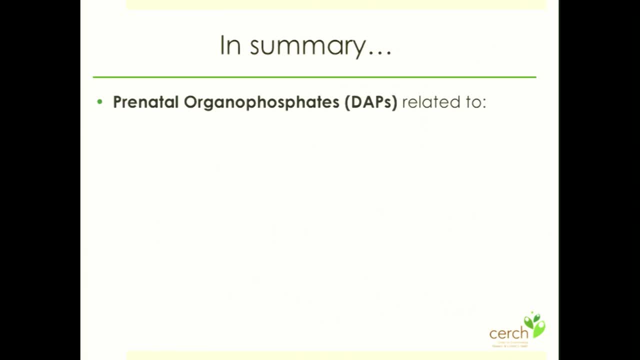 that's the tribe that we're working with: health examination of mothers, babies and the environment in Limpopo, South Africa. So I've come to my end. In summary, we have shown that prenatal organophosphates, as measured, 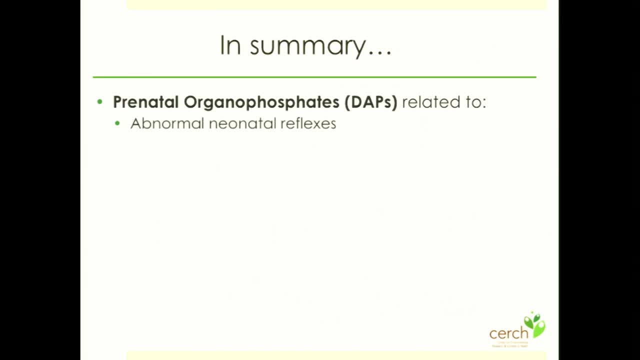 by the DAPs are related to abnormal neonatal reflexes, decreased mental development at two years, decreased IQ at age seven, increase in pervasive developmental disorder at two years and also at five years. but I didn't show that attention problems in school. 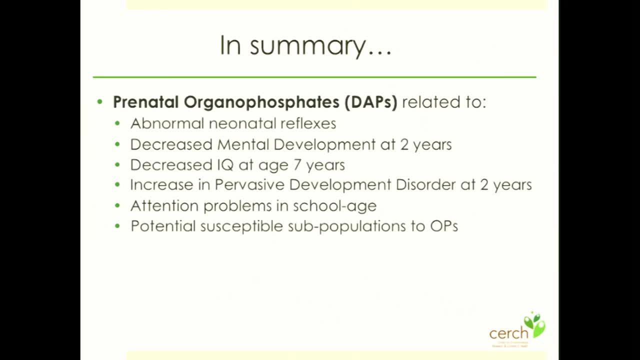 age and there may be potential susceptible subpopulations to OPs, to organophosphates. In terms of the flame retardants, we have shown that prenatal and postnatal exposure, as measured by the blood levels in the mother and the child, 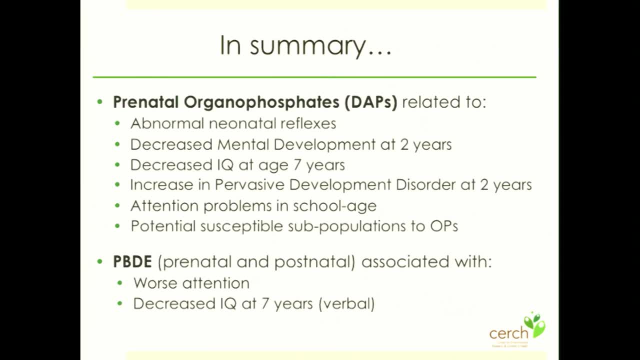 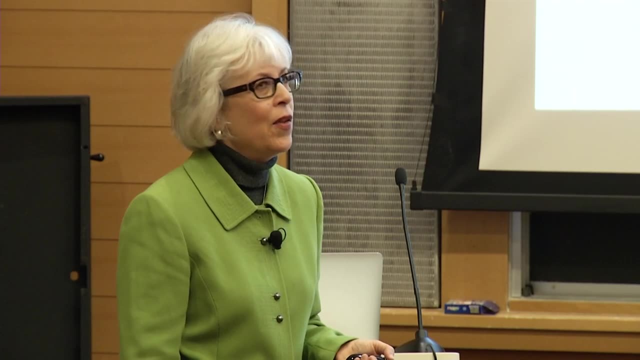 are associated with worse attention, with decreased IQ at seven years, particularly in the verbal domain, and poor refined motor coordination, which I did not show today. But there is change ahead. We have already seen since we started our study in Chamacos that there has been 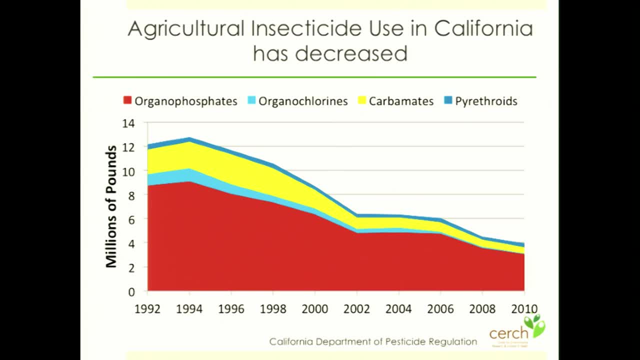 a very drastic decline in the amount of pesticides used for agriculture in California, Not just of the OPs, which are the red- as you can see, it's the lion's share- but of all of the different classes of pesticides. We are seeing a change. 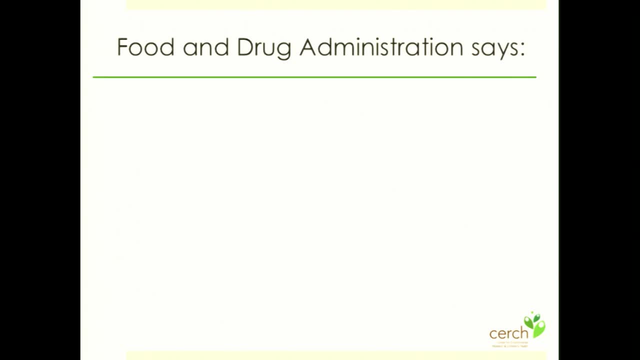 But in the meantime, the Food and Drug Administration says: thoroughly wash your produce, even if it's organic. We all know about the outbreaks of E coli. Wash produce under running water just before cutting it or eating it or cooking it. 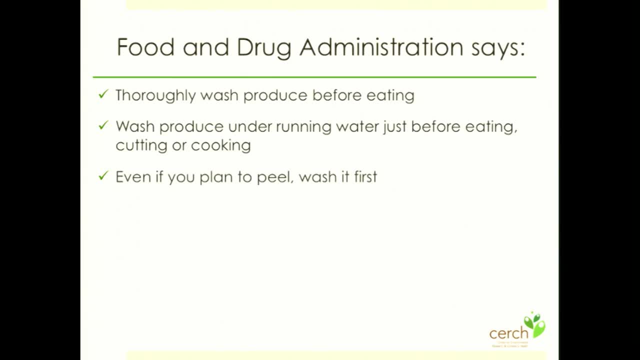 And even if you plan to peel- which I often cheat on- you have to wash the outside first before you cut into it. Washing fruits and vegetables- according to the FDA, especially things you wash with- are not recommended, And they say: 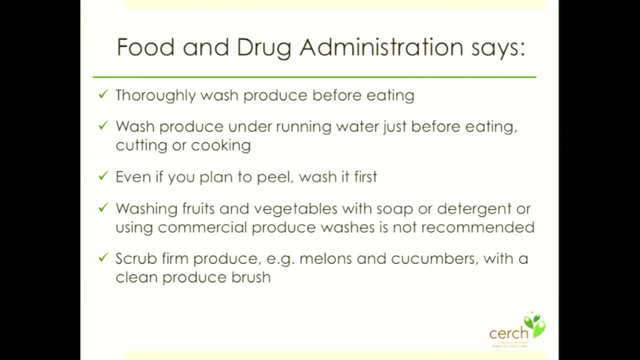 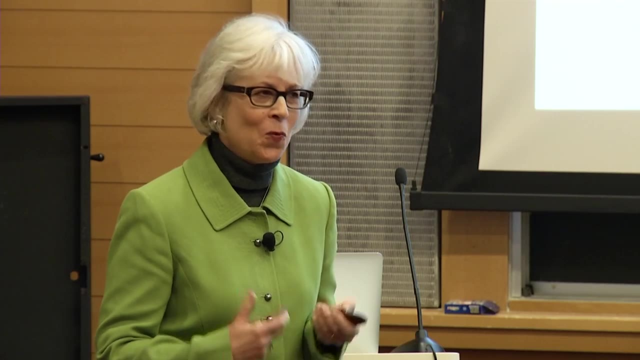 to scrub firm produce, like melons and cucumbers, with a clean produce brush. But one thing I want to make clear, and this is my public health message: the most important thing is to eat lots of fruits and vegetables. Just make sure you wash them. 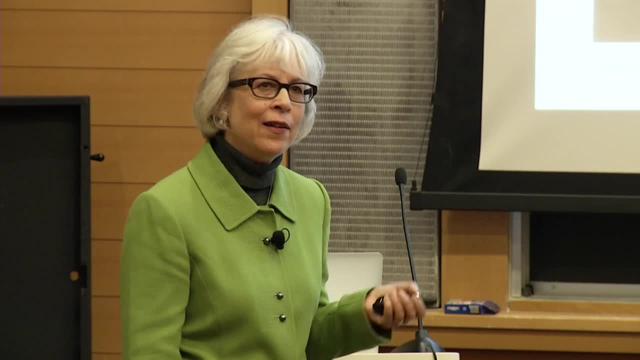 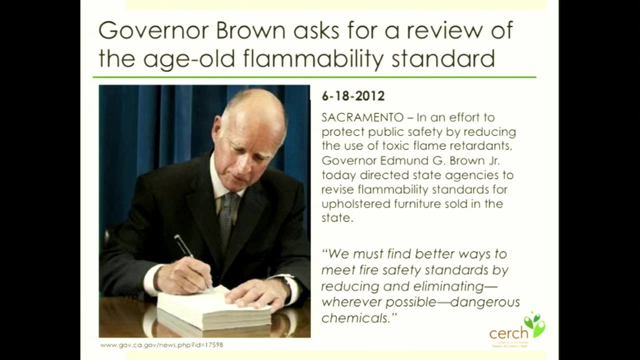 In terms of the flame retardants right now. in June, Governor Brown asked for a review of the age-old flammability standards, So we are in a moment of change. What Governor Brown said is: we must find better ways to meet fire safety standards by reducing. 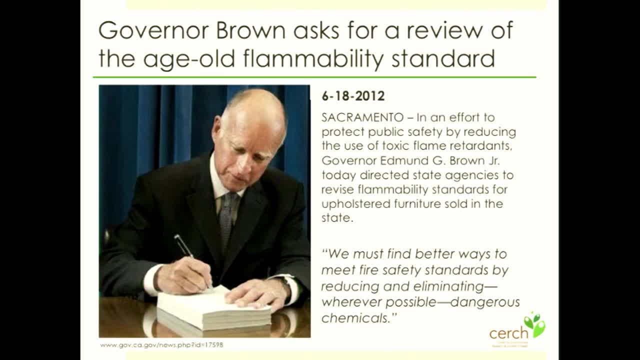 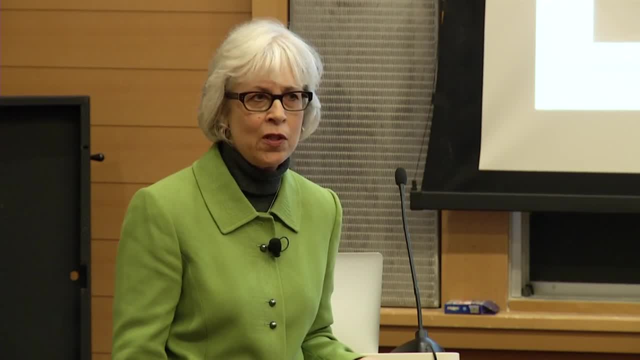 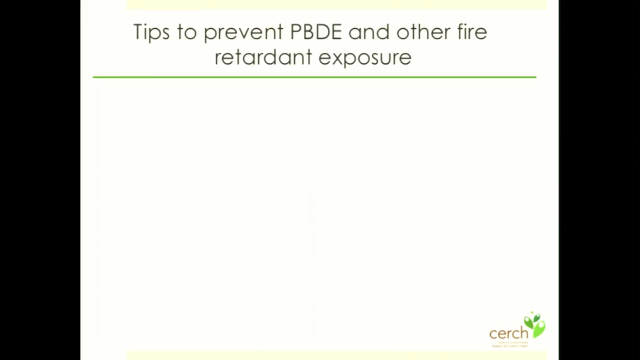 and eliminating, wherever possible, dangerous chemicals. As a public health professor, I don't want children dying by fire, but I also don't want them to be unnecessarily exposed to chemicals that might cause them harm. So tips to prevent PBDE exposure. 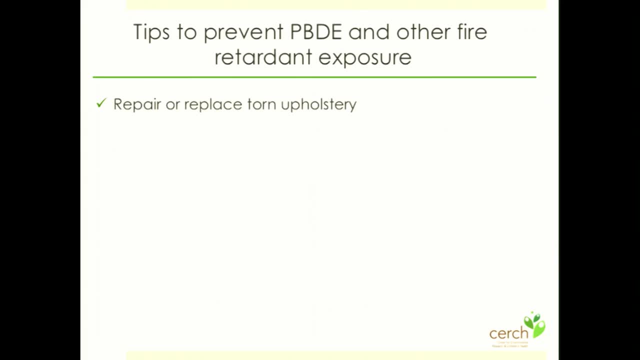 We live in California. We are exposed. Repair or replace torn upholstery. Wash your hands and your child's hands often. Take off your shoes before coming into the house. Use a damp mop or dust cloth to control dust. Open windows to ventilate. 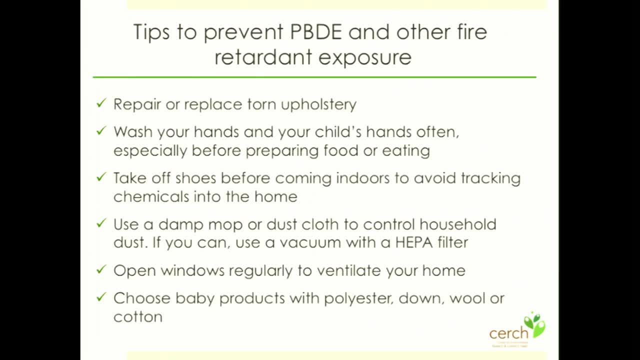 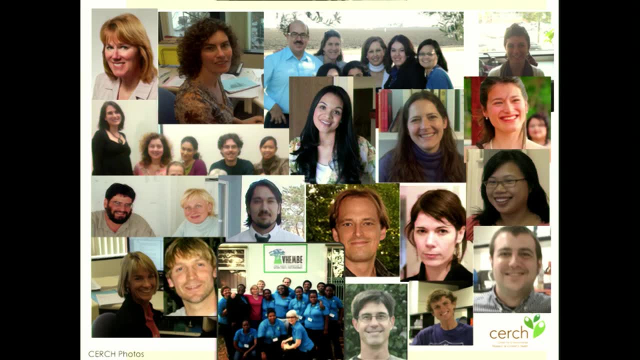 And, if you can, if you've got a baby, choose baby products with polyester, down wool or cotton. With that I'd like to thank- this is only a fraction of the people involved in this study, but I'd like to thank Kim Harley, who is not here tonight. 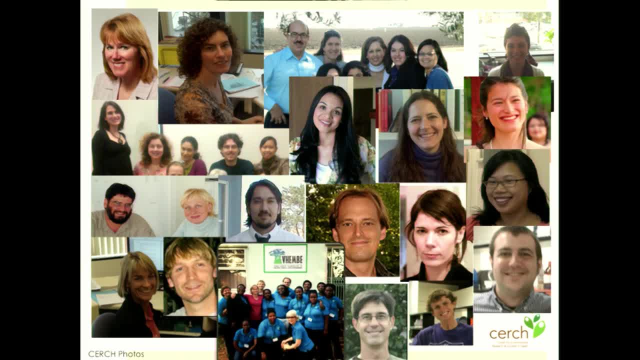 who is our associate director, and Asa Bradman, who is the other associate director, and Nina Holland, who, as I said, runs our biorepository as well as our mechanism studies, and Daniel Winkler and Daniel Madrigal. 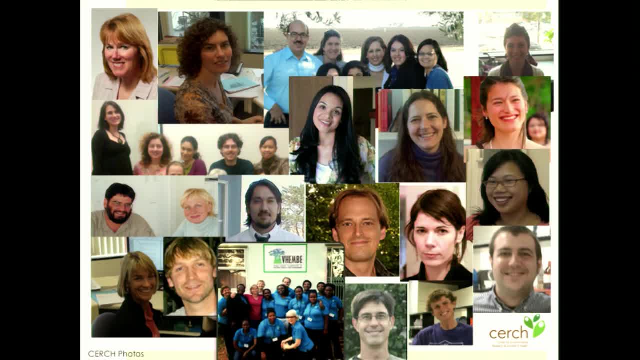 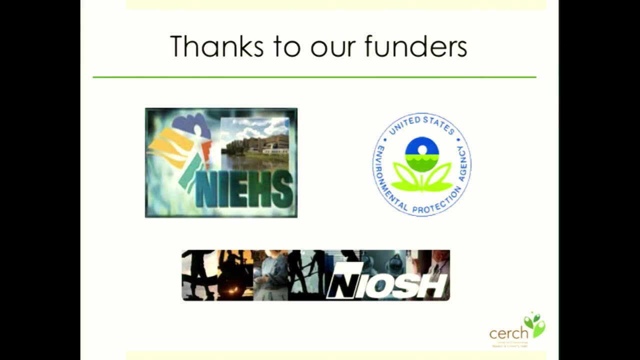 who run the community outreach and translation core, our team in Salinas, our field coordinator Kim and our study coordinator Katie and our field team in South Africa, and all of our other people as well. Vitalia is sitting here too. 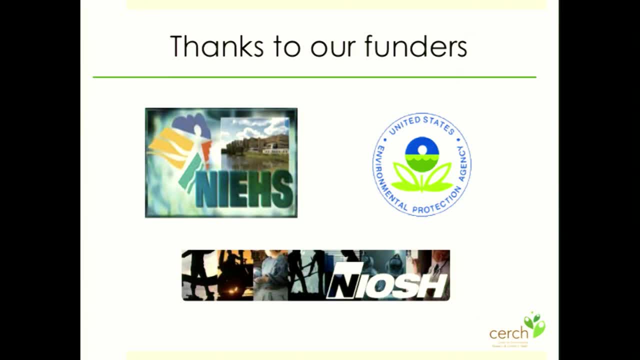 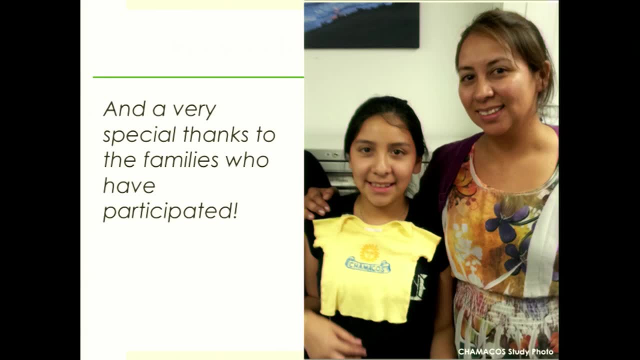 Thanks to our funders, especially the National Institutes of Health, NIEHS and the US EPA and NIOSH, And a very special thanks to the families who participated. This is actually a girl who gave photo consent to be in this picture. 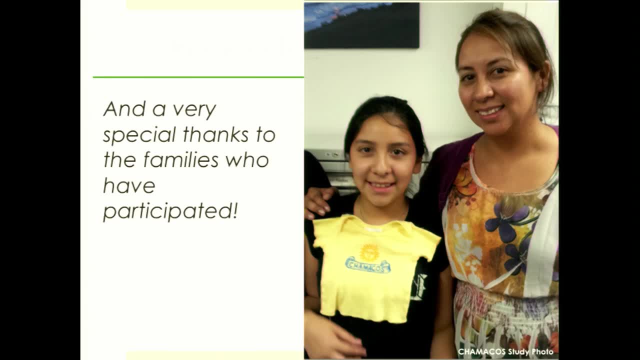 This is the T-shirt we gave her when she was born. She is now 12 years old, And so you can see that they're very involved in our study. This is the mother who cleans houses for a living, and we're told that now she uses only green products. 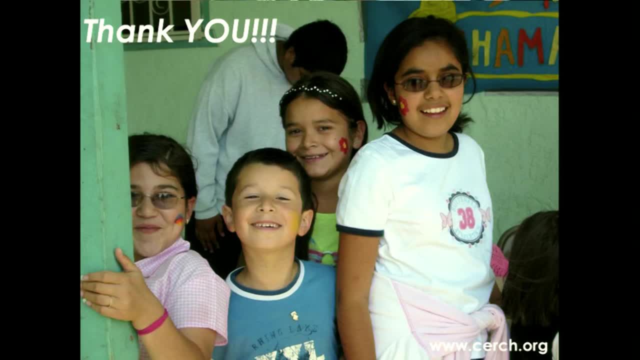 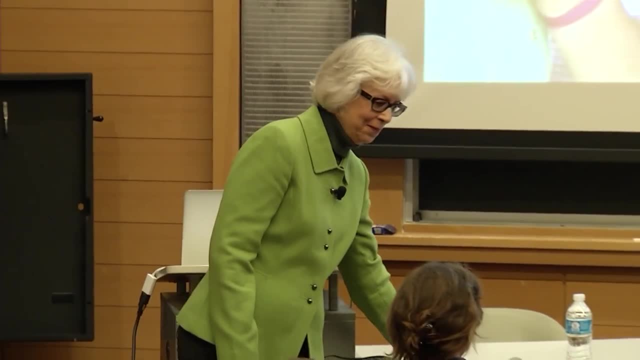 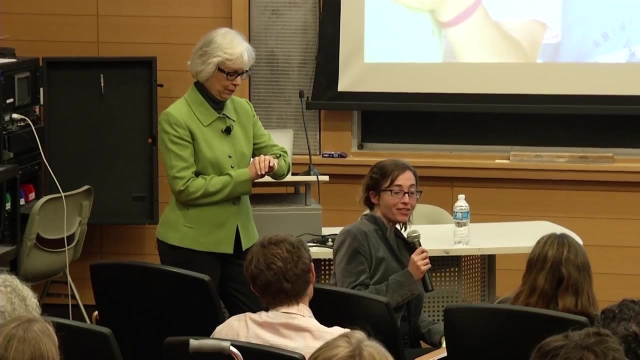 because of chamacos, And we want to thank you. Thank you, Thank you. So I promise that we will end at 9 o'clock, but let's just take a couple of questions for this lovely presentation by Dr Eskenazi. 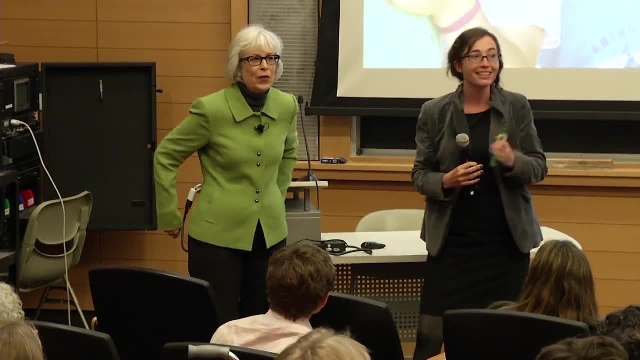 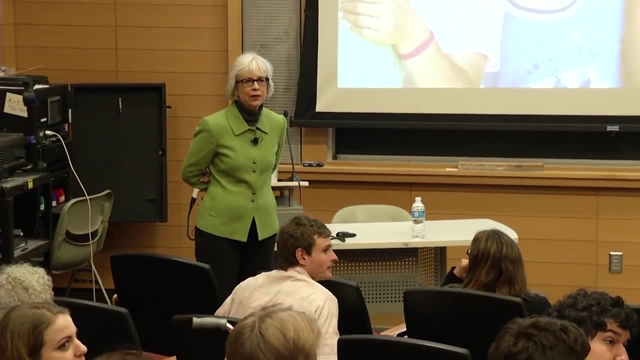 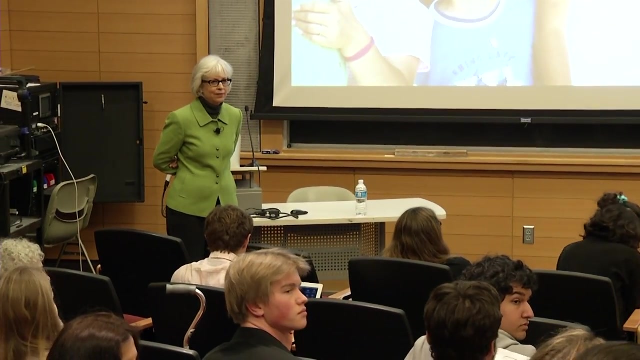 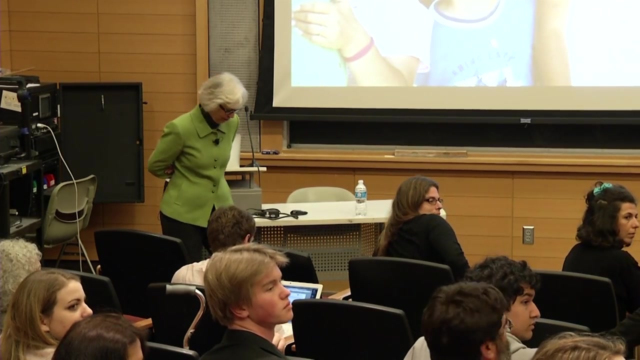 I got this. You got this. Anybody have any questions? You can shout probably, Oh, it won't be on the mic I just had. I was interested in how you answer questions about validity, like scientific validity in terms of. 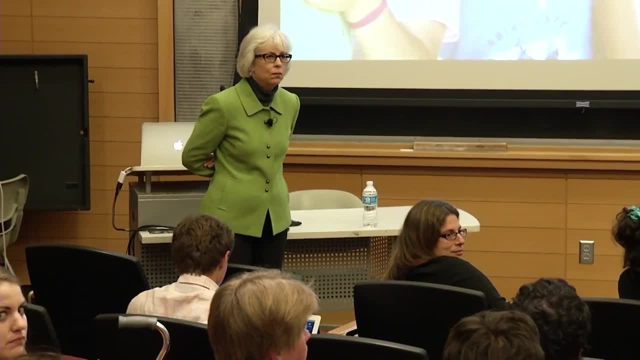 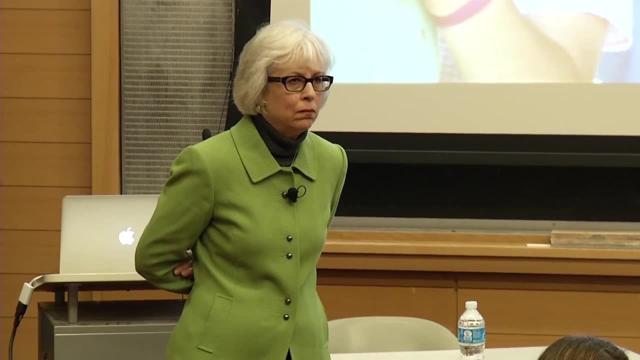 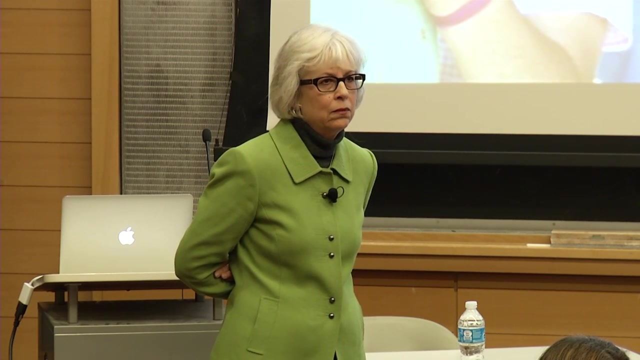 so once you start reporting the work that you've done on methyl bromide, there's a lot of pesticides applied in that area and you said that you know early on, before you started talking about your actual results. you were saying that. 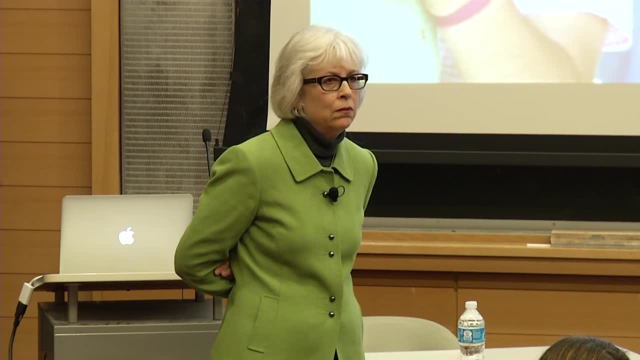 you know you base your epidemiology approach on animal studies, So you're looking at effects that you've already found or that have already been modeled in animals, But then and so that's part of how you choose it. but you did also mention that 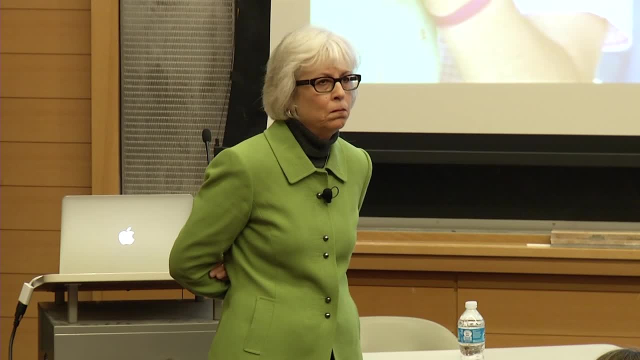 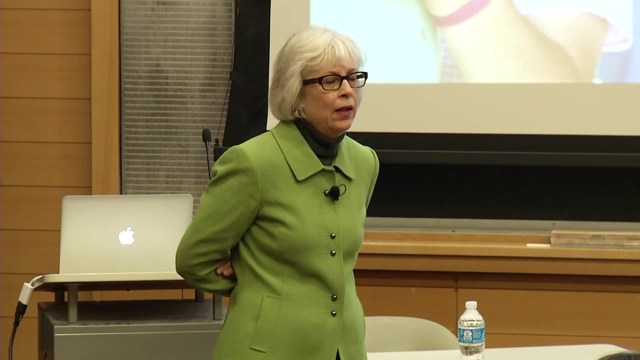 if you looked at all the possible environmental inputs, then you would find an effect somewhere, maybe randomly. that was still statistically significant. So I was just wondering if you could speak to that. Yeah, I think that's a very valid point. What I didn't say is: 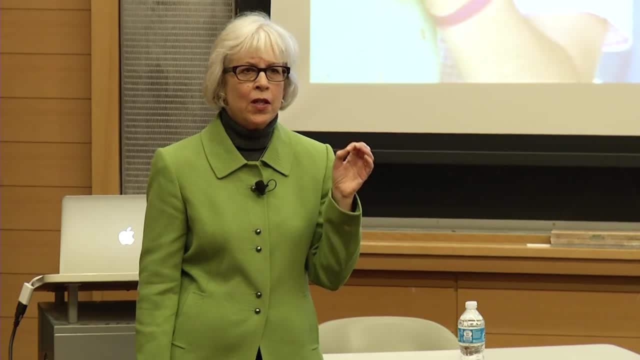 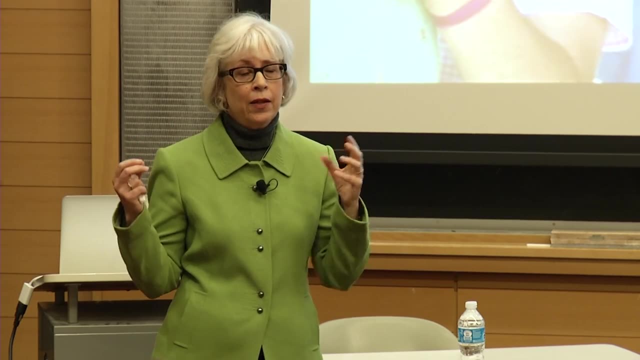 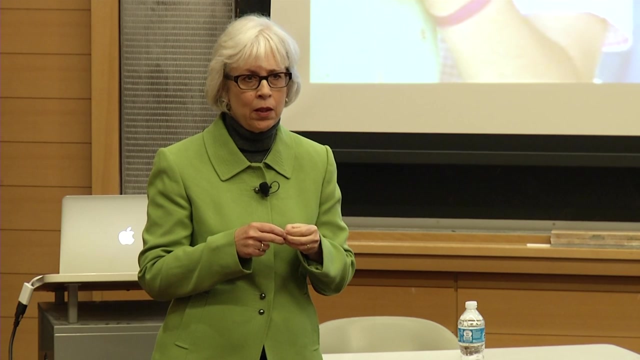 and I think I should say this because I didn't say it- the associations that we saw with the organophosphate pesticides and, let's say, for example, child IQ, and the ones that we saw with PBDEs and IQ were independent of each other. 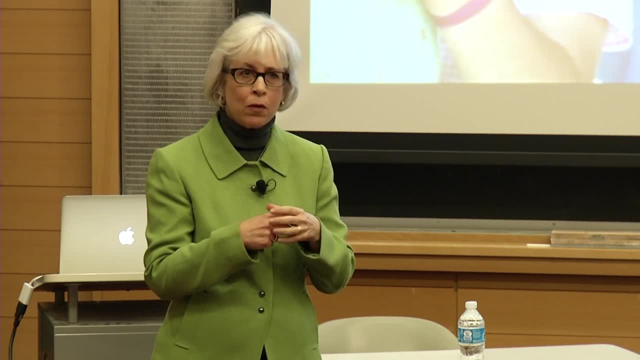 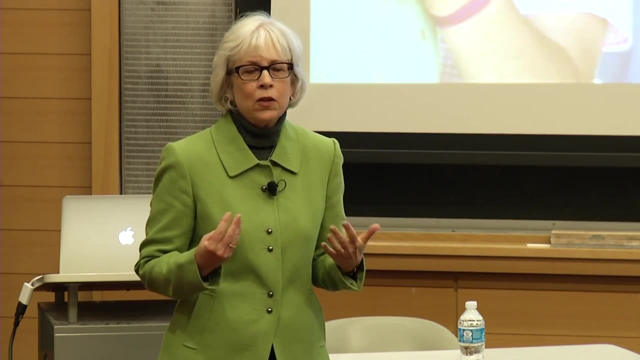 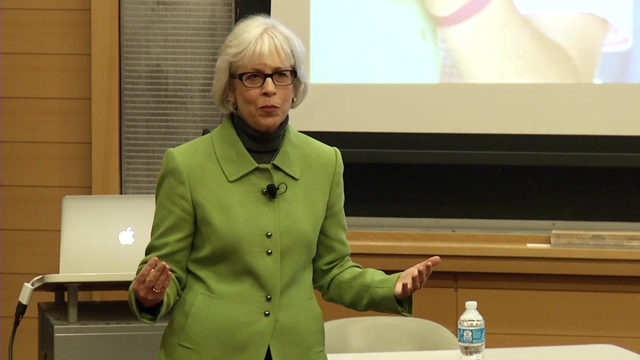 So we looked statistically to make sure that we're not, that there's no overlap, that the associations are independent and they stand alone, And they do. But you know, clearly we have not measured the 80-something thousand chemicals that are used. 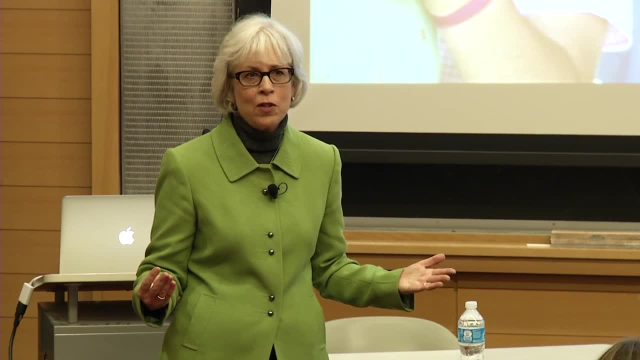 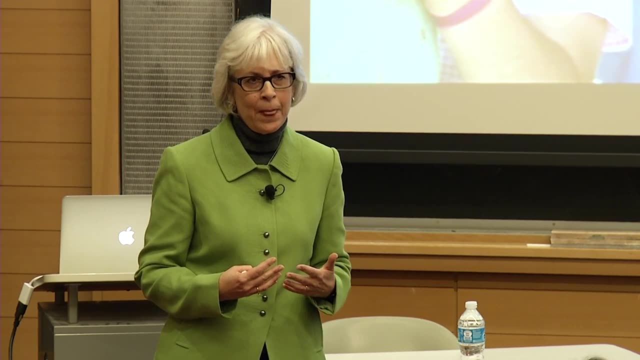 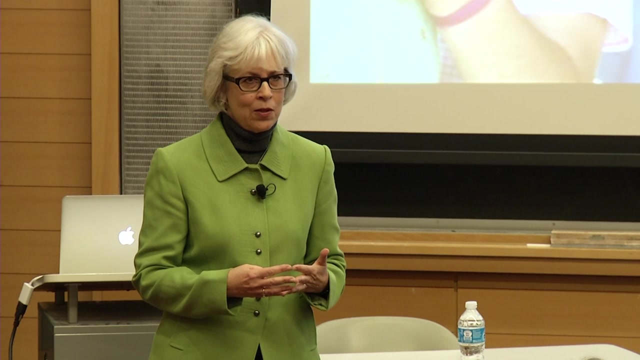 pretty commonly in the United States in the children's bodies. So we can't possibly rule out other chemical exposures and how those affect neurodevelopment. So we could never say that there's causation here We only can talk about associations And we can only 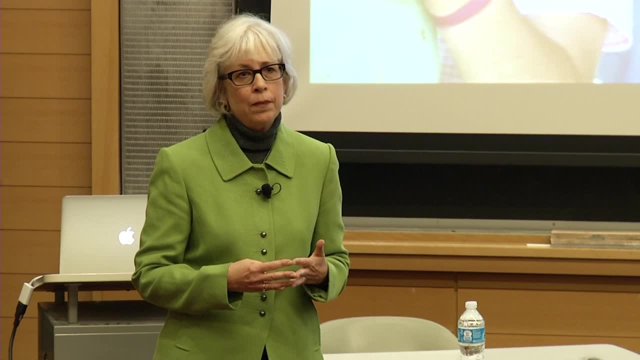 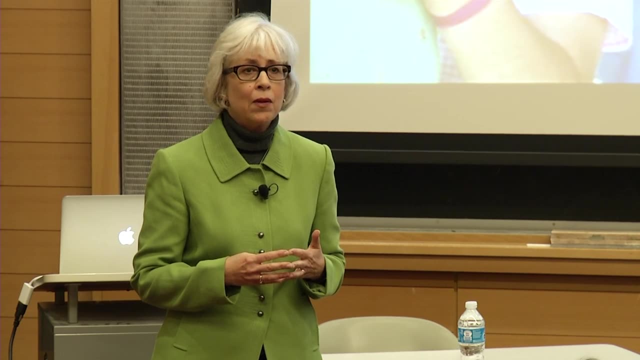 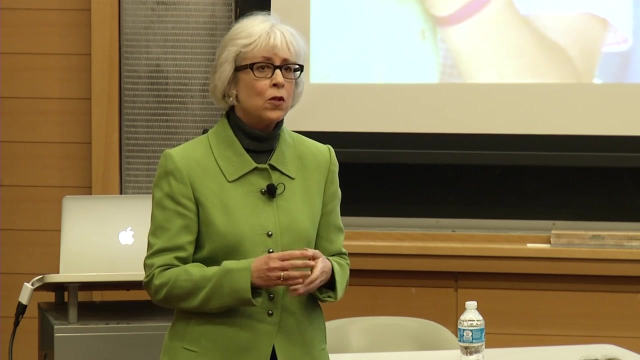 as much as we can control for other exposures, either by having a biological measure of that exposure or knowing something about the location of where that person lives. So, for example, when we look at methyl bromide, looking at the geographic information, we will also control for. 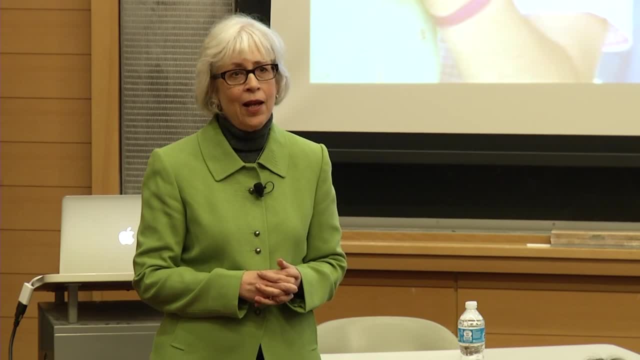 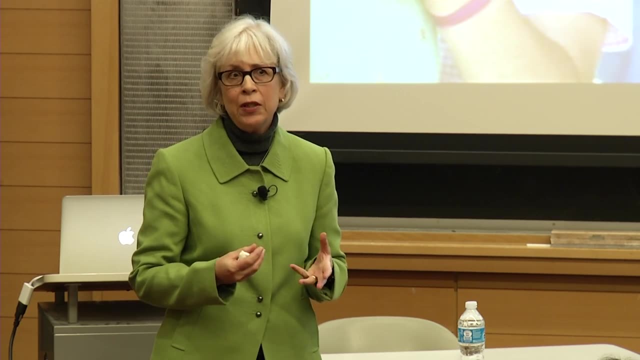 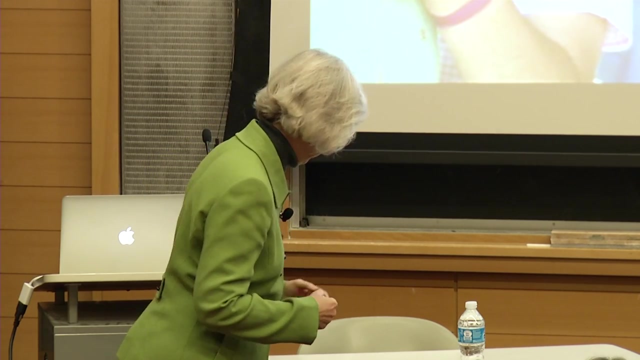 the biological measures that we have. But you're right, It is complicated and it's only by statistics in a way to be able to find independent, to look for independent associations. Have you guys ever looked at polymorphisms in acetylcholinesterase or butyrylcholinesterase? 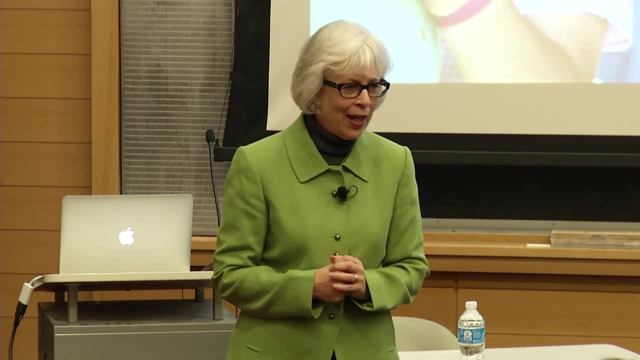 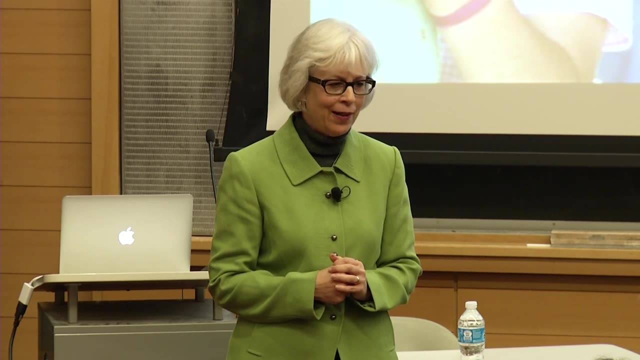 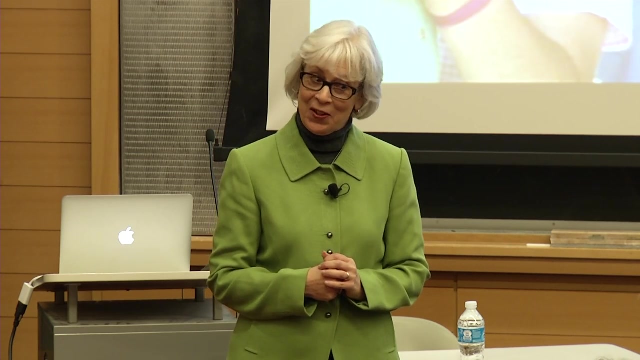 Yes, We have, But we haven't looked at that necessarily in relationship to neurodevelopment yet. We have measured that but we haven't. We've reported on that. And cortisol levels: We haven't measured cortisol levels yet But we could. 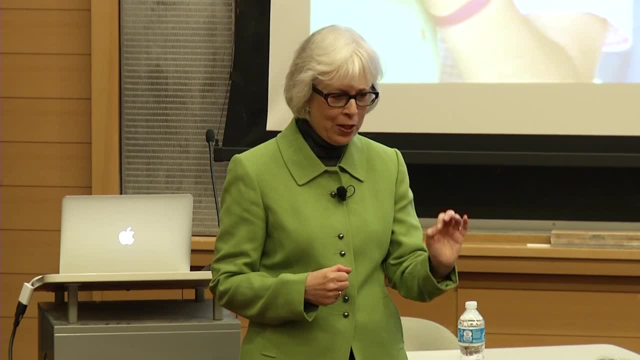 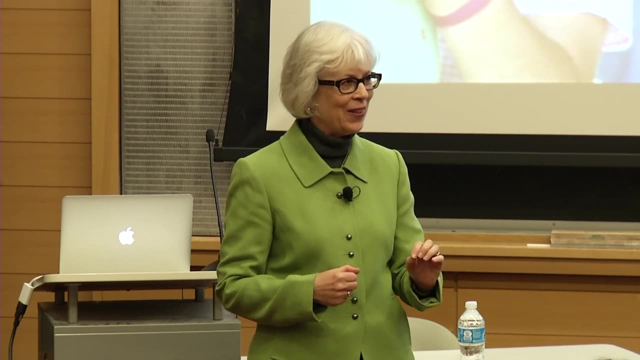 In fact, the reason why we collected the teeth to begin with was because Tom Boyce said: collect teeth so you can measure cortisol levels. But we never use the teeth to measure the cortisol levels. But we're very interested in doing that. Or the hair right. 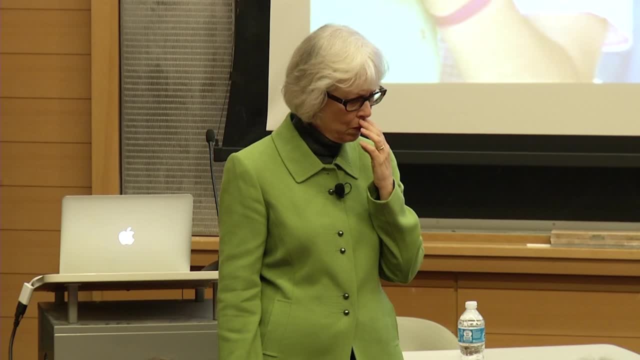 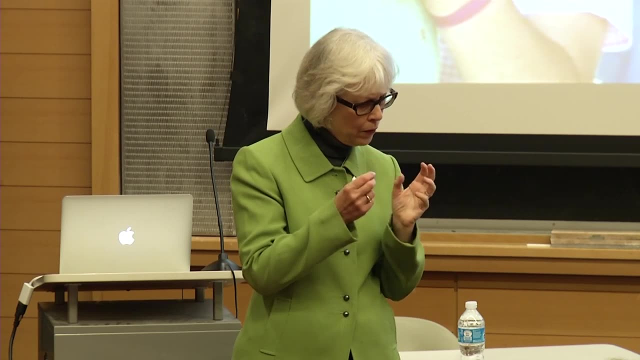 Or the hair. Yeah, we have hair now. Would hair be the best way to measure it? though That seems to be not a new hype, Because you can get time. You can get more of time, Right? I hope I remember this correctly. 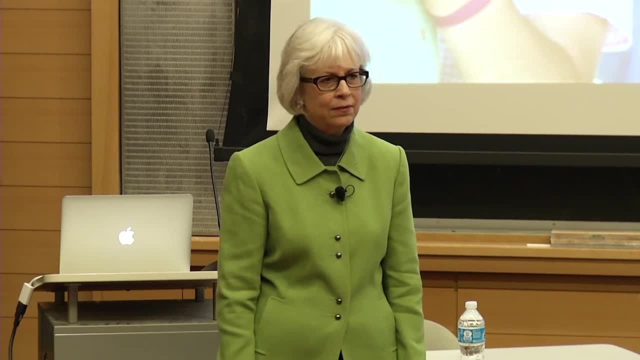 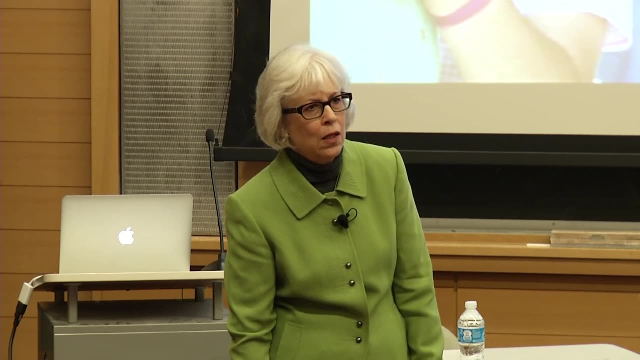 but I think you said that using the scale, you found differences at H2.. I was wondering if you could talk a little more about which specific aspects of development were impacted at H2? I can only tell you it was mental development. I can't tell you which parts of the 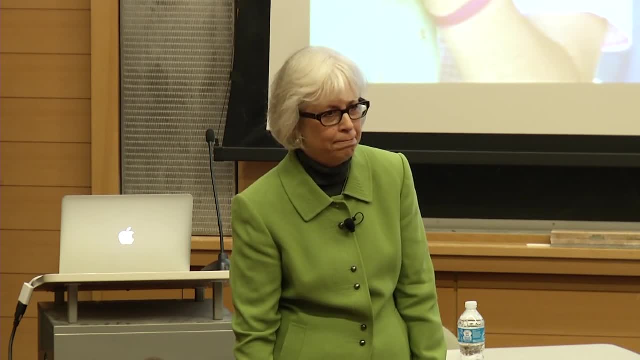 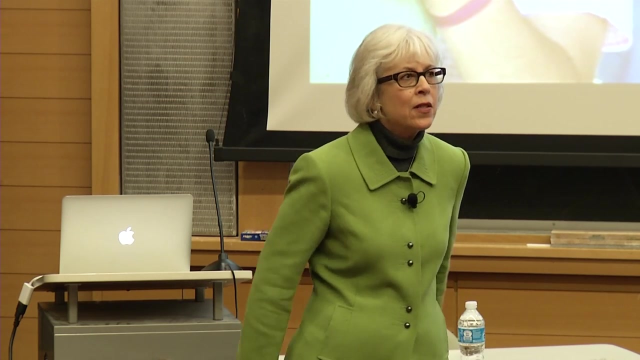 mental development scale. But I could look Any other questions. I have one: Can we scan the children? Scan them? Yeah, we've talked about it before. We'll talk offline. There is a beautiful study that was published out of one of our sister centers. 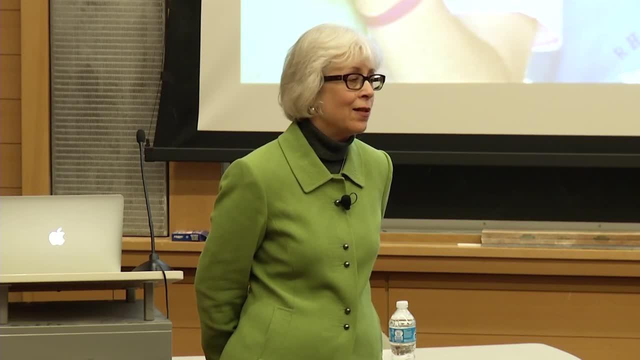 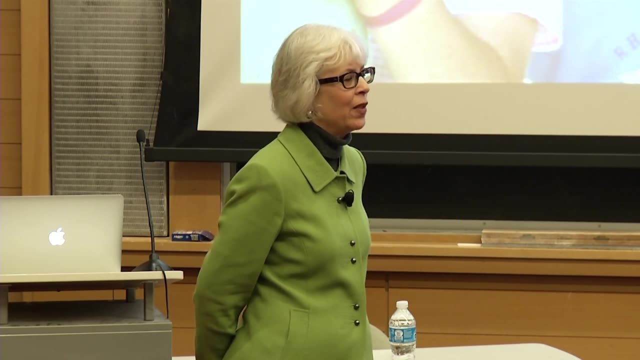 at Columbia University which did exactly that. The difference is that their children live within, I think, nine blocks of the hospital, Some very small diameter, around the hospital, And they scan the children and they found out that the chlorpyrifos levels, which is an 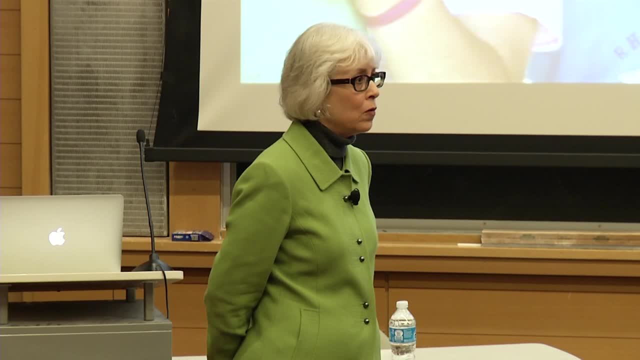 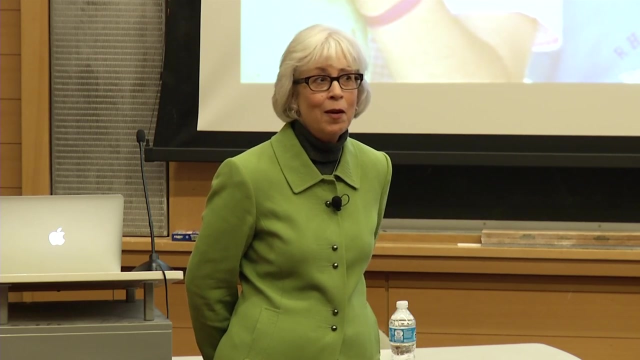 organophosphate pesticide that the children were exposed to in utero were related to changes on the MRI And that was published in PNAS recently. But our kids live too far away to get them here. That's one of the problems, But we'll consider it. 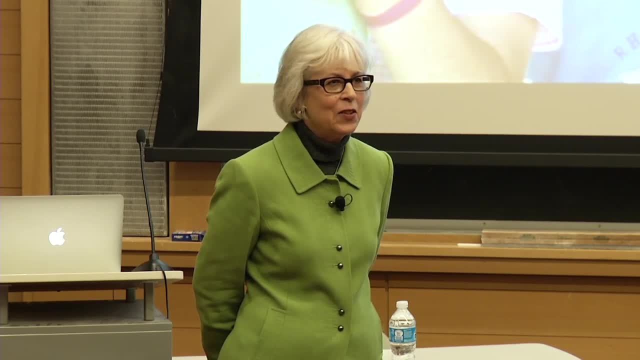 I have sort of a statistical question. Just looking visually at the charts, when you divided the subjects into quintiles, it seemed like the most severe detrimental effects were always for the upper, like the most exposed 20%, While the other 80%- I mean 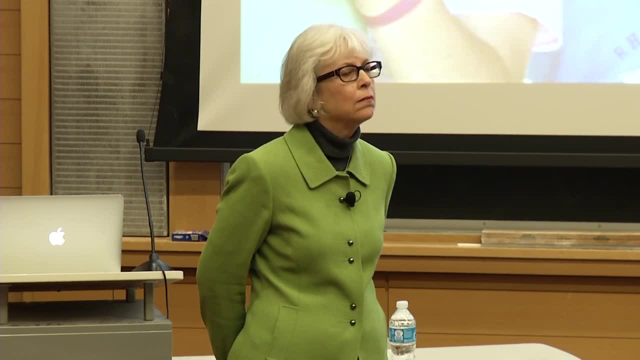 while still showing a tendency to have deficits, were less severe. So I was wondering if you had noticed any patterns for that particular upper 20%, or what the difference is between exposure levels for those upper 20% versus what the other 80% were. 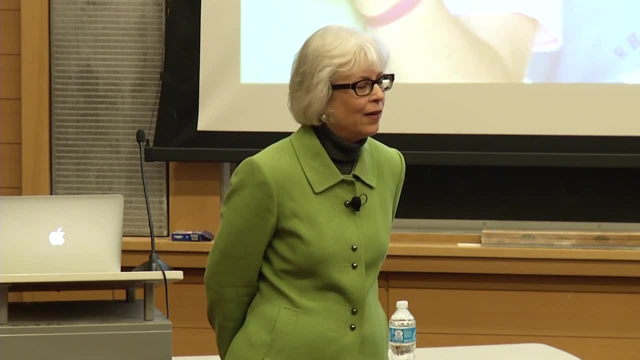 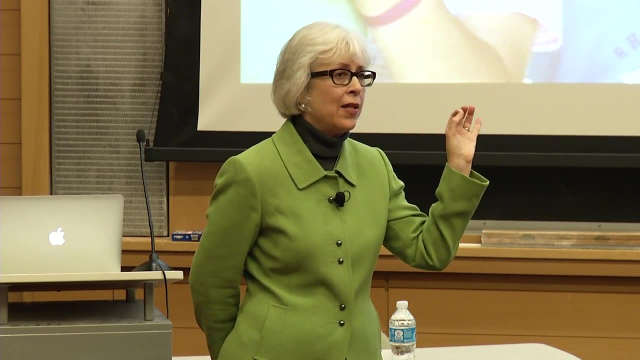 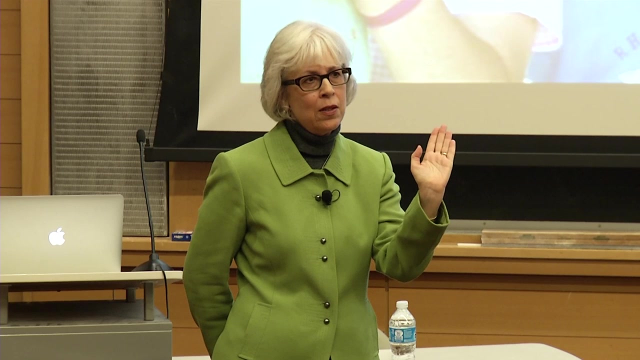 So I don't know exactly which one you're talking about, Because I did it a number of different times. But we always test for linearity And in a few of those cases I actually showed it that way for illustration purposes. But really, what we found in 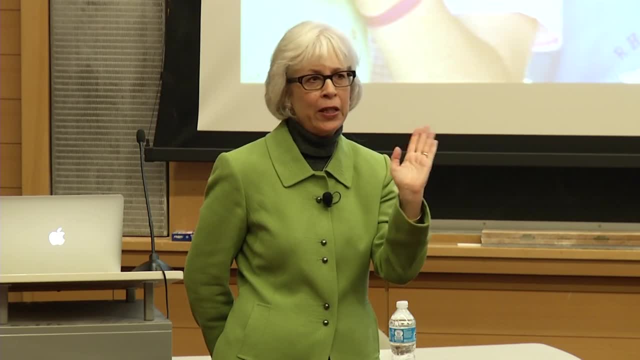 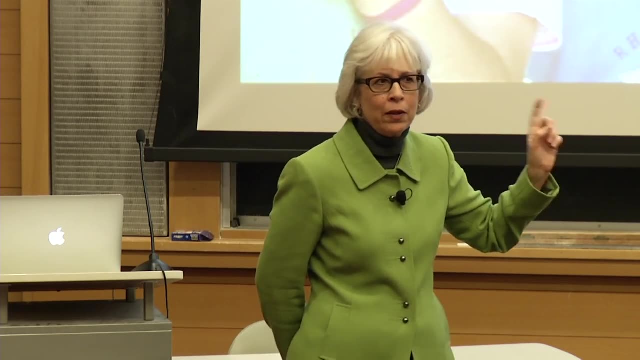 at least a couple of those slides- is that there was no deviation from linearity, So there was actually a gradual change as the exposure increased, But in one of those cases it was nonlinear, And I can't remember which one it was, In which case 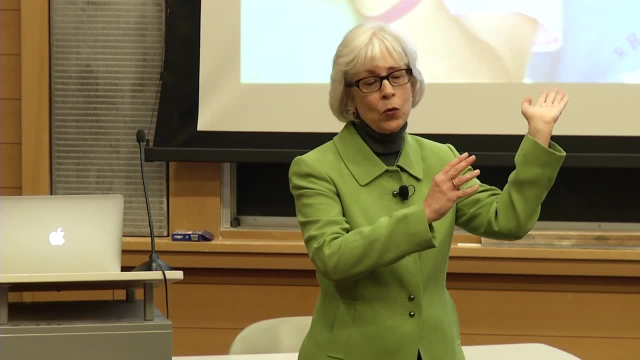 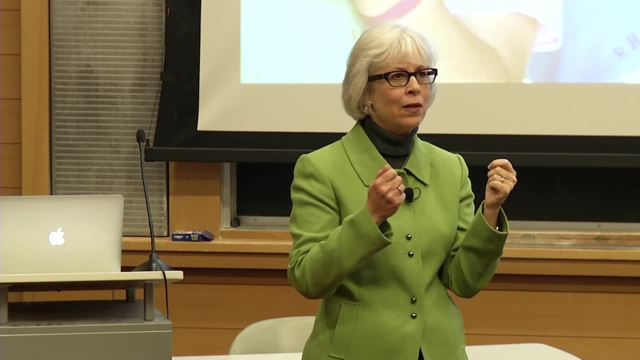 we then showed in the paper only by not quintiles, but in the paper we did it by quartiles because it wasn't linear. But in most cases we're seeing that the linear model does hold And there's no clear threshold. 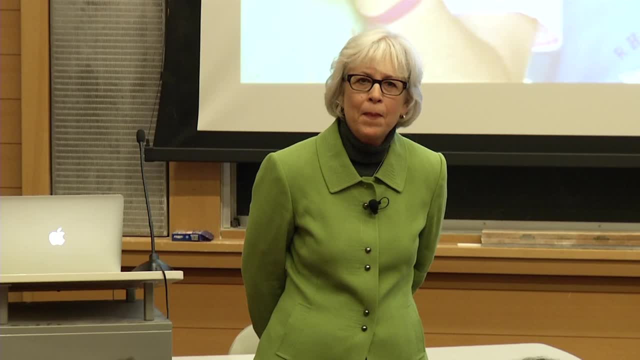 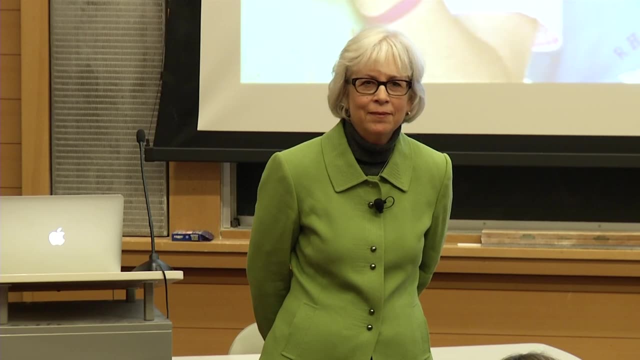 Hi Maya. So I'm curious, like maybe, like all, pretty much all of the findings that you presented are very convincing to me. So this is just kind of an idea that I'm floating, which is that what if the mothers who kind of were really protective of their children, 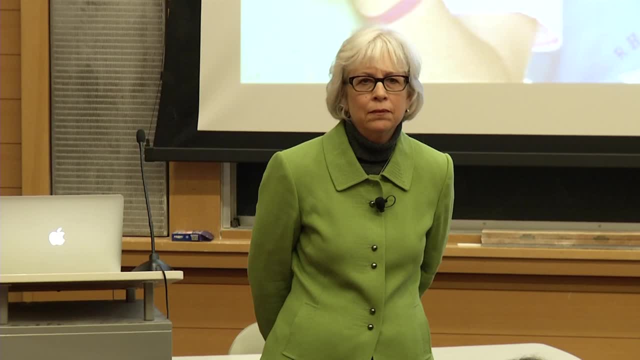 and really careful with what they were exposed to. those were the kids who, you know, had the least exposure, Whereas maybe the mothers- who- not trying to blame the mothers, but maybe they were more careless or they didn't know as much And maybe they were less educated. 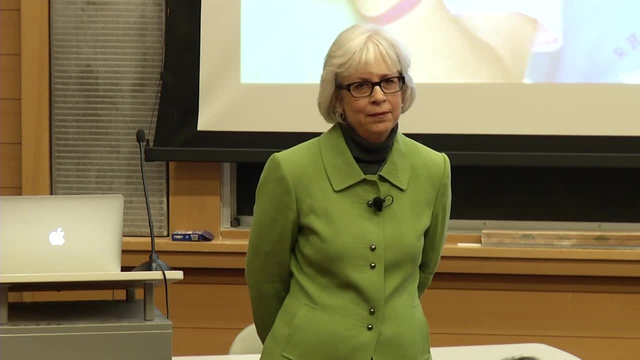 Although I know you have a relatively small band, But maybe it has something to do with the parenting style And I'm wondering how you think about that As a confound. Yes, That's a very good question. We keep thinking: okay, is there uncontrolled? 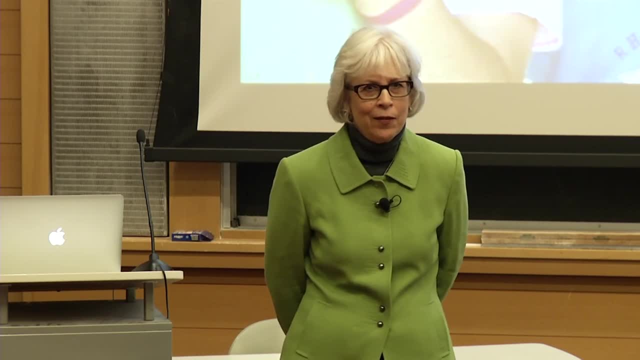 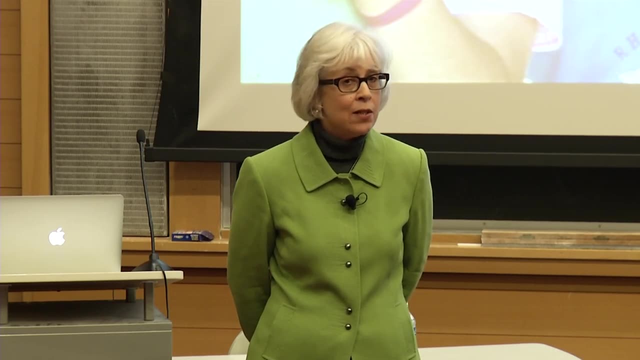 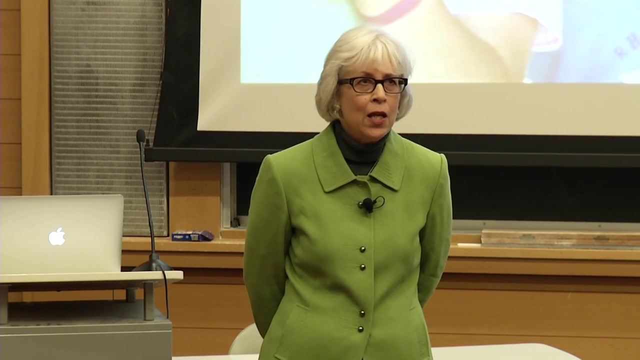 confounding And we have an extremely long questionnaire And also we did home assessments on the kids, Which doesn't mean that we've ruled out in any way, shape or form uncontrolled confounding, Because that's the problem of epidemiology. 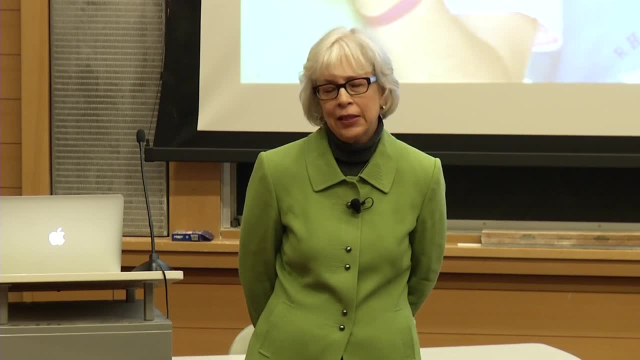 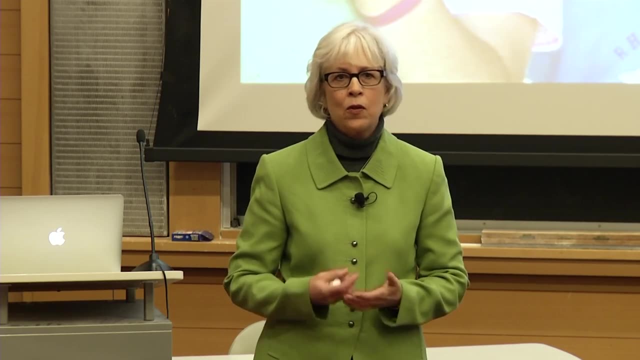 But we did do something called the home scale, Where we looked exactly at those kinds of things: Parent attachment, I mean those of you who are familiar with the home scale. you're looking at the interpersonal relationship of the child And we controlled for those. 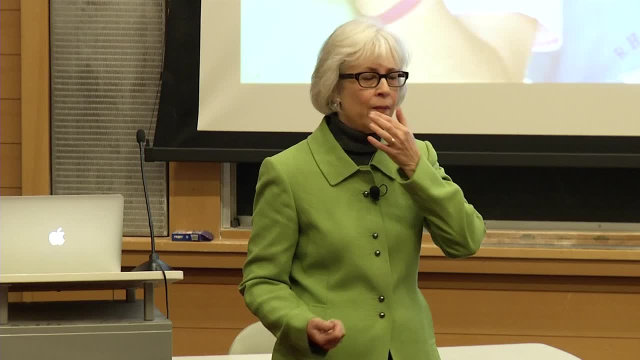 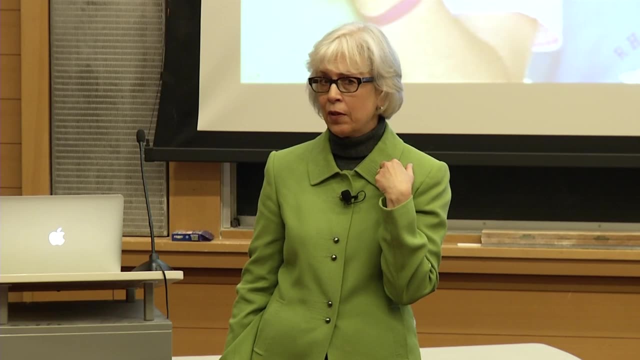 You've noticed, in some of the slides it said controlled for the home scale. That doesn't mean that there isn't something else that we didn't control, for Like, one of the things we were really concerned about was maternal depression, And so we did. 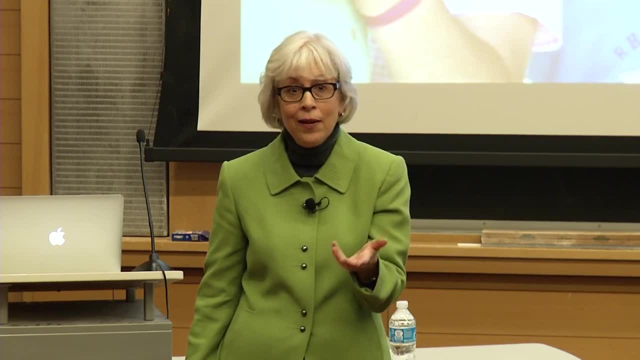 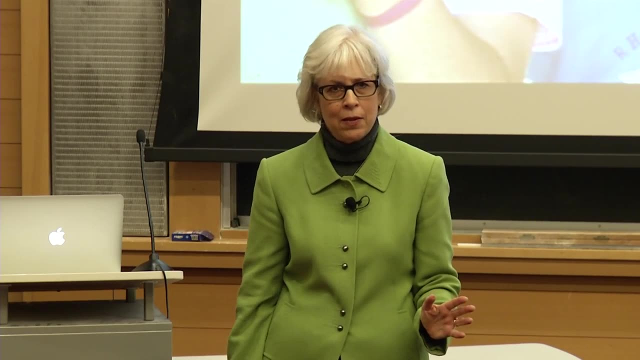 look specifically at that. So in other words, a mother that's depressed, is she more likely not to care about her kid getting into things and therefore may have higher exposure. So we controlled for that And it didn't seem to make a difference. 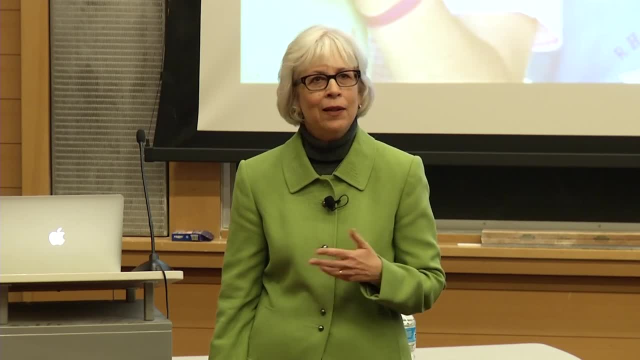 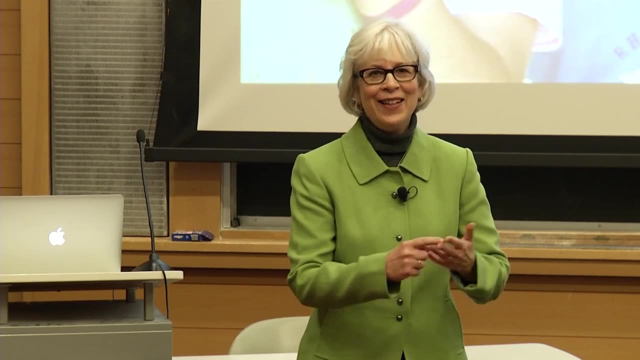 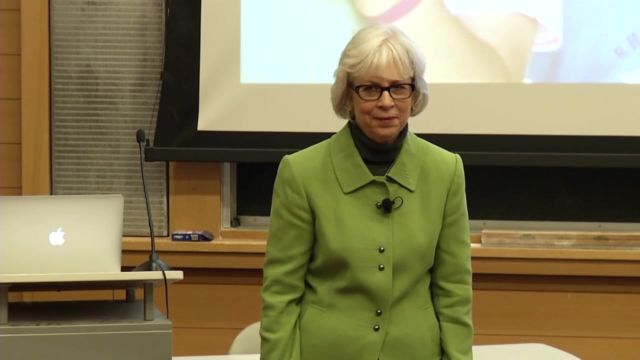 But there still could be other things And, believe me, we have scales on almost everything- Social support, depression, home environment- But we haven't looked at everything. I want to end. I want to thank all of you for coming here.